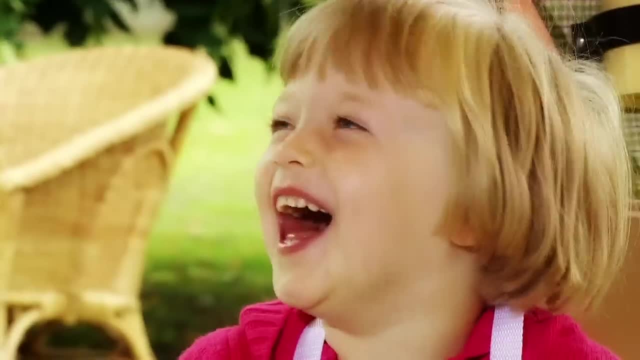 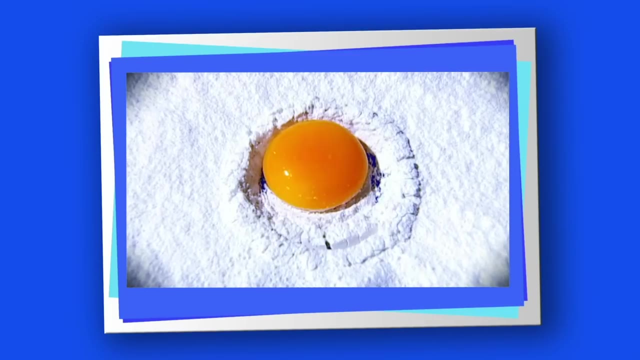 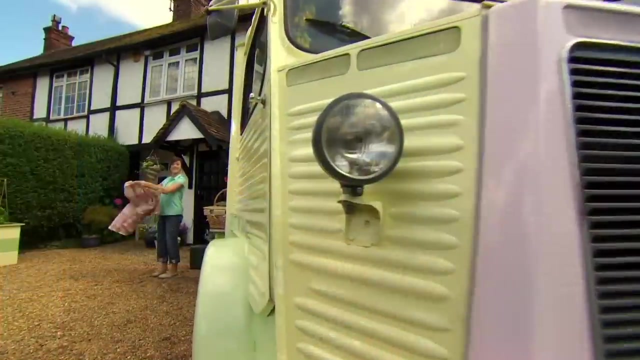 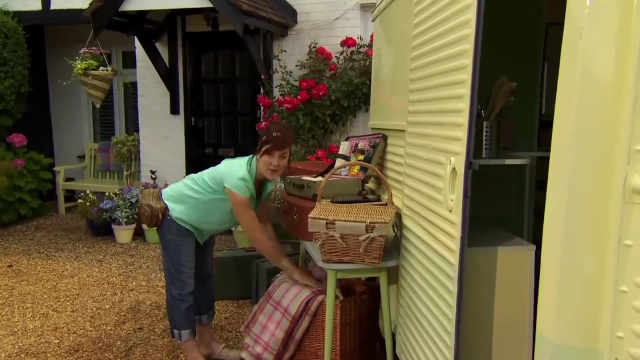 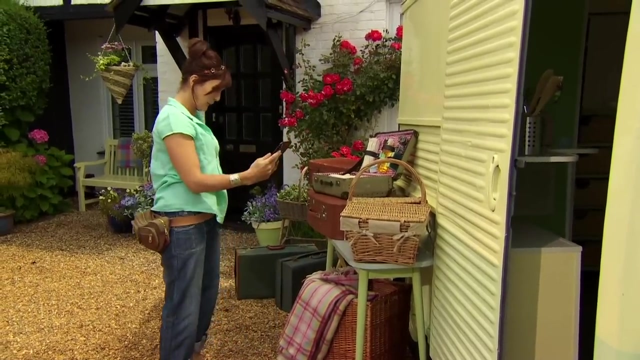 With you, Hello. Oh, great to see you. I'm just getting everything ready to go on a journey and I hope that you're going to come with me and make some new friends. Aha, Hello, Katie, Come have a picnic with me at the lighthouse. I love fruit. Wow, that would be brilliant. 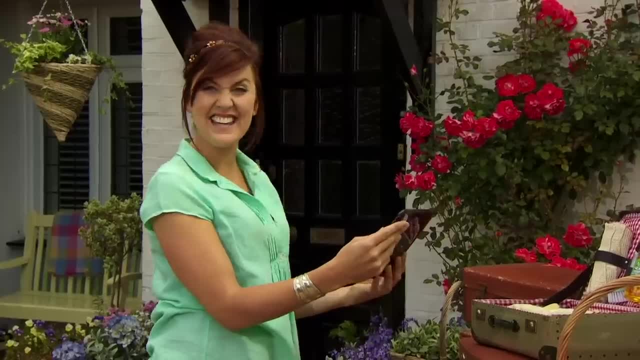 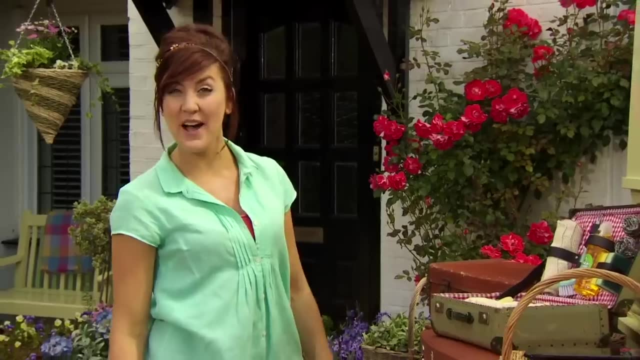 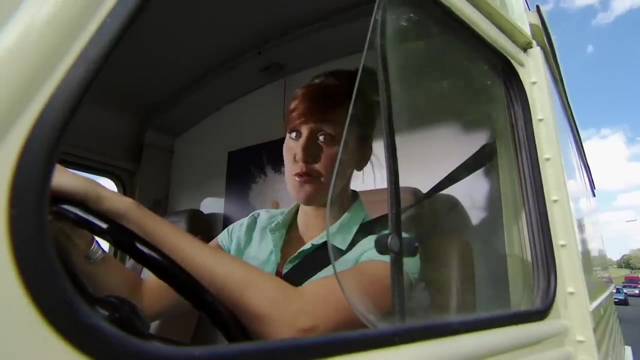 Katie, can you cook with me please? I can, and I love lighthouses, and you can cook with me too. So let's pack up and go. I'm on a journey and I'm coming to you. It's going to be busy and there's lots to do. Get ready to help, Join in and have fun. Let's cook. 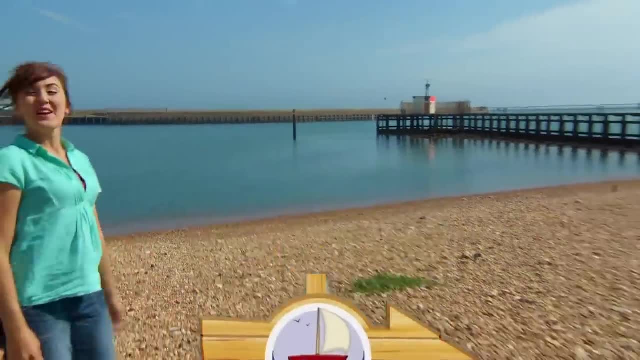 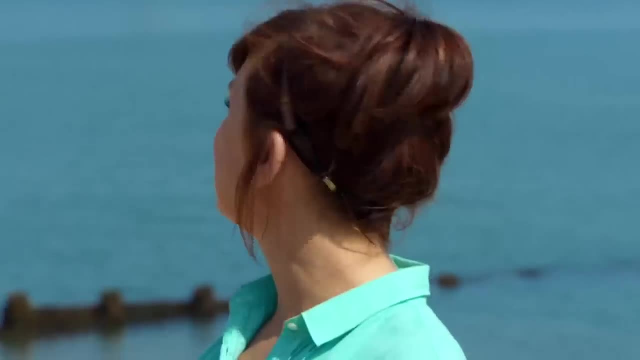 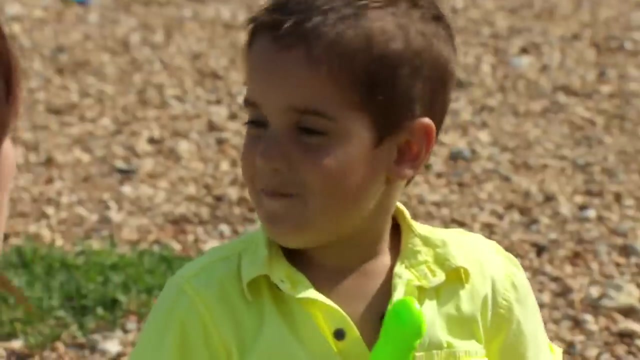 a feast for everyone. Well, here we are at the seaside, and hopefully I'm going to find Billy and a lighthouse around here somewhere. There he is. Hi, Billy, Hi, Katie Billy, are these all of your friends? Yes, So what's your name? Neely Jake Ivy. So Billy is. 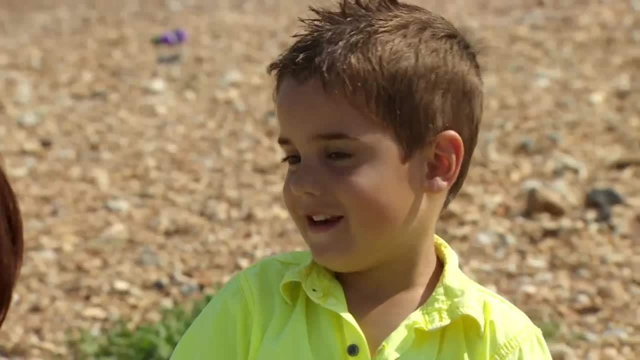 there really a lighthouse? Yes, So what's your name? Neely Jake Ivy. So, Billy, is there really a lighthouse around here somewhere? Yes, So we're going to have a picnic by it. Fantastic, I have got a delicious recipe to cook. Do you want to make it? Yes, Fantastic. 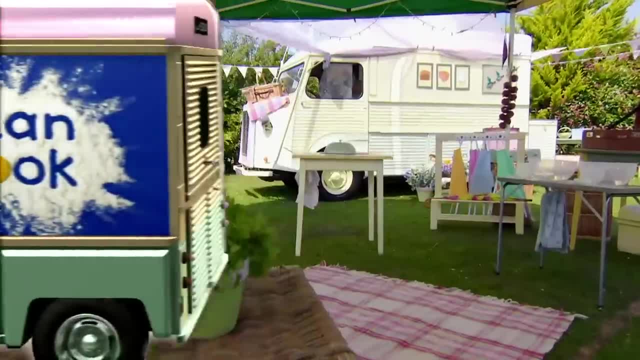 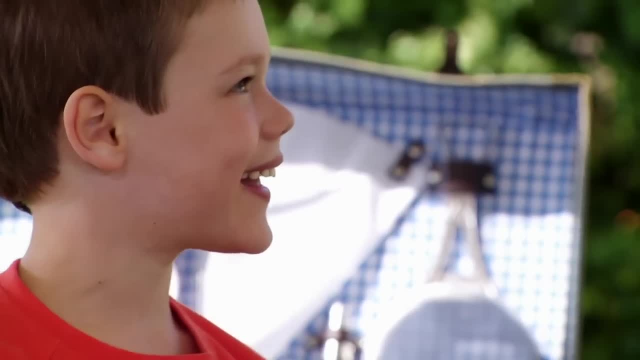 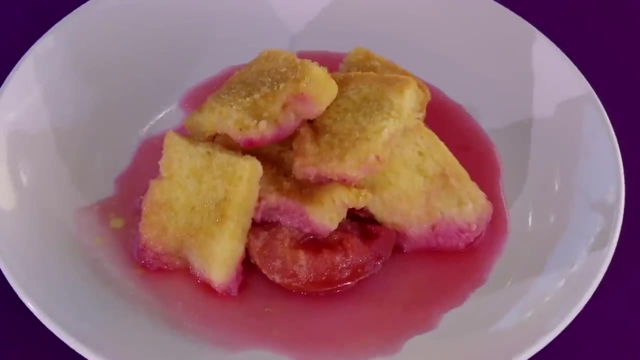 Follow me. Welcome to my outdoor kitchen, everyone. Do you want to know what we're going to cook today? Yes, Okay, I'll show you. Today's recipe is fruit jumble. Mmm, Mmm, Delicious huh. But before we get started on the cooking, we've got to do something. 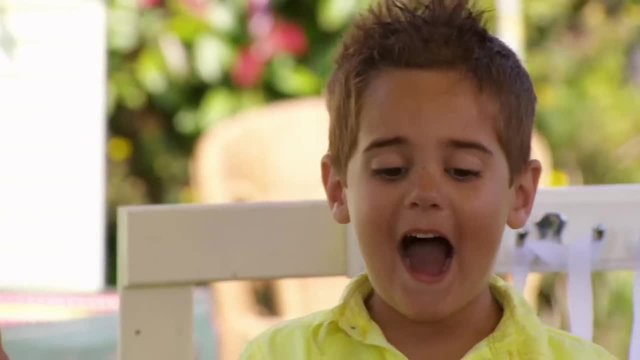 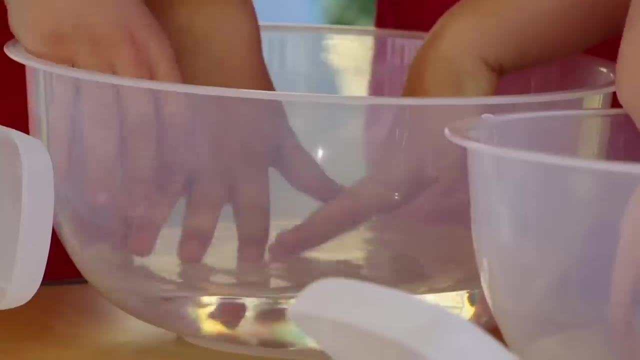 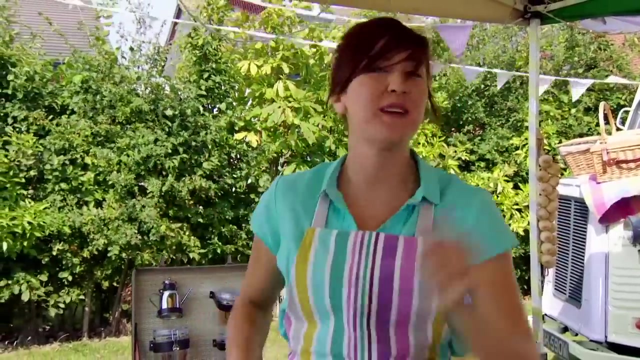 really, really important. Do you know what it is? Wash our hands. You've got it. We've got to wash our hands, of course. Come on, everyone, Let's get going. Roll up your sleeves, Give your hands a wash with slippy dippy soap, Splish, splash, splosh. Have you done your? 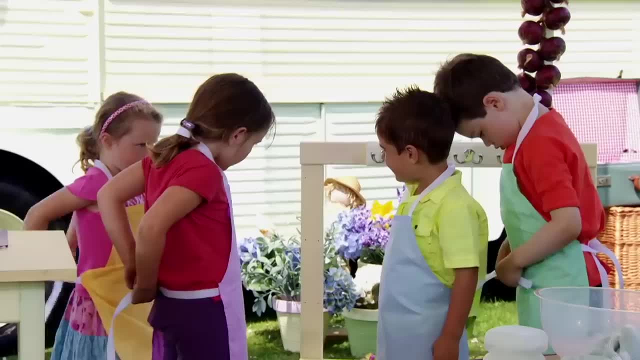 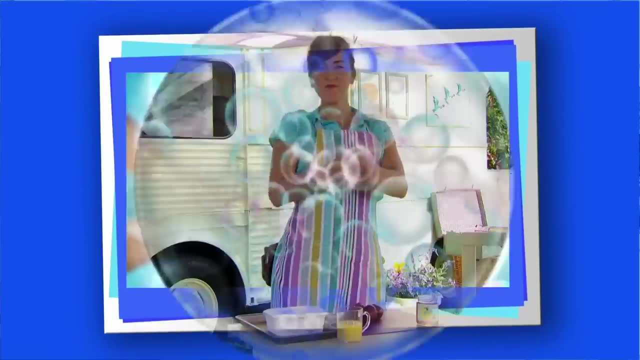 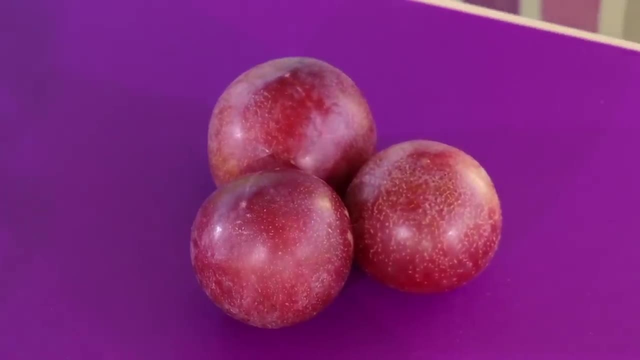 hands Washed and dried, Sleeves rolled up, Apron tied. What can you do? I can cook. Right. then let's get started on our fruit jumble. The first ingredient we need is some plums. Now. plums can come in all sorts of different shapes. 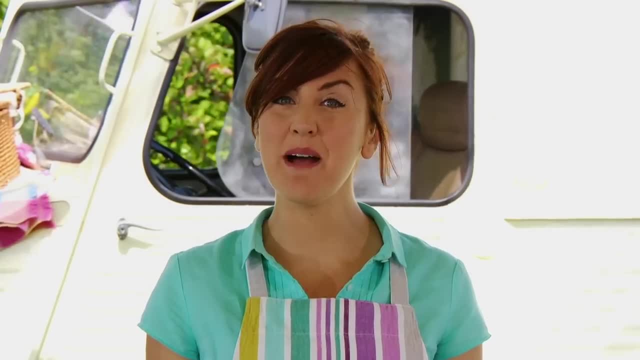 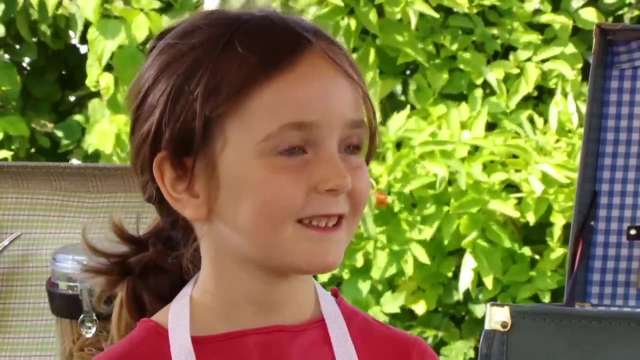 and sizes, but the ones we've got here are small, around like little bouncy balls. And what colour are they? Ivy Red, Lovely red colour. I wonder what colour they are inside. Shall we find out? Yeah, Yeah, And to do that we're going to use a table knife. Now, some 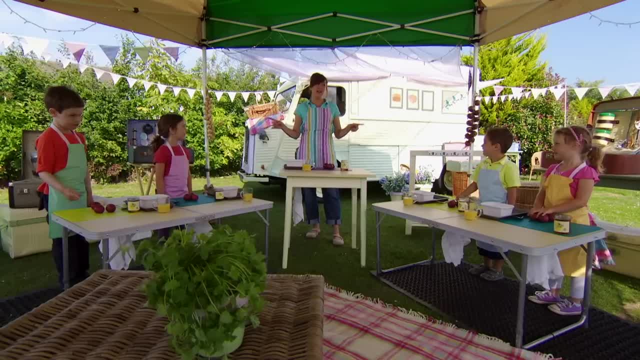 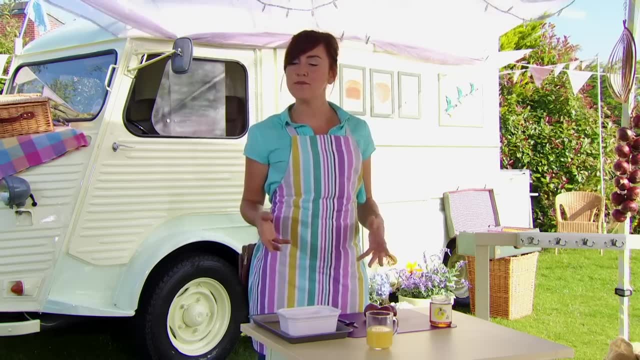 knives can be sharp, can't they? Yeah, So we're going to use a table knife And we're going to use a table knife, So you do have to be very careful, But a table knife is the kind of knife that you're used to using when you're at home, so it's fine to use. So we're. 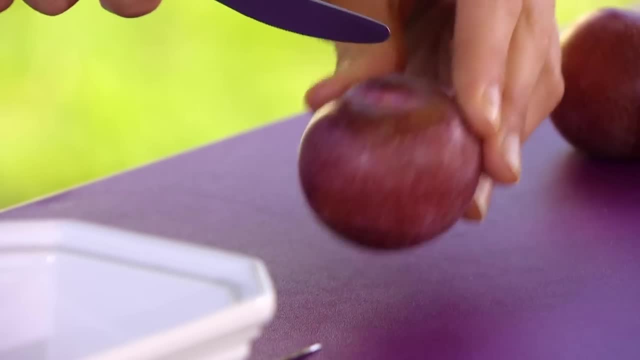 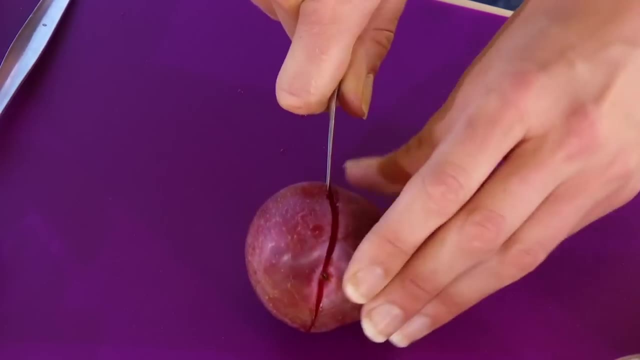 going to move these two to the side and we're going to hold the plum like this and we're going to put the knife into it until we hit the stone And then we're going to walk the knife around the plum. There we go Round there like that. There we go, Like going. 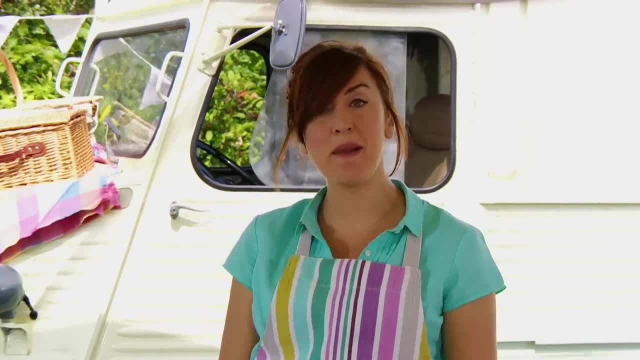 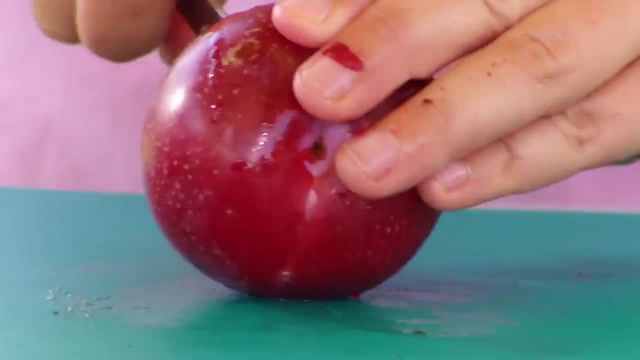 round the world. Yeah, we're going to cut round the world. Yeah, we're going to cut round it like it's a plum planet. So keep your plums on the mat, Cut through until you can feel the stone. Yeah, I've hit the stone. Take it all the way round. You should have. 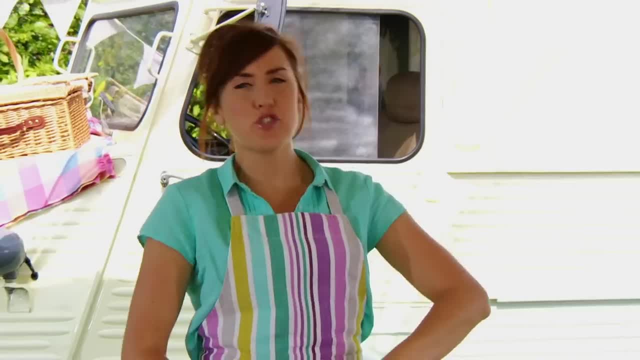 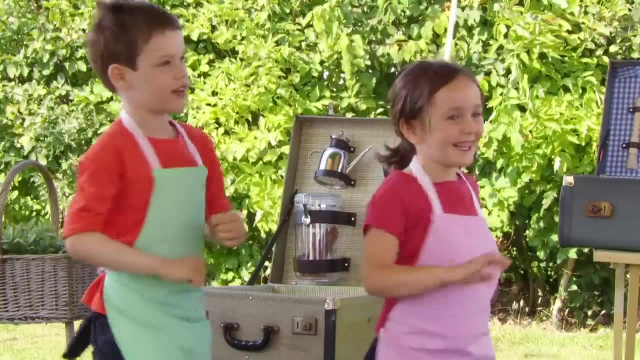 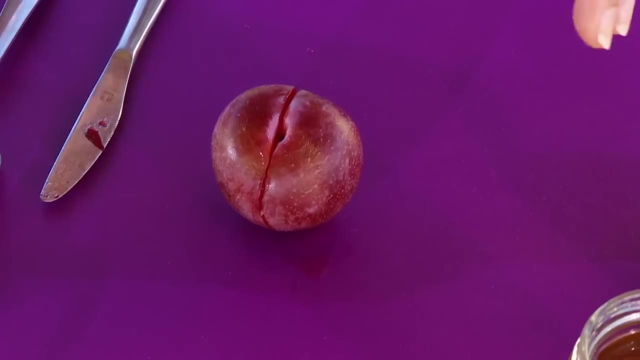 a line all the way round your plum. So next we're going to twist the plum, But we do the twist like this: We do the twist, We do the twist, Do the twist, We do the twist. Fantastic, Now we're going to do the twist with the plum. So to do that, we need to hold the 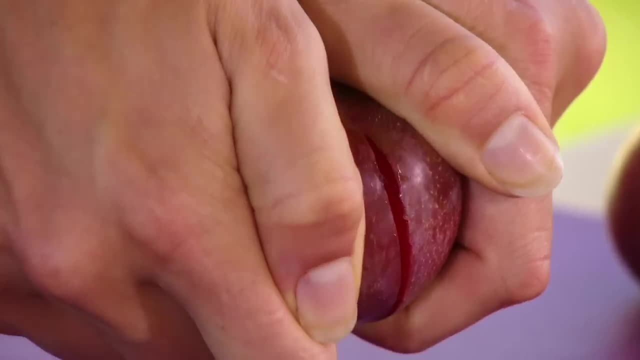 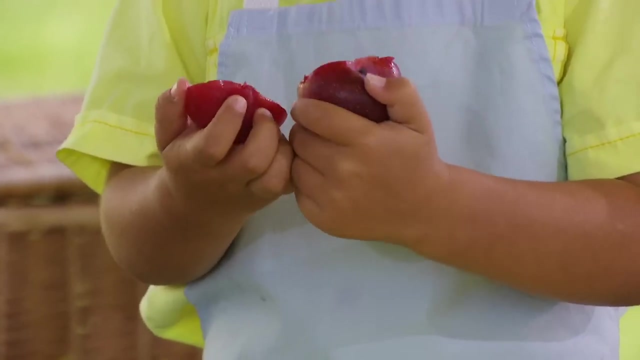 plum And we twist it like this. You can do it, You can do it, Keep going. You're nearly there, Yeah, Yay, OK. Next we need to cut both of these halves into two more pieces, So we put them down. 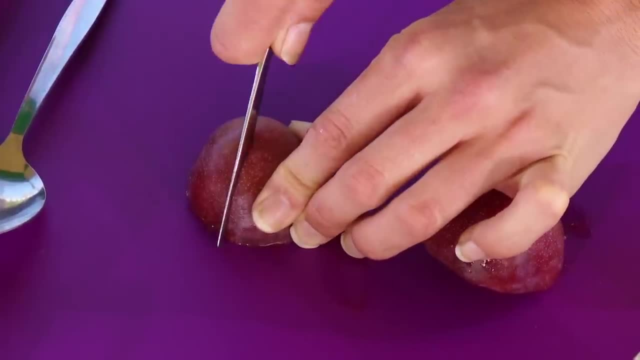 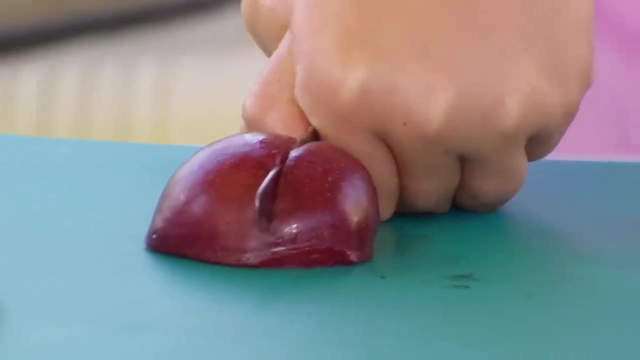 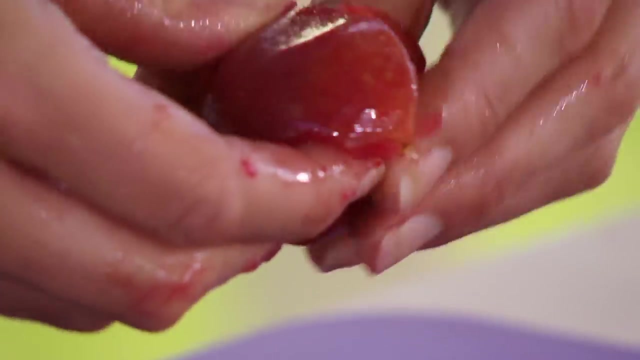 there like that. and then we cut the plum down the middle like that, until they look like two little ladybird wings. Then we're going to cut the other one as well and cut around the stone, And then we twist it apart like this. There we go, And now we need to dig our fingers. 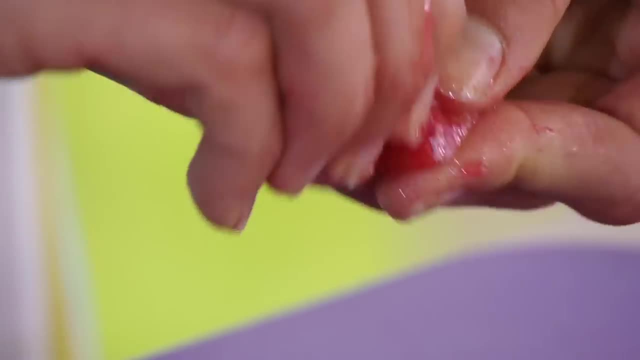 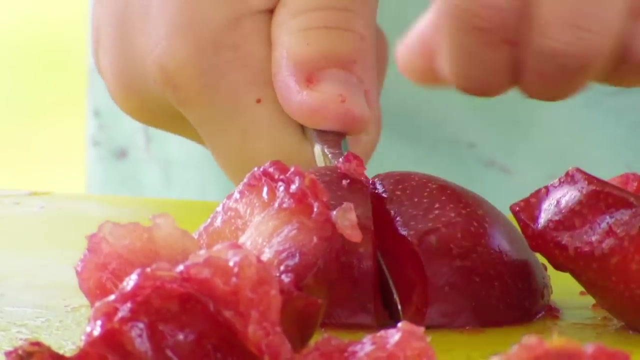 underneath this stone here and twist it out There. it is Alright, let's carry on with the other two plums. Oh, look at these plums. They're so red inside. Now we need to take these plums and put them into our dish. 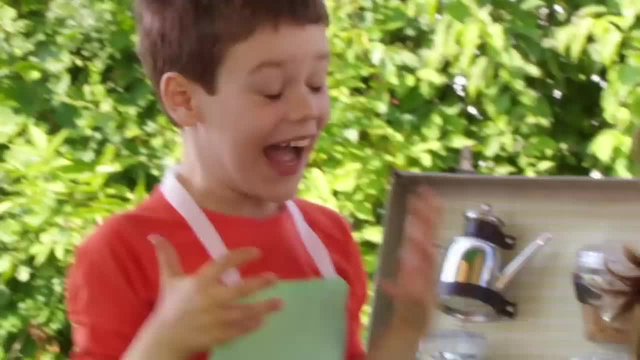 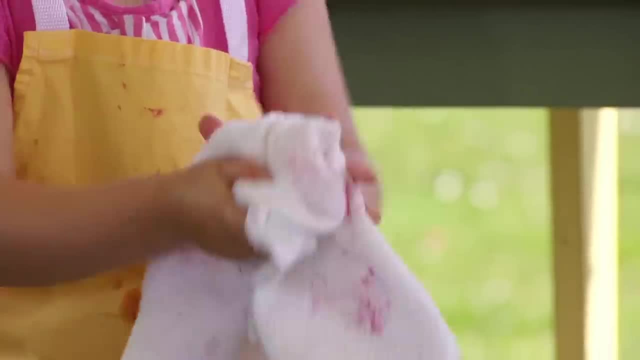 I got a little one. I look like I've got monster hands. Jaaah, Yay, Me too. I'm the winner. Shall we give our hands a wipe. OK, ready for the next part? Yeah, The next step is to add some orange juice to our plums. 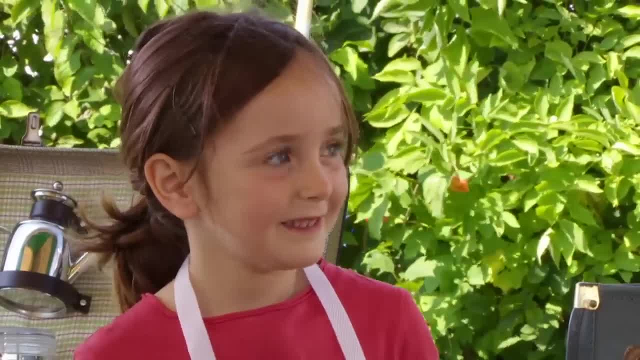 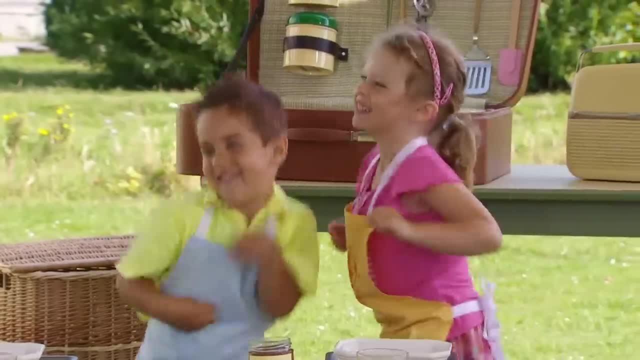 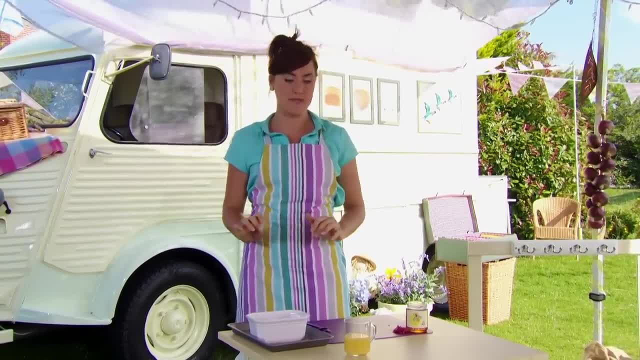 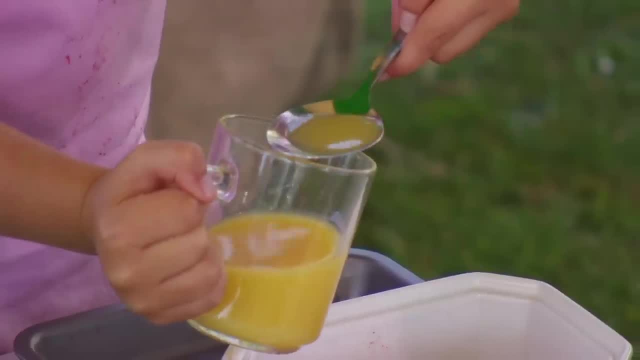 I think it's about time that we added some fruity juice to our fruity plums. OK, we need to measure out one tablespoon of orange juice, So we put the spoon into the cup and we tip and load to fill it up And we put one in there, like that. 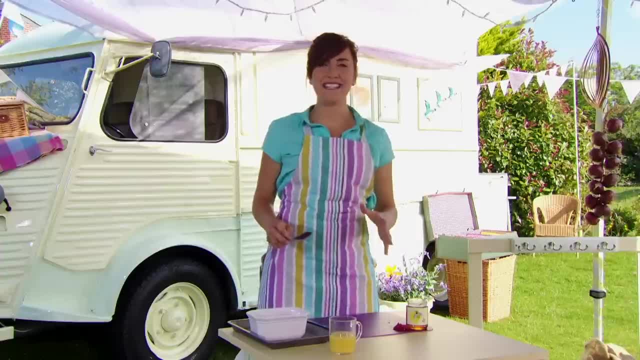 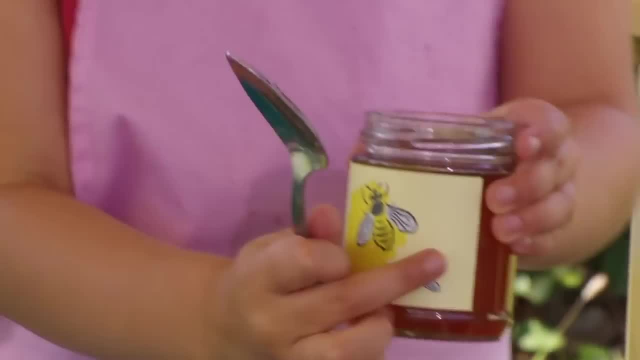 And that's all the orange juice you need. Next, we're going to add a tablespoonful of yummy runny honey. Oh, I love honey. Bring the jar over to the dish and drizzle it all around. Oh, over the plums. 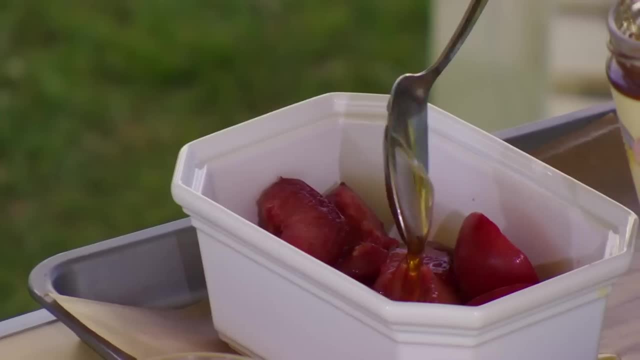 Oh, look at that, Everyone go drizzle, drizzle, drizzle, Drizzle, drizzle, drizzle. OK, and then, when you've done that, we want to mix the plums with the honey and the orange juice. 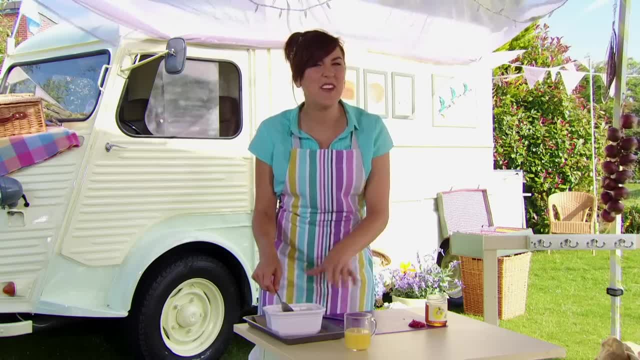 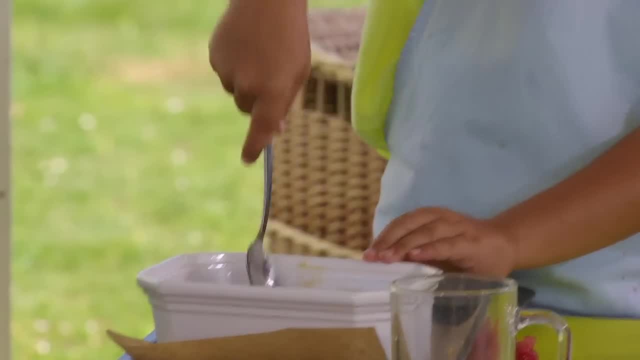 Mix, mix, mix. And you can mix with us as well. You can get your dish and your spoon and go mix, mix, mix. Now that's the fruity part of our recipe done. Now I wonder what ingredient we're going to need next in this recipe. 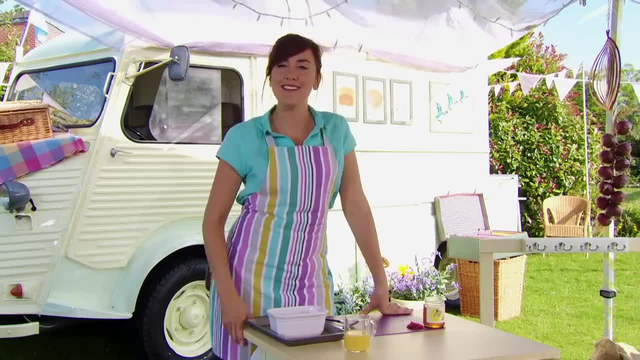 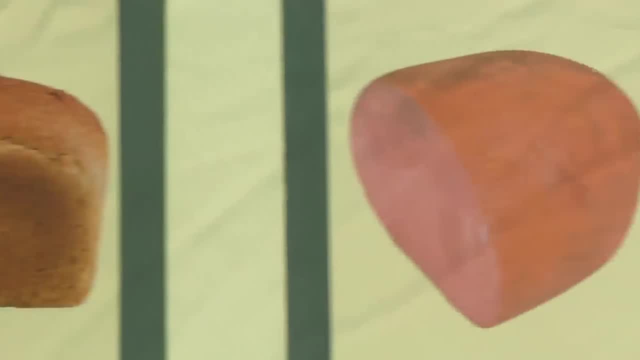 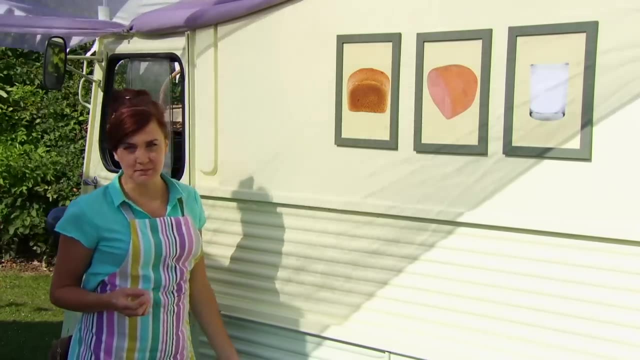 What's next? Well, let us see if you can guess what it could be. So we've got some bread, some ham and a glass of milk. What would you use for our fruit jumble? I know I'll give you some clues and you can try and guess what it might be. 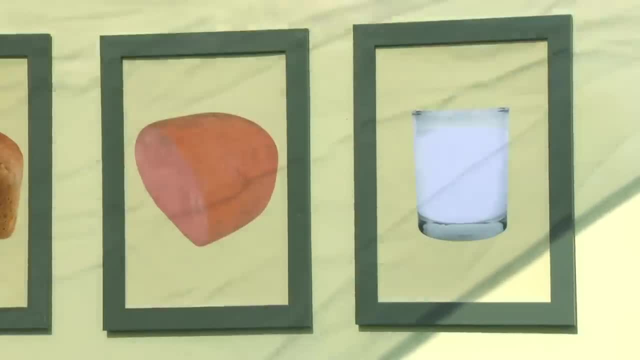 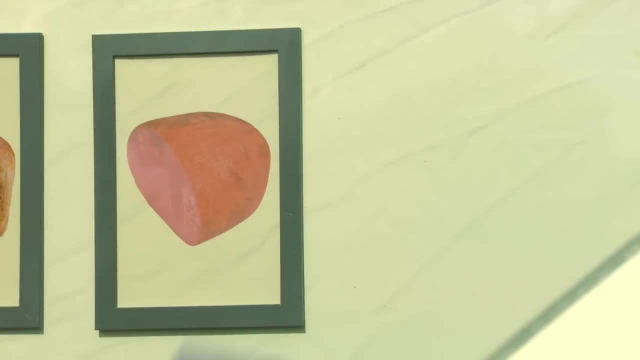 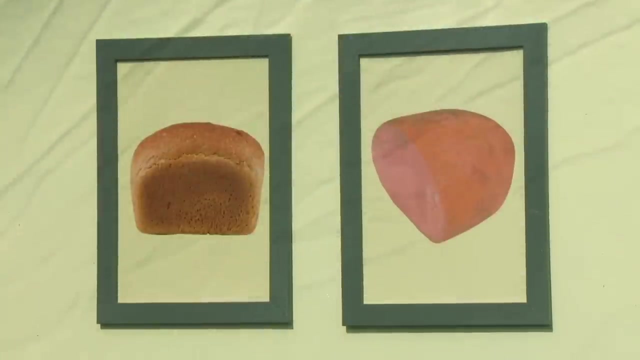 The special ingredient is something that you can slice. You can't slice a glass of milk, can you? So we can take that one away. There we go. OK, here's another clue for you. The special ingredient is something we can slice, but also it's something that you can make into toast. 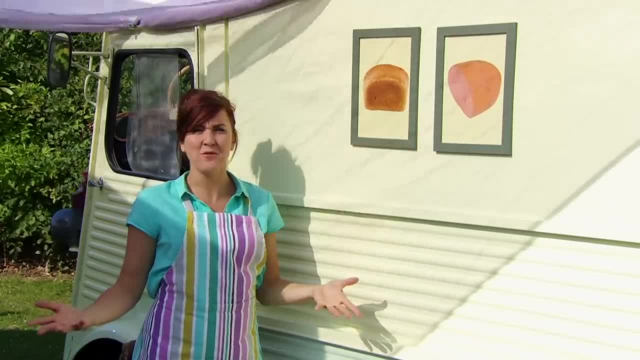 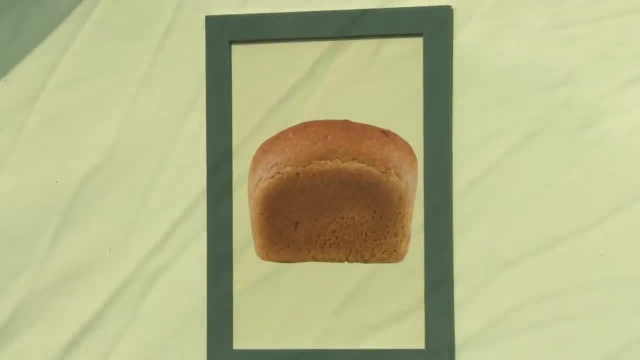 Well, you can slice ham, but you can't make ham into toast, can you Never done that before? So let's take that one away as well, Which leaves us with bread. We're going to need some lovely bread for our fruit jumble. 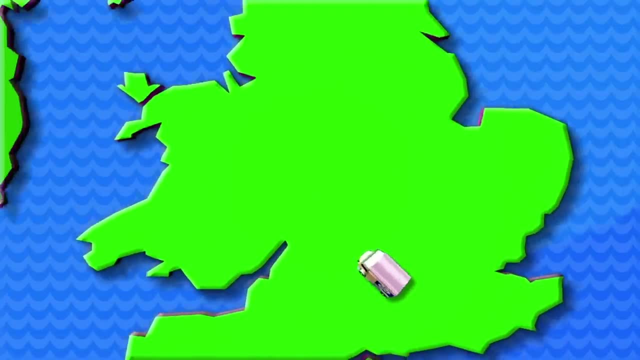 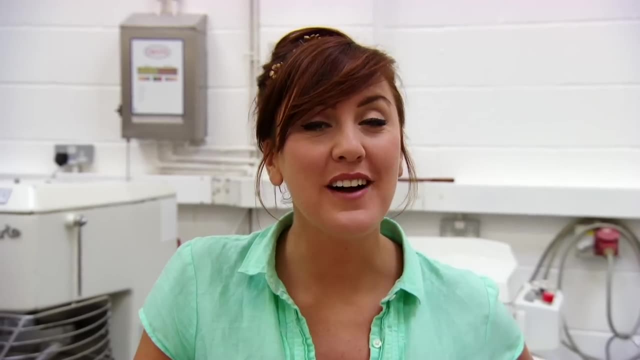 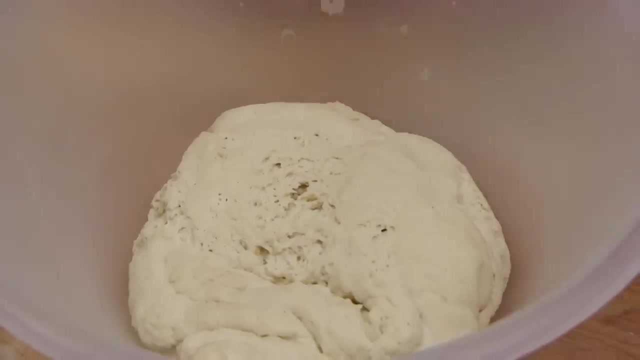 And I went to find some. I've come to Newcastle to meet my friend, Ian the baker, who's going to tell me how bread is made. We've got flour, sourdough, yeast, salt and water and we mix them together. 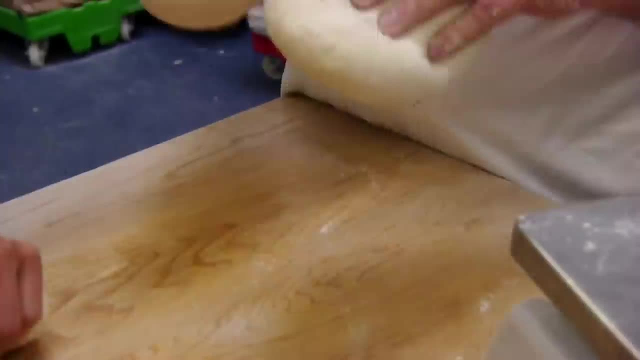 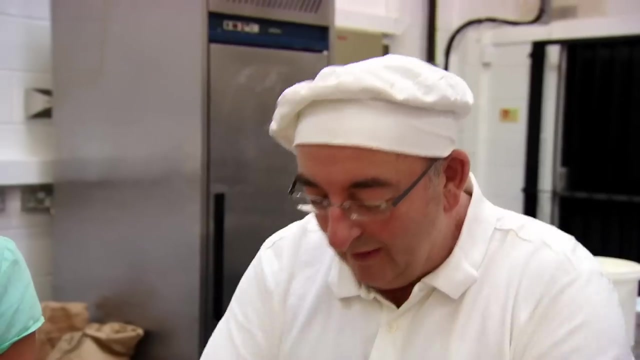 Once it's been really well mixed, Ian needs it to spread the yeast and make it all stick together, And when you've got the dough really tight, you elongate it. roll it out like that, OK, and then we put it into the bread tins. 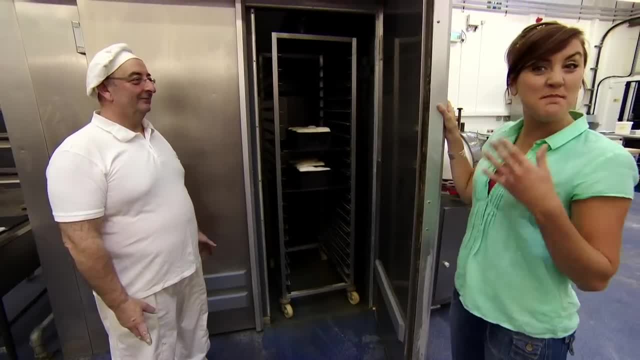 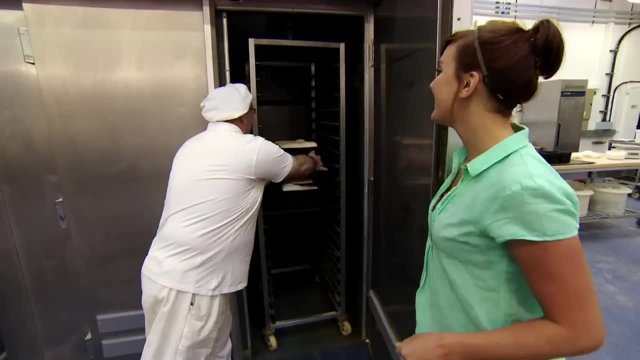 Our dough has been put into this big warm room called the prover and the yeast has made the dough rise up. Then it just goes in the oven to bake for about 45 minutes. So what do we do with the bread now that it's cooled down, Ian? 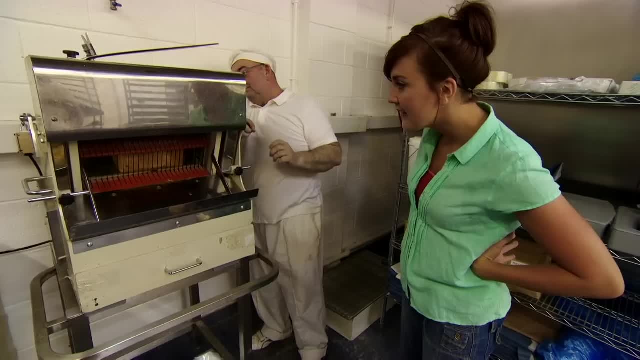 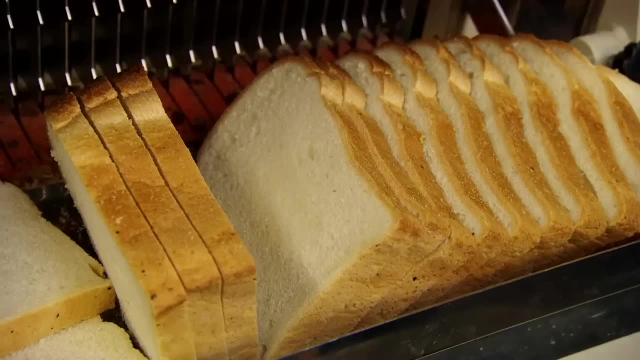 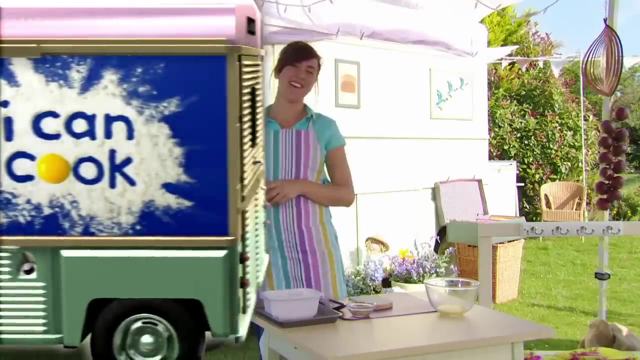 What we've got to do is slice it. Oh wow, this bread is going to be perfect for our fruit jumble. Thanks very much, Ian Pleasure. I love the smell of freshly baked bread. So we've got one slice of bread here, and what we're going to do is cut it. 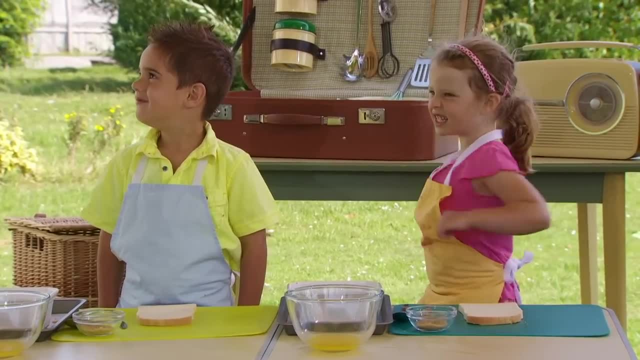 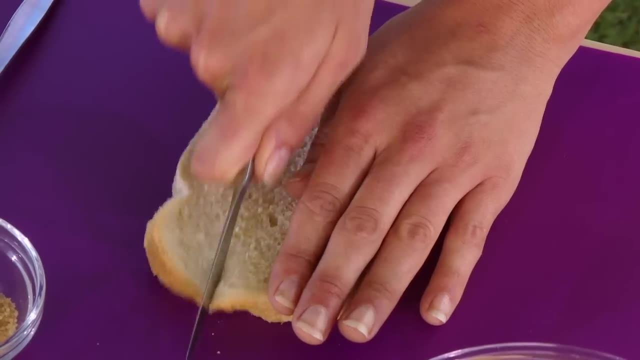 So is everyone ready to do some more cutting? Yes, OK. so put your hand on one side of the bread and use the table knife to cut a line down this side, like that. And if you can't cut through the crust, that's OK, because you can just tear them with your finger. 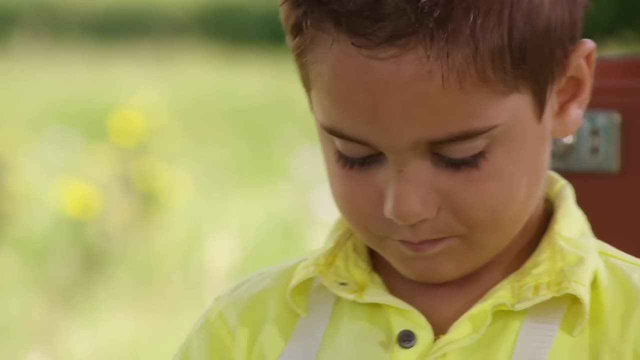 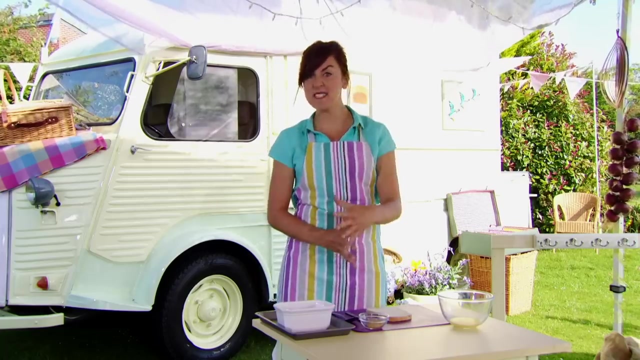 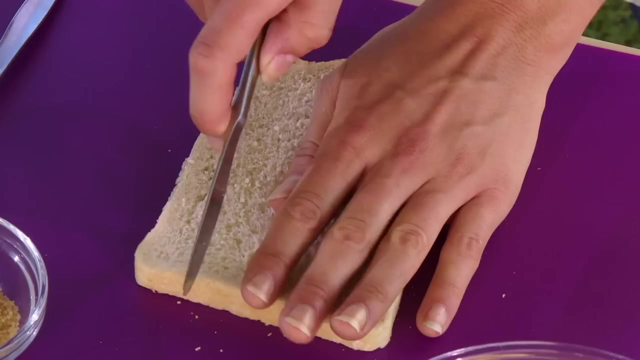 That's it, and put the piece of bread back together like it's one piece, And then we're going to turn the whole slice of bread upside down like this: Look at that. And then we're going to cut it again. So put your hand there and then cut, cut, cut. 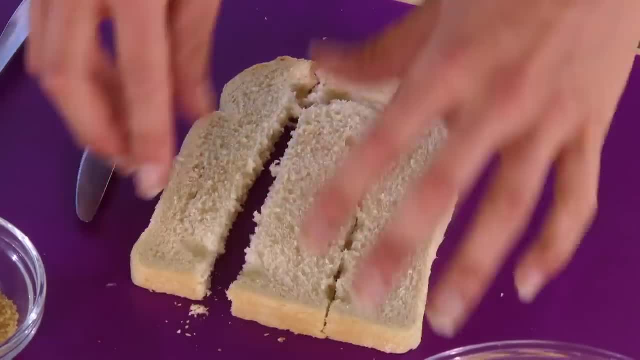 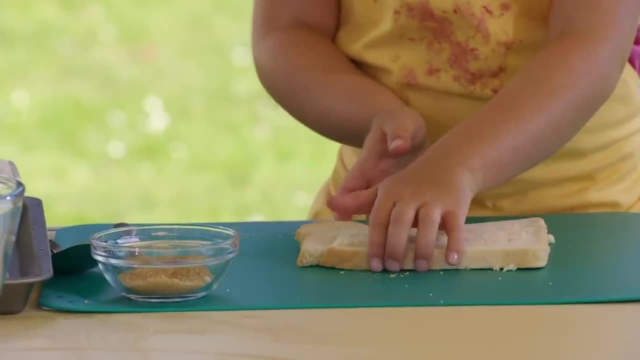 And if you don't cut all the way through the crust, we just give it a little rip And now we need to do two slices the other way. So we turn the bread around like that And then we cut And then cut down that side. 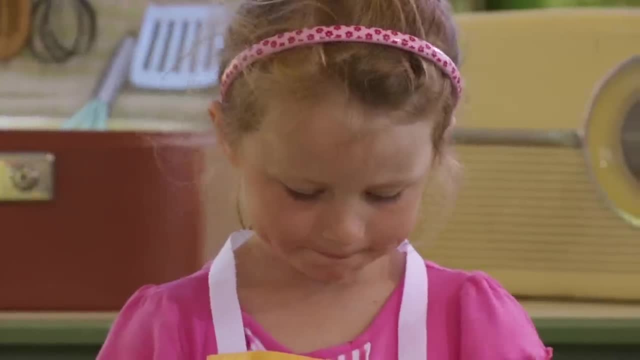 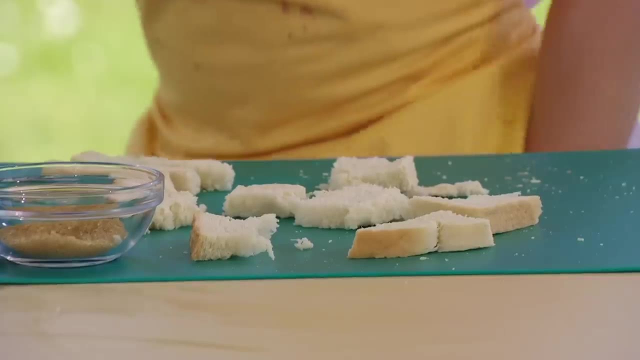 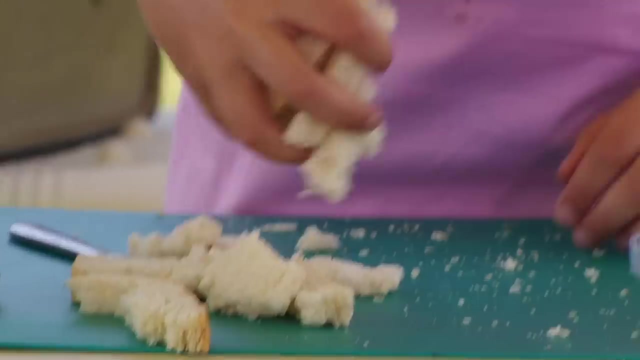 And then move your hand over a little bit further and cut down a bit more, And it doesn't matter if they're not perfect, OK, All right, are we all ready for the next part? Yeah, OK, now we are going to put all of our bread pieces into this butter that I've already melted for you. 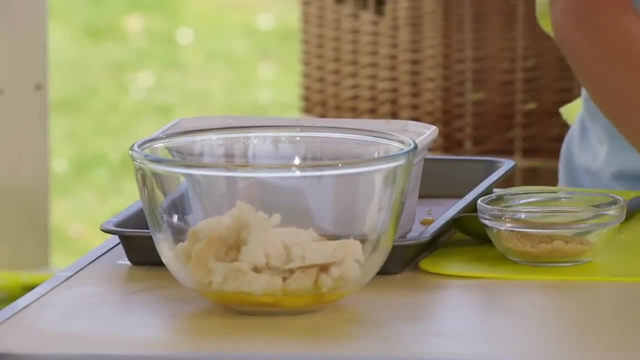 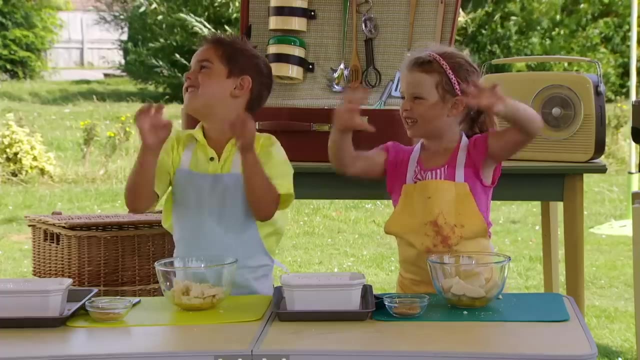 I've got a lot And then bring your bowl over to you on your mat. Yeah, Now we're going to get really messy. Let's get messy, Brilliant, Everyone. put your hands into the melted butter with the bread and get them all buttery. 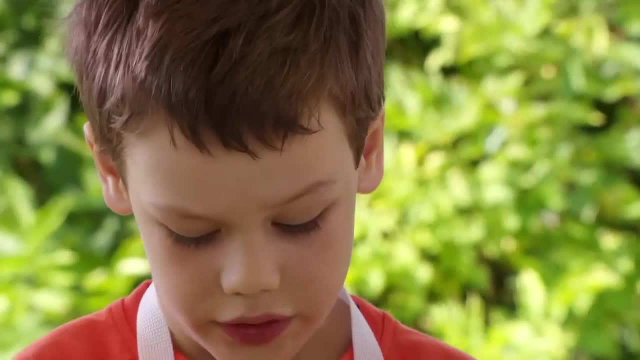 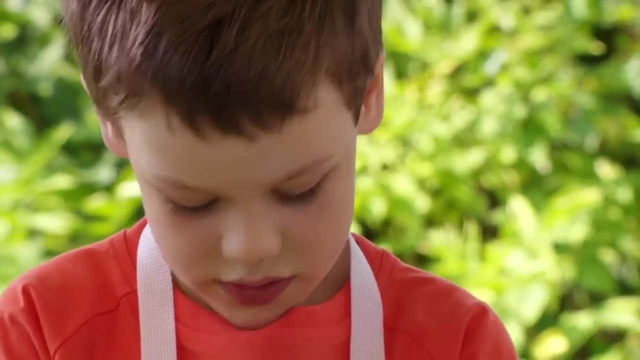 Jake, what's the bread doing to the butter? It's getting thick, Tom, It's sucking it all up like a sponge, isn't it? Oh cool, It's going like this. Everyone who can do a big slurp. 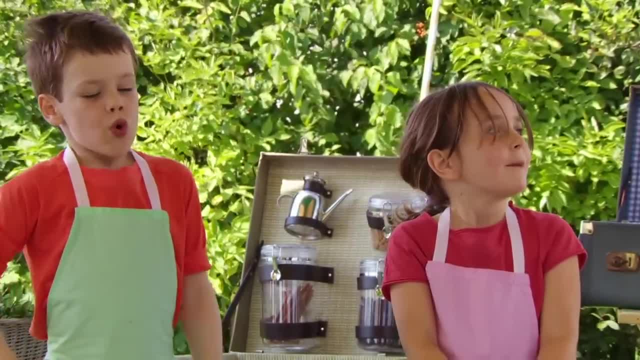 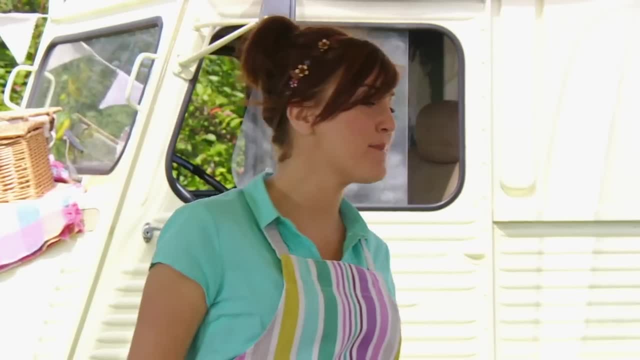 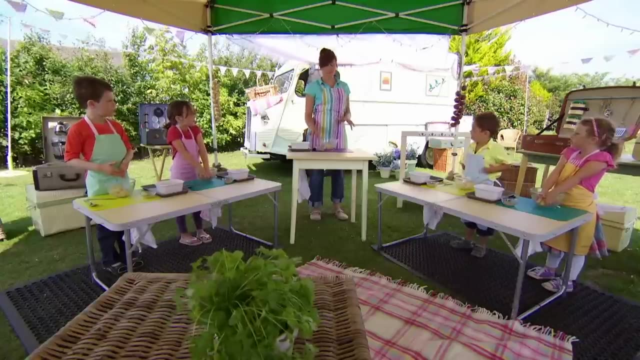 Ready? Oh, can I do it? Yeah, you can Do that again. Yeah. So, Neelie, what colour has the bread gone? Yellow, That's right It has. The next thing we're going to do is take some of this lovely sugar. 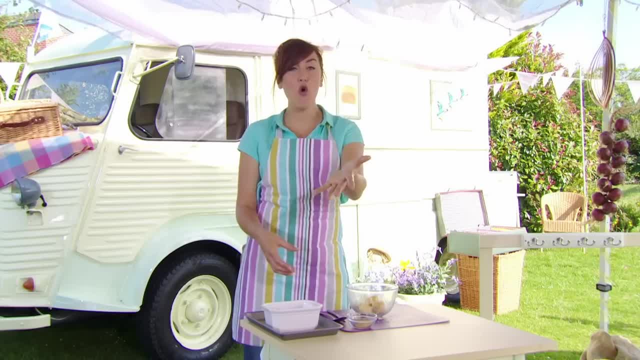 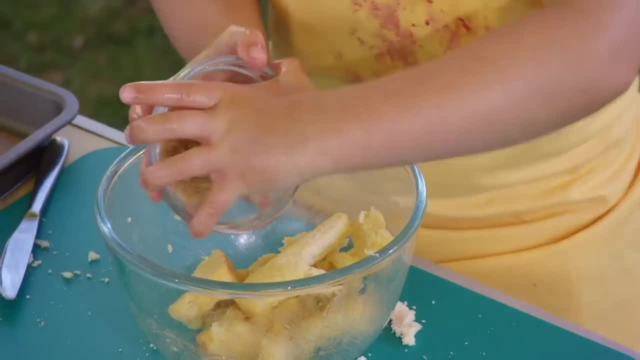 But it's not the normal kind of sugar that you might be used to. It's called demerara sugar And we're going to use some but not all, So make sure that you leave a little bit of sugar in your bowls for later on. 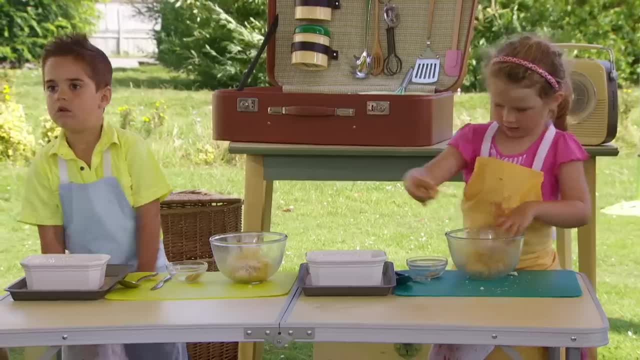 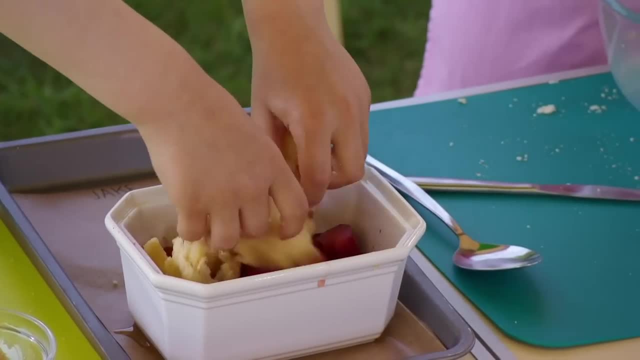 And now we need to put all of this lovely bread on top of our plate, Of our plums. Oh, look at that, It's like burying treasure. Yeah, you are. Last of all, we're going to take the rest of the demerara sugar and sprinkle it on top. 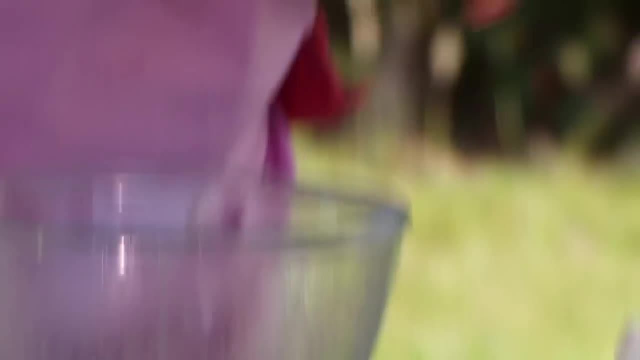 of the bread Ready: Sprinkle, sprinkle, sprinkle. It's all done, Finished, Finished, Finished And that is it. You did it, everyone. You put all of the ingredients together for your fruit jumble and you did it all by yourself. 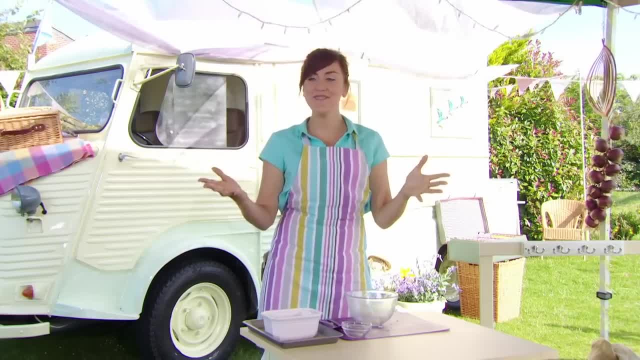 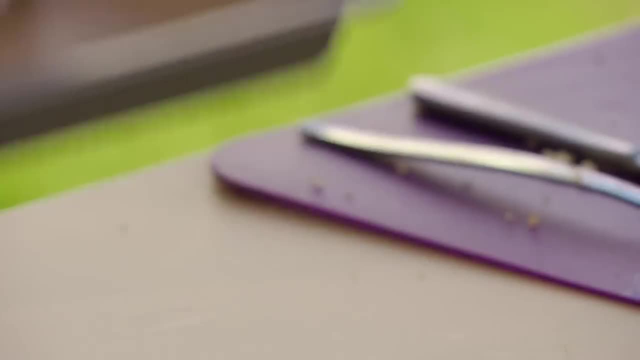 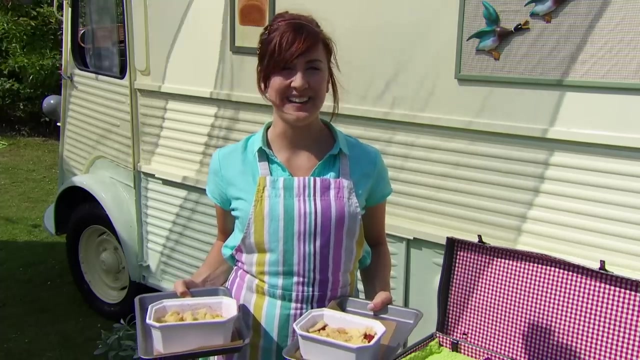 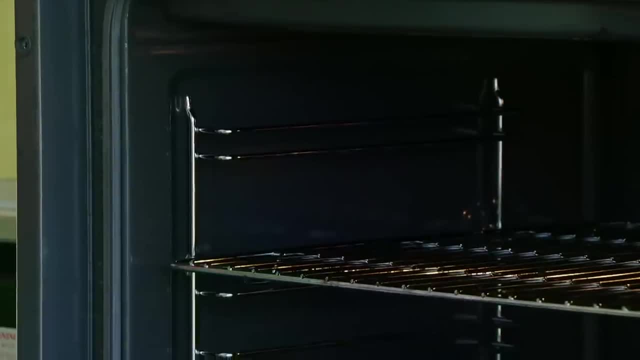 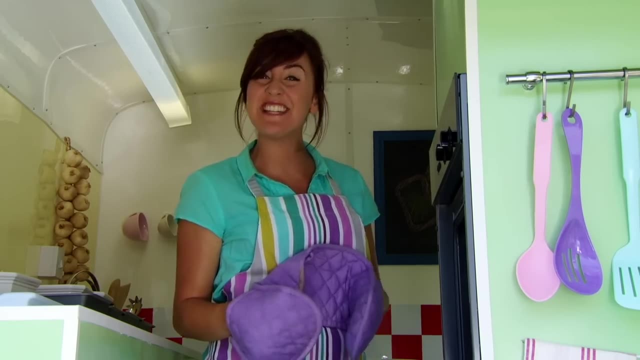 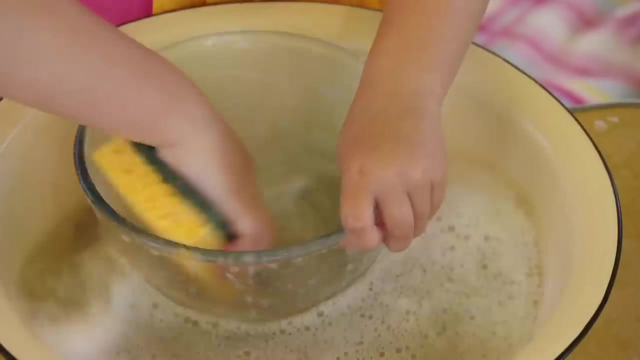 Now we've cooked with you and had lots of fun. Let's tidy up and think of all the things that we have done. There was cutting, lifting, sprinkling, mixing. Now clearing any mess and putting things away is always fun to do at the end of the 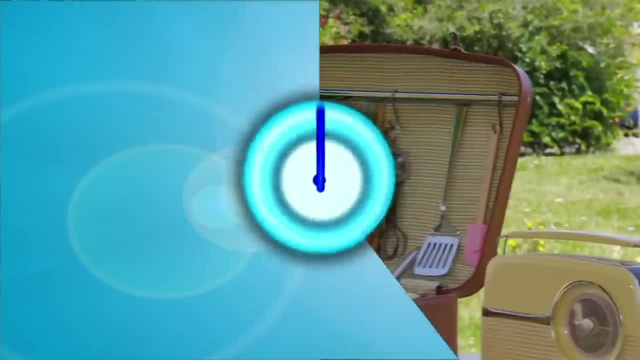 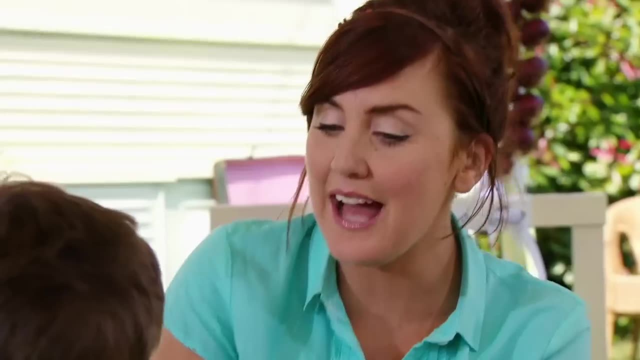 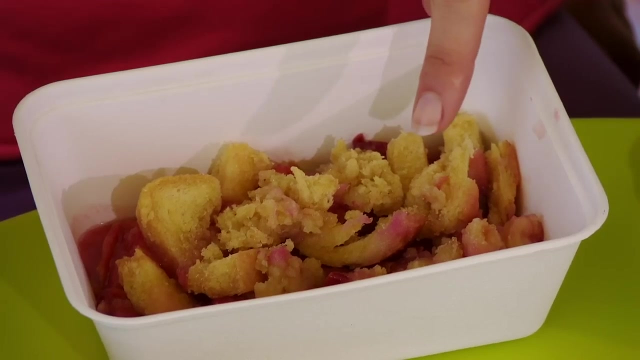 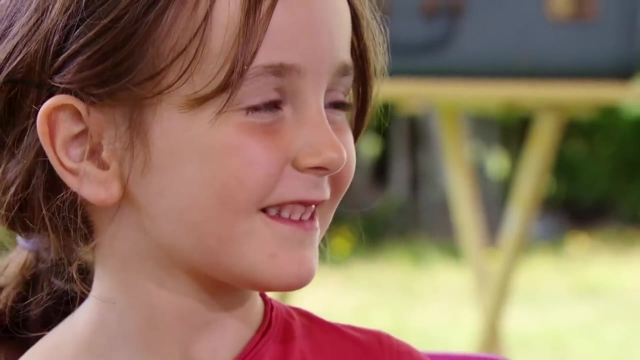 day, All right day, and here they are, everybody your delicious cooked fruit jumbles. okay, let's have a look at ivy's. well, i wonder what it's gonna look like. oh hey, you've got pink bits in yours. where have those pink bits come from? the juice? the juice from the plums? plums, that's right, and let's have a look. 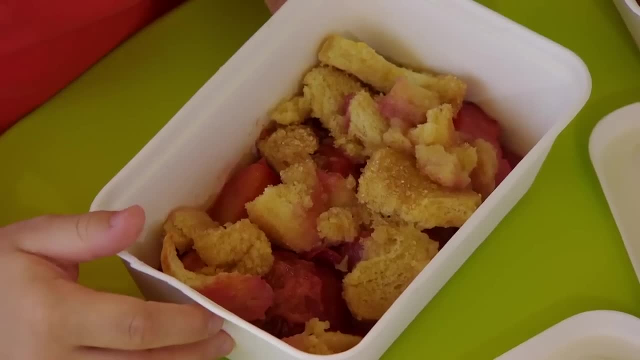 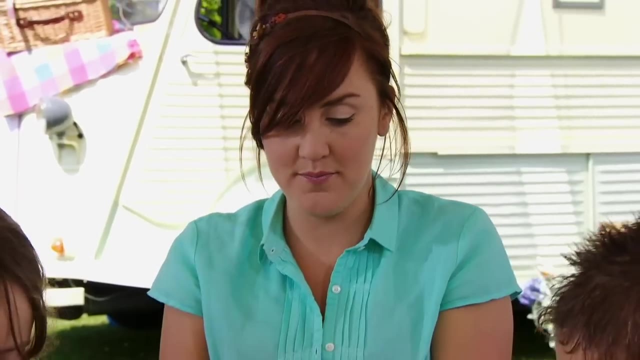 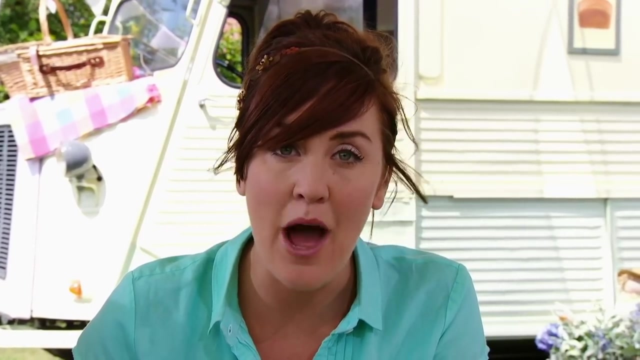 at jake's. hey, jake, check yours out. what do you think? it's nice, it looks very good. right, let's put the lids on top and we'll save these for later on when we go to the lighthouse. we've traveled to you, we've cooked and had fun. now let's have a party with everyone. 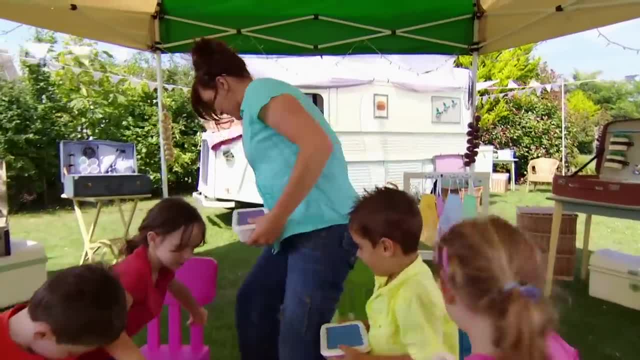 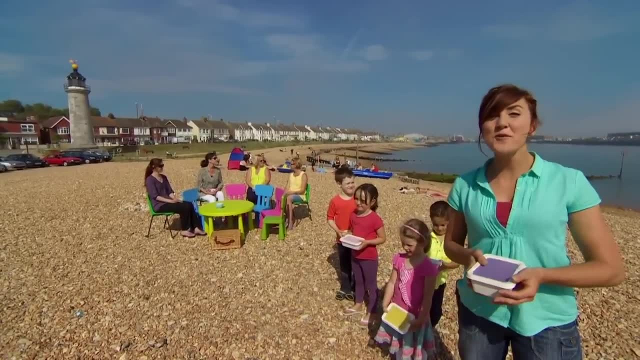 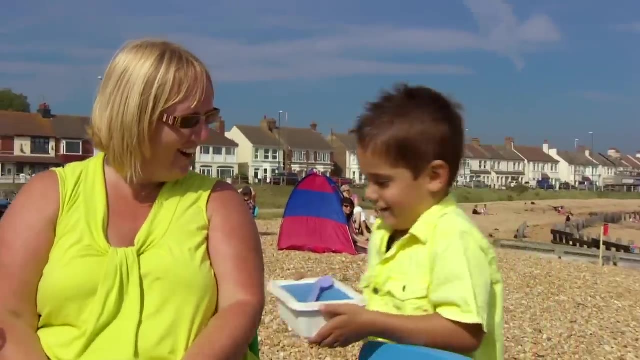 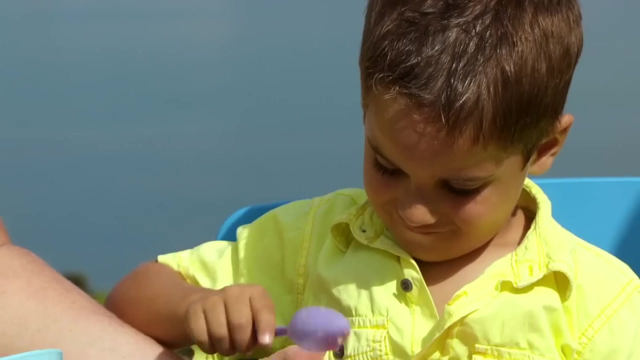 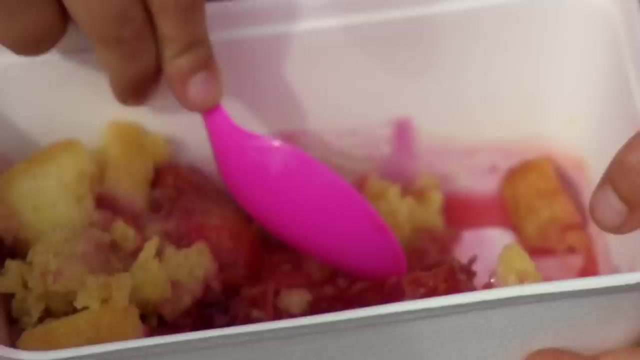 come on, you can come too. and here we are at the lighthouse and we've got our delicious fruit jumbles to share with everybody. come on, let's go. everyone did you? come on. that's beautiful. you're going to save some for your sister. no, no, what did you do to do them? wow, yummy, did you really make that? 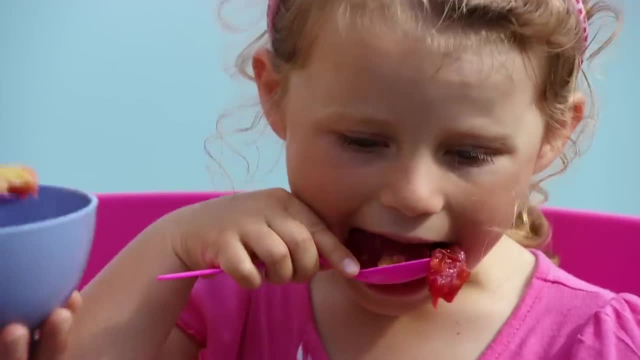 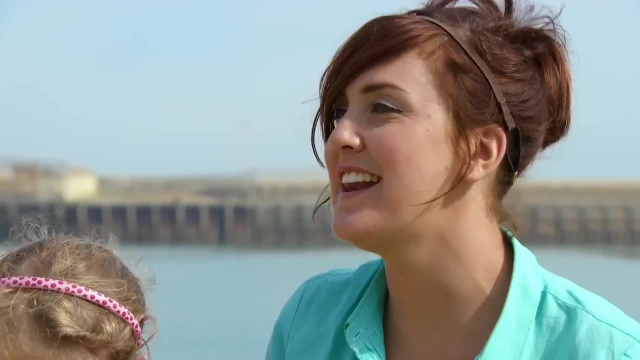 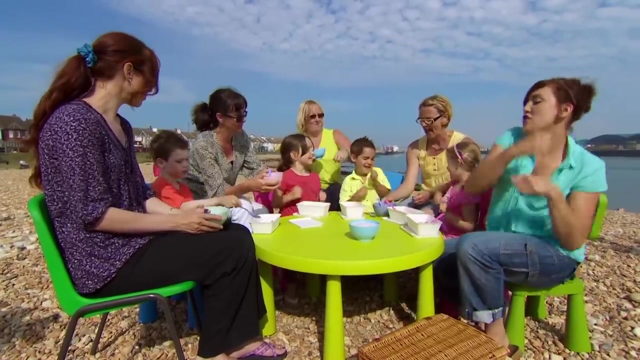 wow, that's lovely. thank you very much for making this billy. do you remember the part in the recipe where we did this? billy loved the twist dance. actually, should we all teach the mums how to do the twist dance? come on, let's do it. we go like this ready, do the twist, do the twist, do the twist. look how good billy. 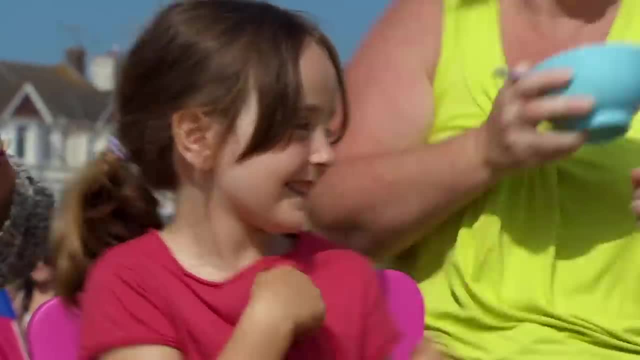 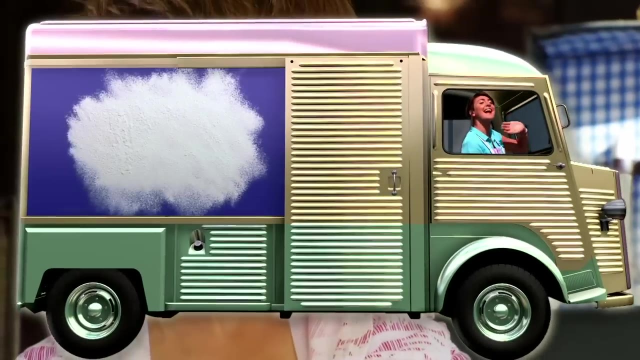 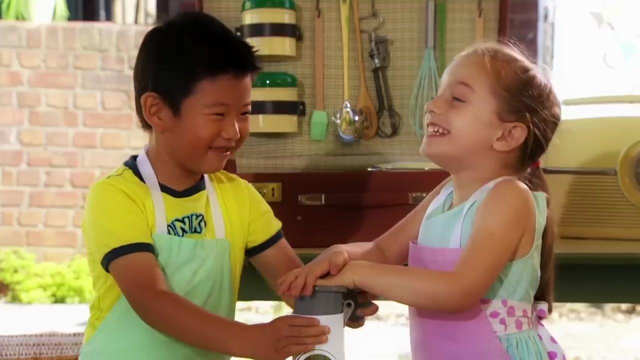 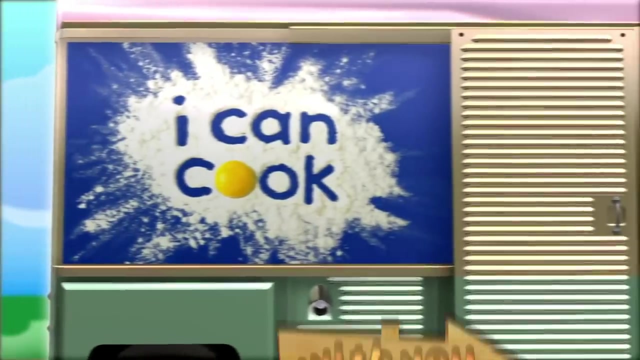 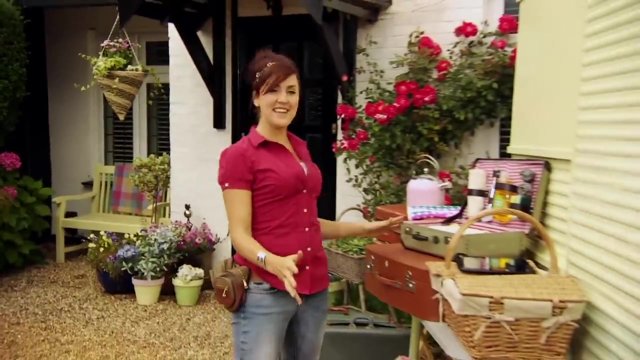 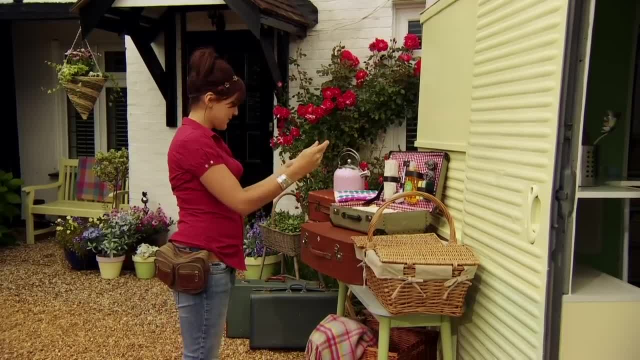 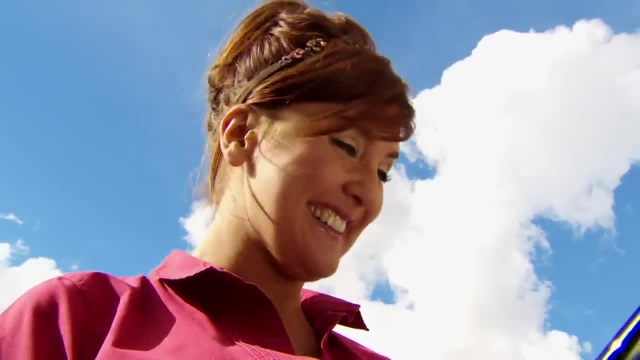 i can cook. aha, there you go. hello, katie, i can cook. I like to have a prince and princess party at the castle and I love chickens. Wow, that sounds amazing. Katie, can you cook with me please? Yes, I can, And you can cook with me too. 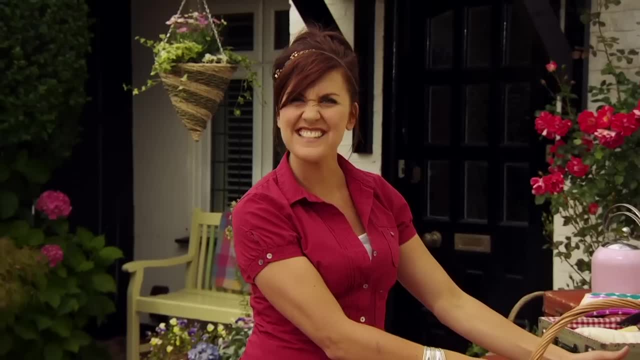 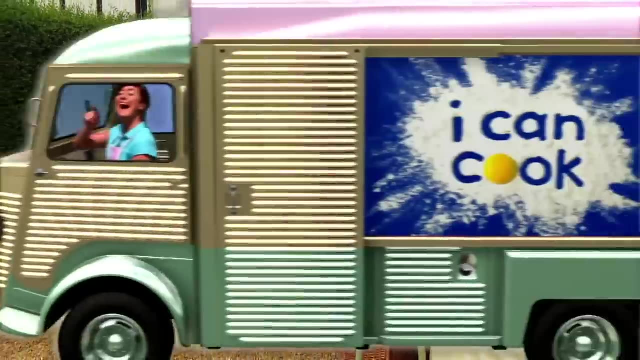 Oh, I hope I get to dress up as a princess. That would be really fun. Right, let's get everything packed up and put it in the van and then we'll get going Off on a journey and I'm coming to you. It's going to be busy and there's lots to do. 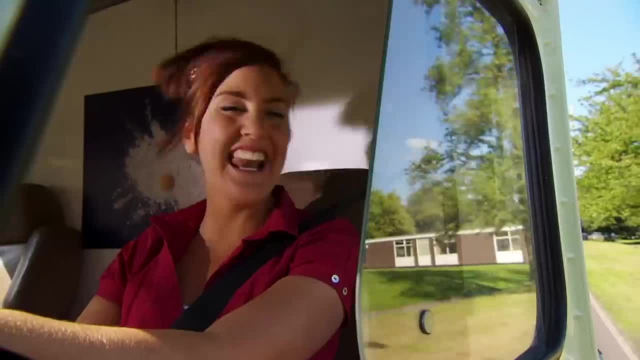 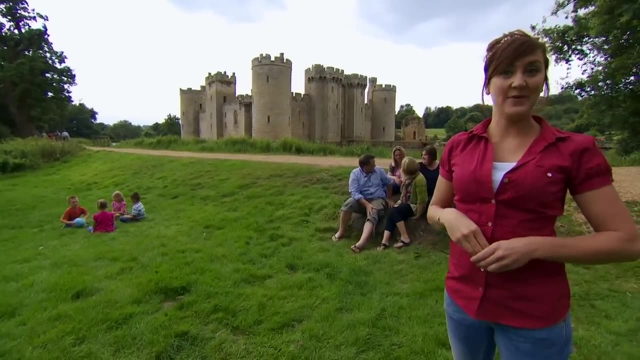 Get ready to help, join in and have fun. Let's look a feast for everyone. Well, here I am at the castle where I've been invited by Anya. Look there, she is over there with all her friends playing a game. Hi Anya. 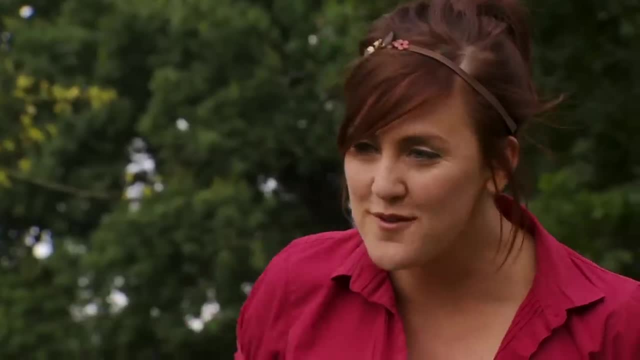 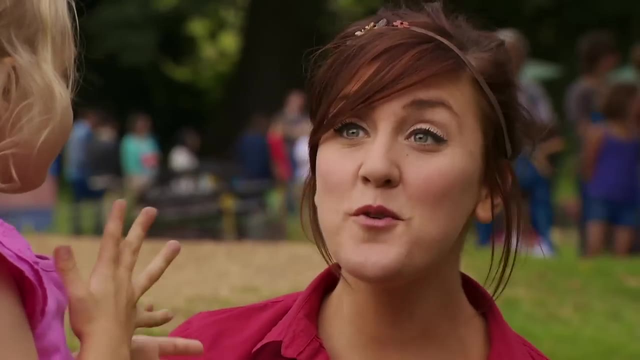 Hi, Katie, Oh, Anya, are these all of your friends? Yes, Oh, great. what's your name, Kai? And what's your name, Mia, Charlie, It is so good to meet all of you and Anya, I am so excited. 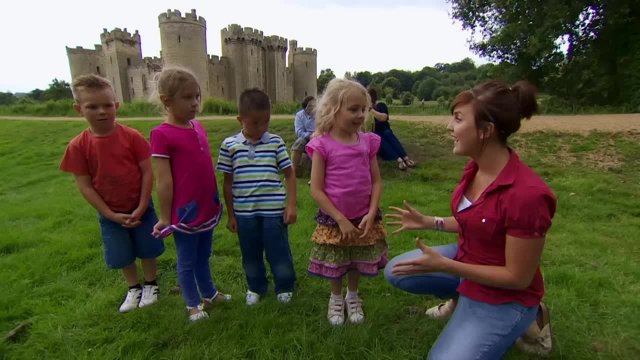 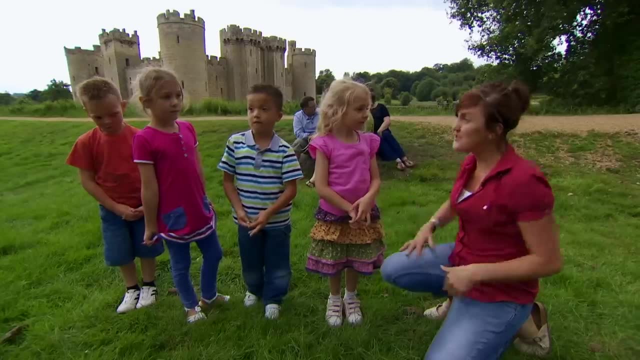 Are we actually friends? Are we really going to dress up as princes and princesses? Yes, and we're also going to have a banquet. I don't believe it. I've got a brilliant recipe to cook for a banquet. Come on, I'll show you. Follow me. 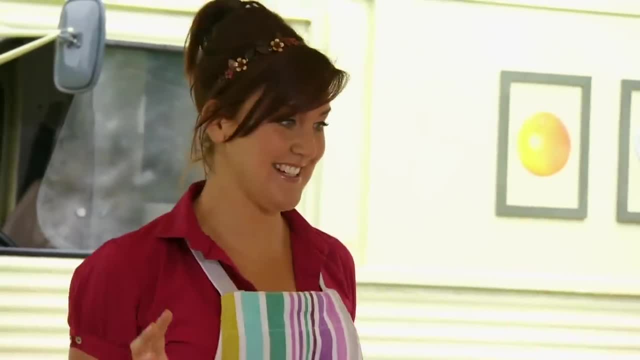 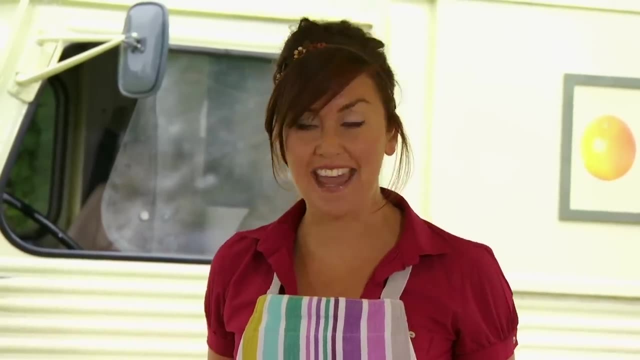 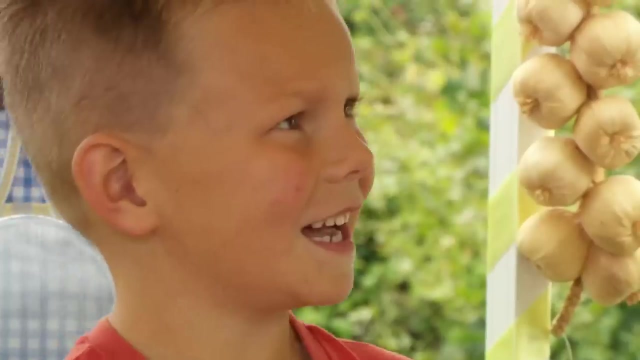 Welcome to my outdoor kitchen. everybody Who is excited about doing some cooking Me, I can't wait. Hey, do you want to know what we're going to cook today? Yeah, Okay, I'll tell you. Today's recipe is scrunchy crunchy chicken. 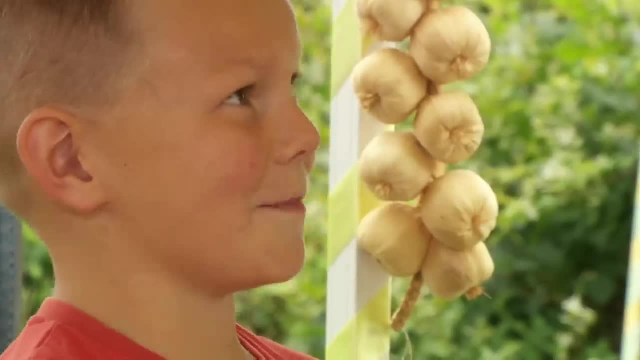 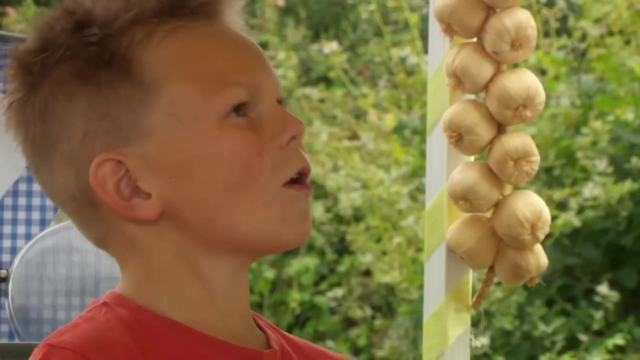 Yay, That looks yummy. It looks great, doesn't it? Now, before we get started on the cooking, we've got to do something really important. Do you know what it is? Wash our hands. We've got it. We've all got to wash our hands team, So let's get going. 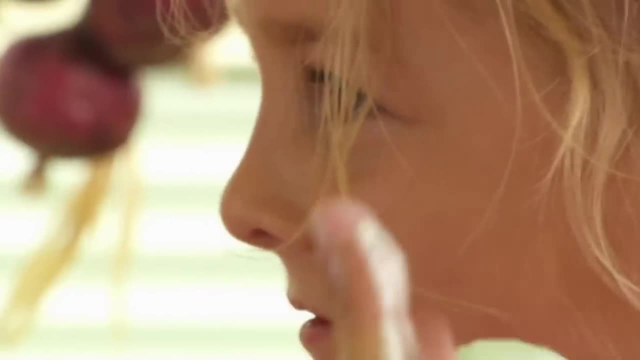 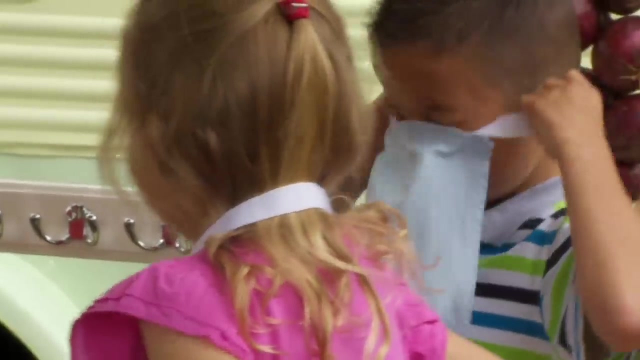 Roll up your sleeves. Give your hands a wash with sleeves. Give your hands a wash with slippy, dippy soap: Splish, splash, splosh. Have you done your hand Washed and dried? Sleeves rolled up, Apron tied: 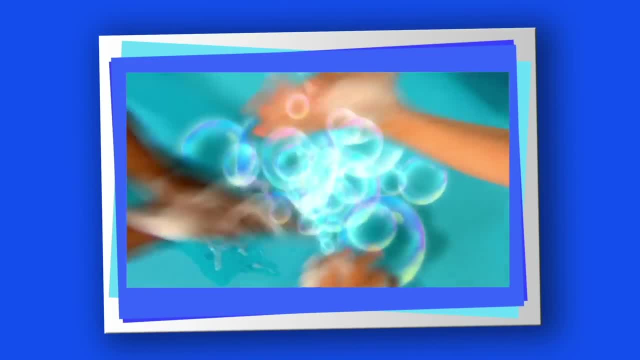 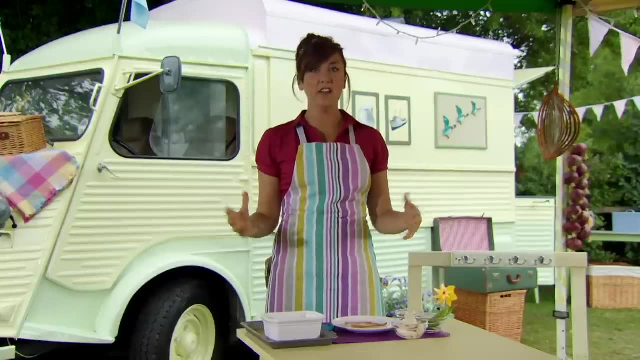 What can you do? I can cook, Right. well, let's get started To make our scrunchy crunchy chicken. Gosh, that's really hard to say. Can you say that really quickly? Scrunchy crunchy chicken. 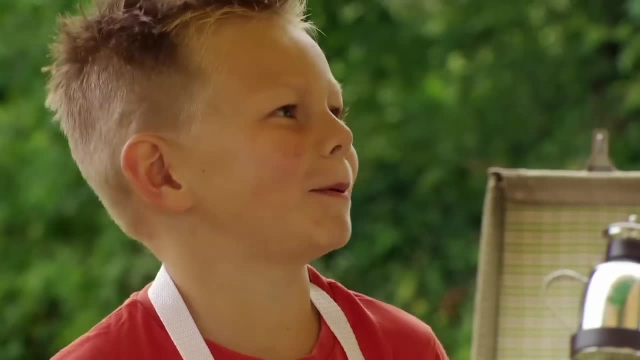 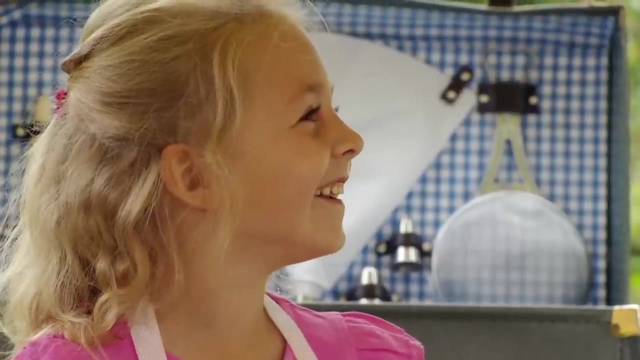 I bet you can't say it really fast. like this Scrunchy crunchy chicken Sounds like you're going like this: Chicken, chicken, chicken, chicken chicken. To make our scrunchy crunchy chicken, we need some chicken, of course. 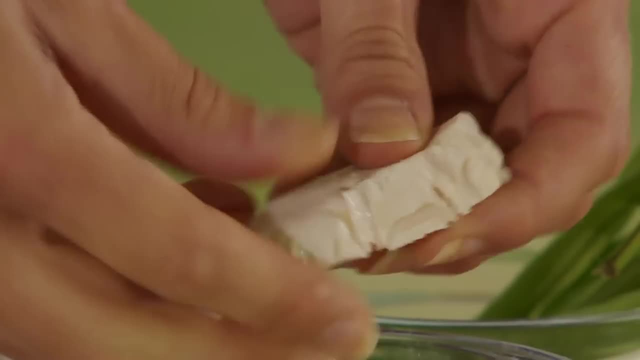 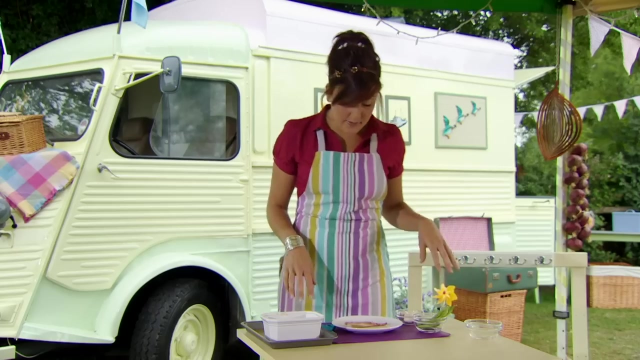 And we've got some lovely chicken that's already been cooked for us. Look at that lovely chicken. I love chicken. It's delicious, isn't it? Let's put this chicken into our dish And the next thing we need is some cooked bacon. 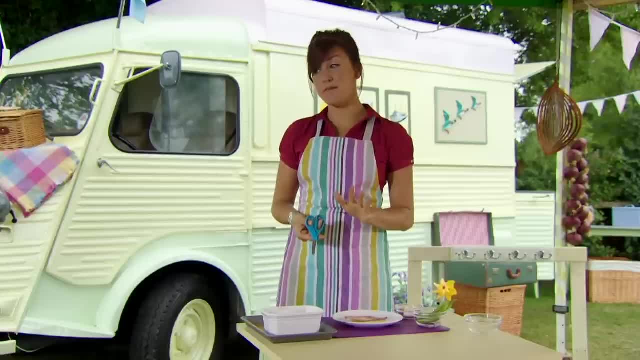 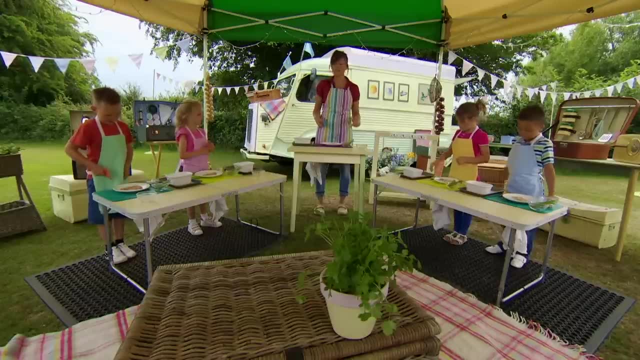 And we need to snip this bacon up. But remember, be safe with scissors. Everybody knows that you point them down towards your Toes. Let's see: you point your scissors towards your toes. Toes off and ready. OK, there we go. 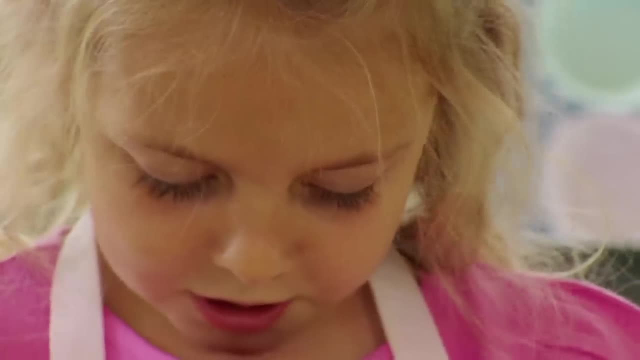 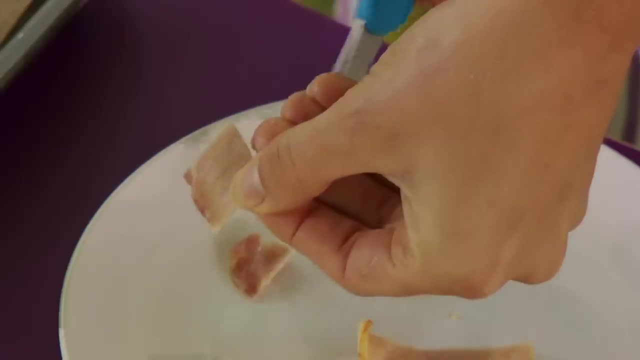 Remember to point them down towards your toes. Snip, snip, Snip, snip, snippity, snip. Make them into different shapes as well. I'm going to cut this one into a square. Look, there's a little square. 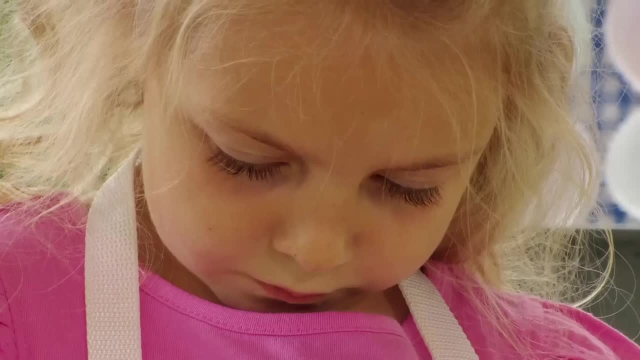 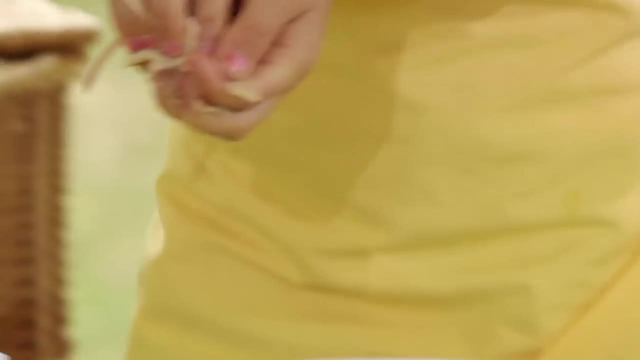 What shapes have you got? Look, diamond. Oh yeah, looks like a kite. What shapes have you got? Kai, That looks like a pencil. Let's scoop up the bacon and put it in with our chicken And then give your hands a good wipe. 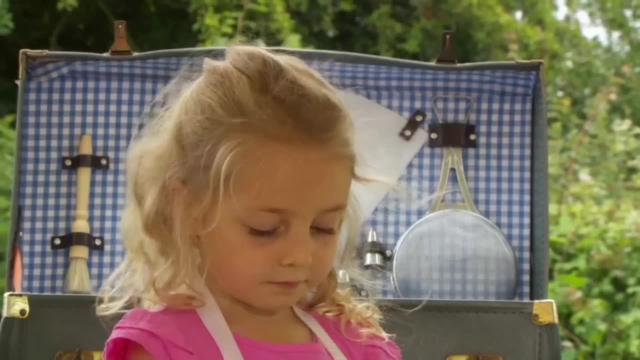 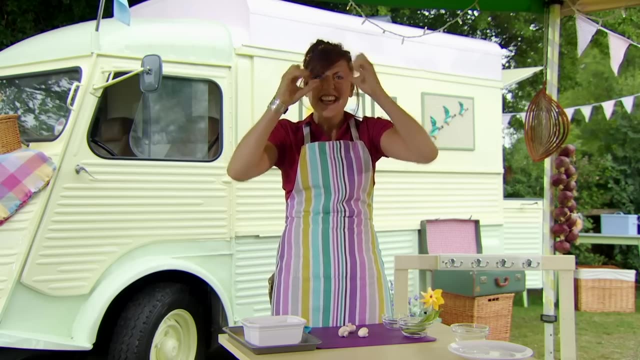 And next we've got a type of mushroom called a button mushroom. Imagine having mushrooms for buttons. That'd be a bit funny, wouldn't it? And we're going to use our fingers to crumble them up. Squash, squash, squash. 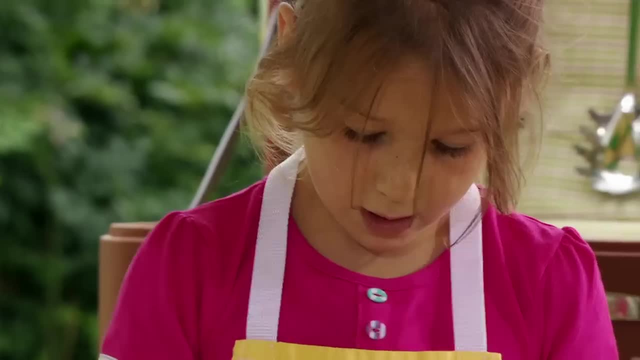 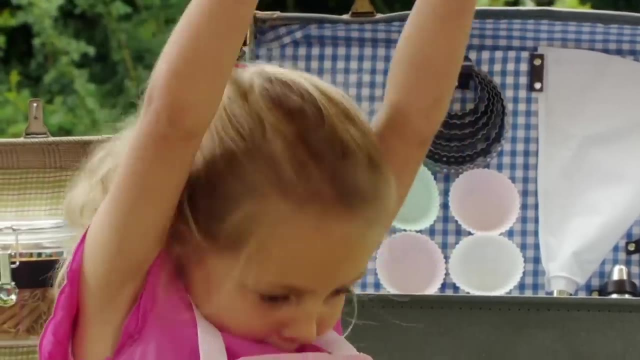 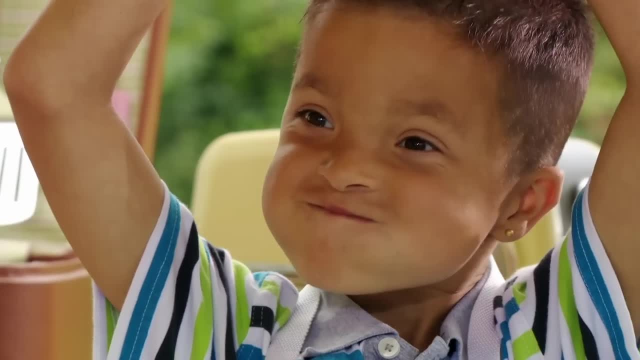 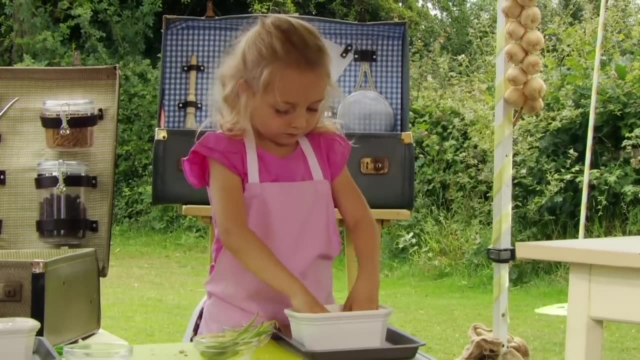 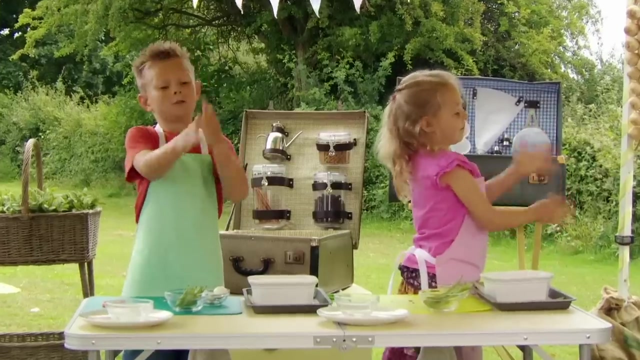 Put your hands above your head and you go. Use your fingers to mix the mushrooms with the bacon and the chicken. OK, who's ready for the next part? Yeah, OK, just do this with your hands to get all the little bits of mushroom off. 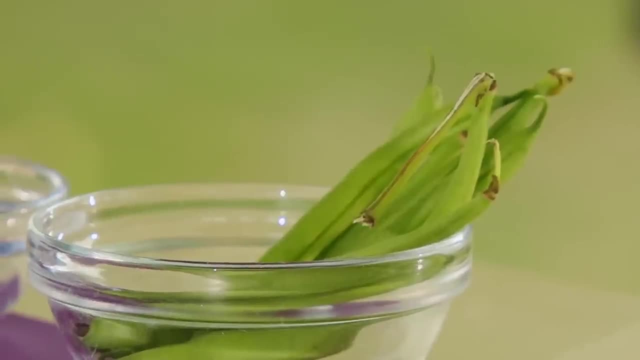 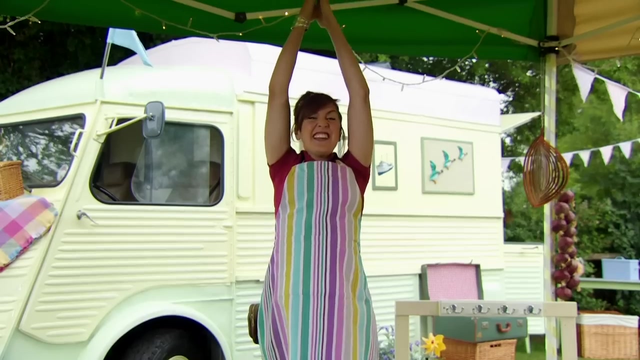 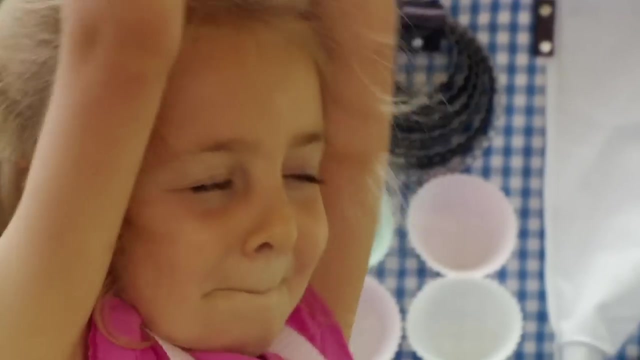 OK, The next ingredient is some green beans. Does anyone know how to do the green bean face? You put your arms up like this, Really, really, really tall, and you go like this: Look at Charlie when he does it look. 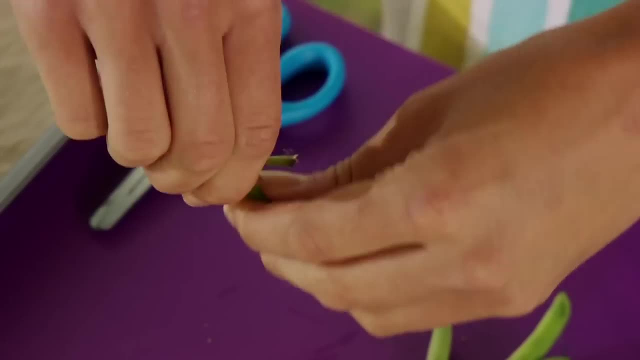 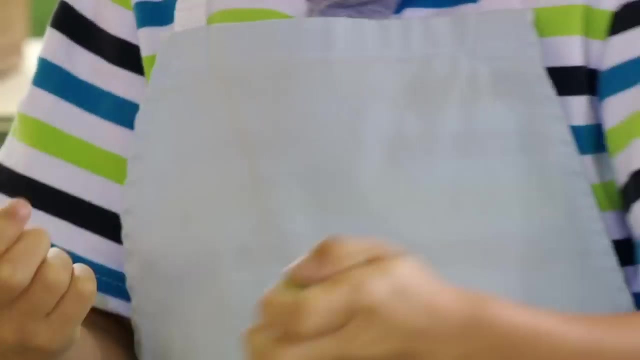 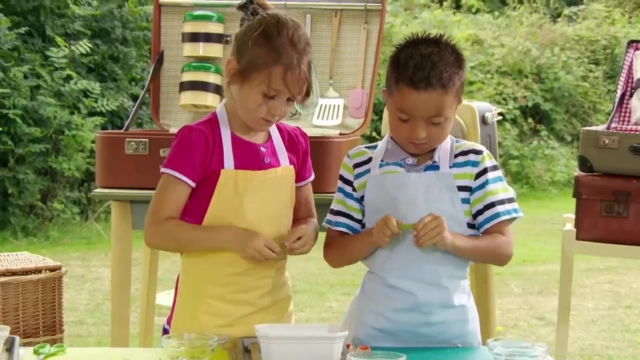 We're going to play the pinch and snap game. Pinch and snap, Pinch, snap, And then you've got to try and do it as quickly as you can. Pinch, whoop and snap, Pinch and snap. There we go, another one. 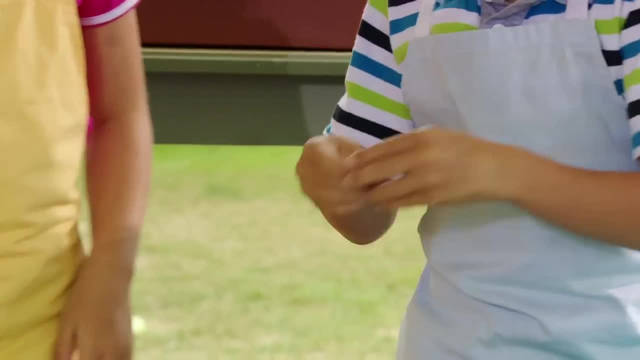 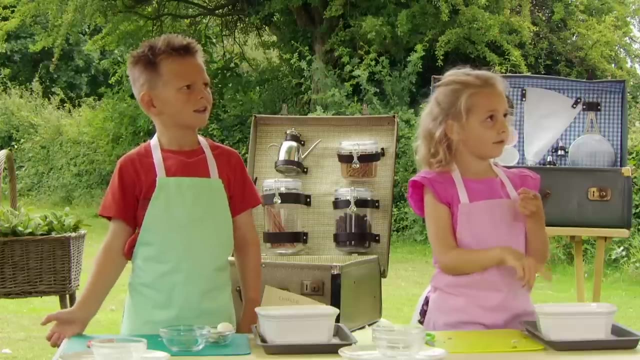 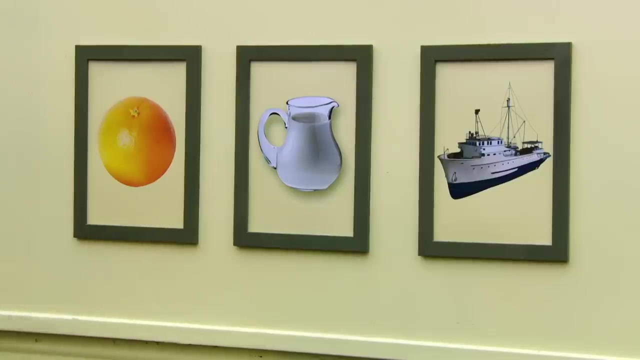 And last one: Pinch and snap Great. So what ingredient do you think we're going to need next in our scrunchy crunchy chicken recipe? Well, let us see if you can guess what it could be. Well, we've got an orange, some cream. 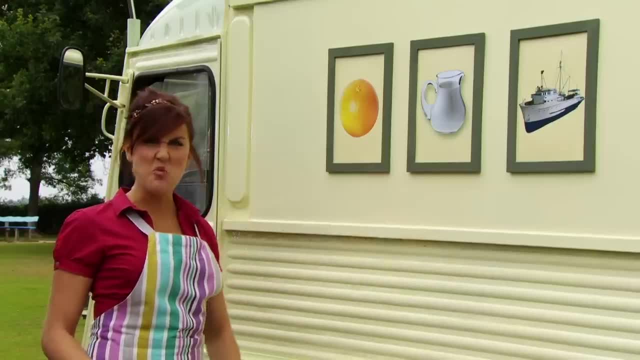 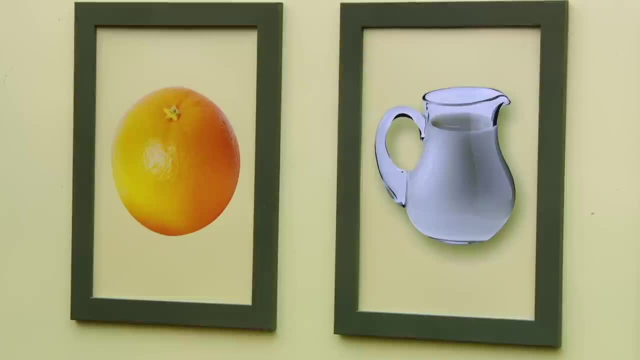 And a boat Boat. What would you use for our scrunchy crunchy chicken? The special ingredient is white. Well, an orange is orange, isn't it? So it can't be that one. We'll take that one away. 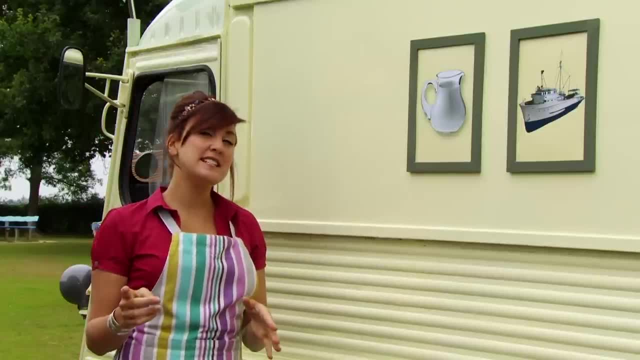 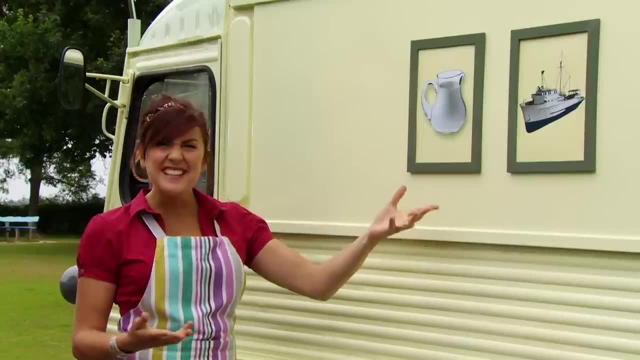 OK, here's another clue. The special ingredient is white and it comes from cows. Well, a boat doesn't come from cows, does it No? So we'll take that one away too. A bit funny having a boat in the recipe. 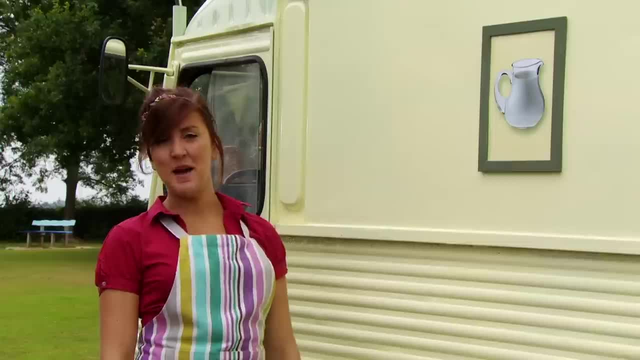 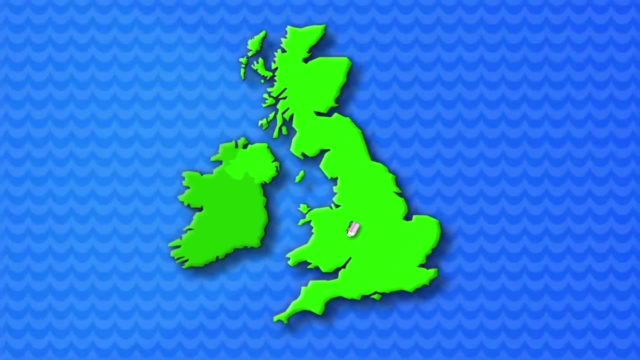 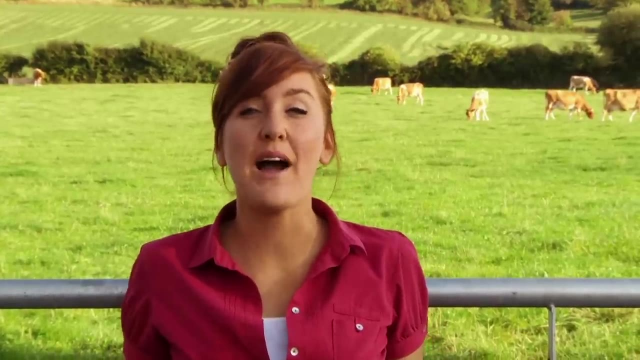 Well, that leaves us with cream. We're going to need some lovely cream for our scrunchy crunchy chicken, And earlier I went to find some. I've come to Rawton in Wiltshire to find out how cream is made. 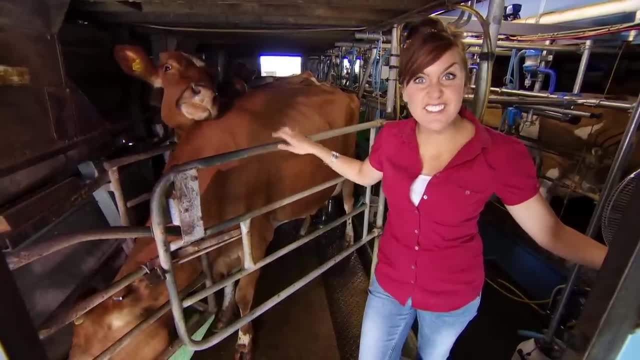 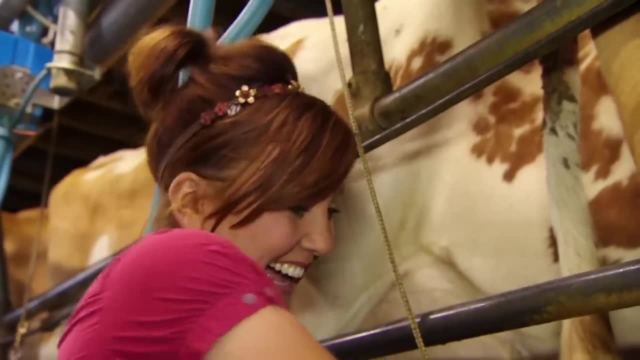 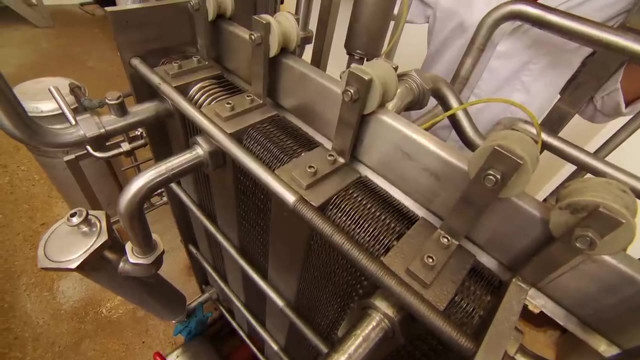 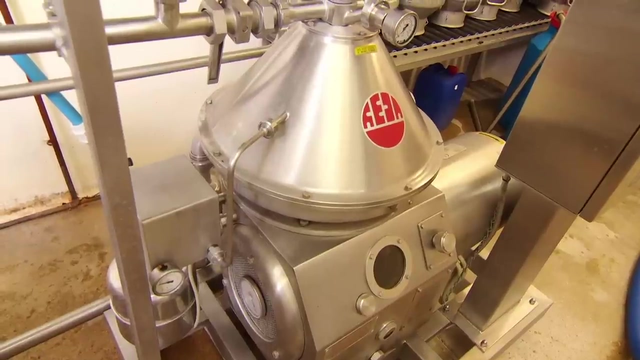 Cream comes from milk and these cows are being milked right now: Ready Daisy. OK, The milk goes into this machine, It's called a pasteuriser, And it heats the milk up and makes it safe to use. Next, the milk goes into another machine called a separator. 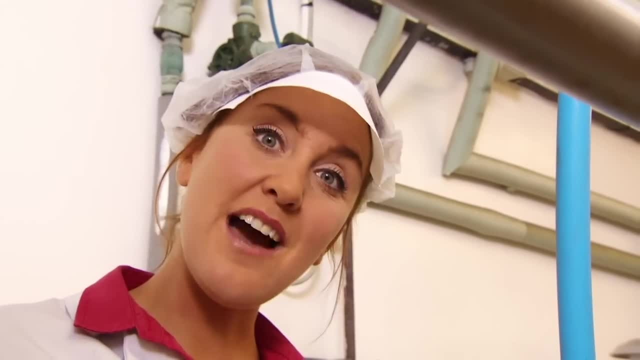 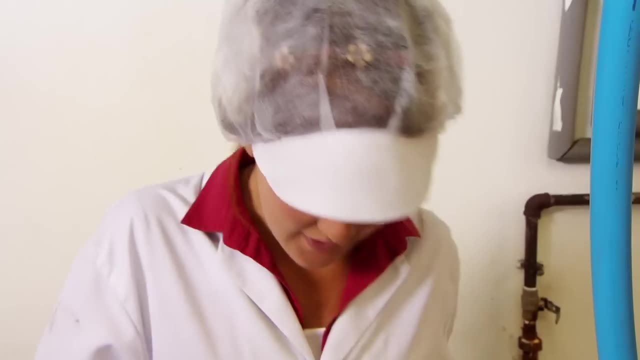 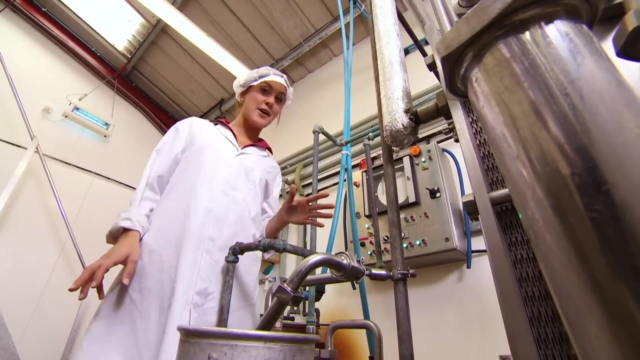 In here. the thinner skimmed milk is pushed to the outside and the thicker cream stays in the middle And the thick cream comes out of this pipe. Look, there it is. Can you see it? After that the cream is cooled down and it comes out right here. 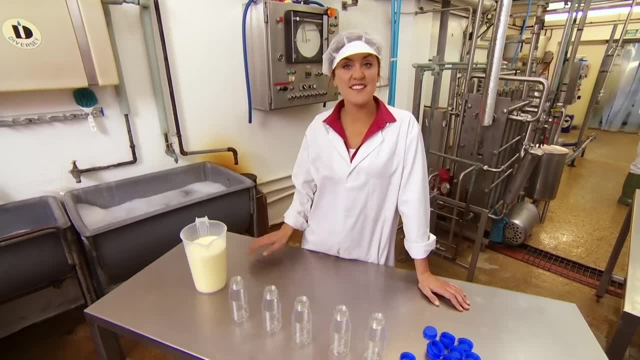 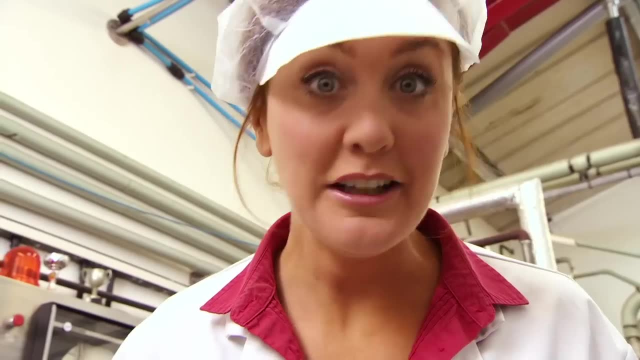 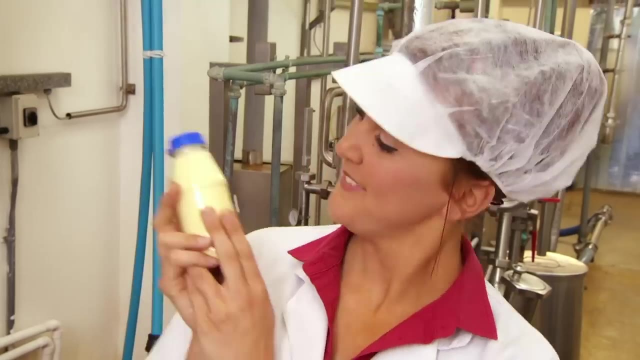 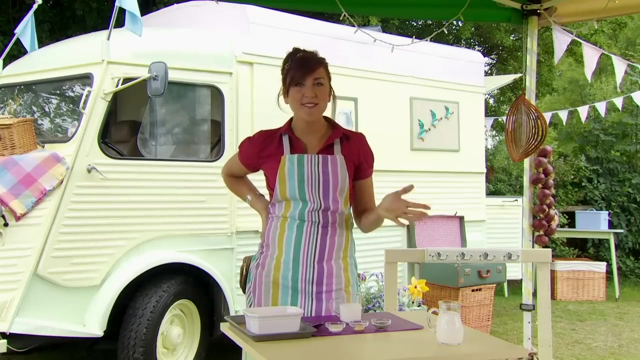 And finally we pour it into bottles like these and it's ready to use in our scrunchy, crunchy chicken recipe. Ah, delicious. Making cream is so much fun. I loved it, And so we've got our cream here, ready to use in our recipe. 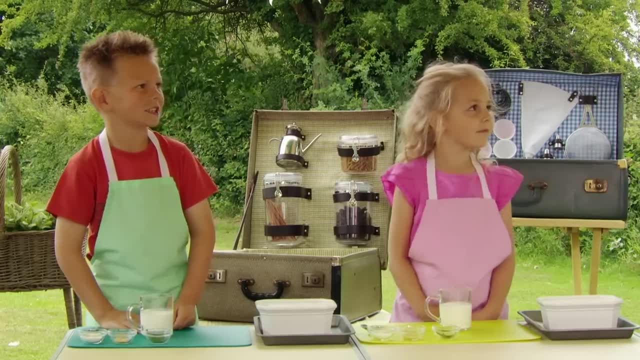 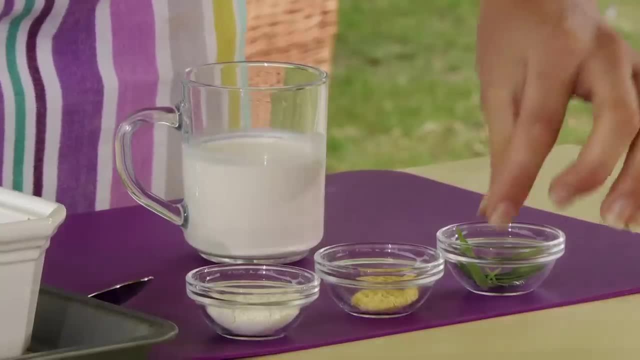 And we're going to make sort of a potion with it. Everyone say woo, Woo, Because we've got lots of ingredients here that we're going to add into our cup of cream. The first one is a herb called tarragon that we've got in this little bowl. 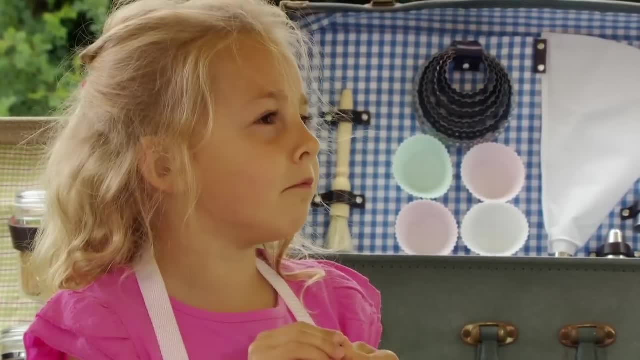 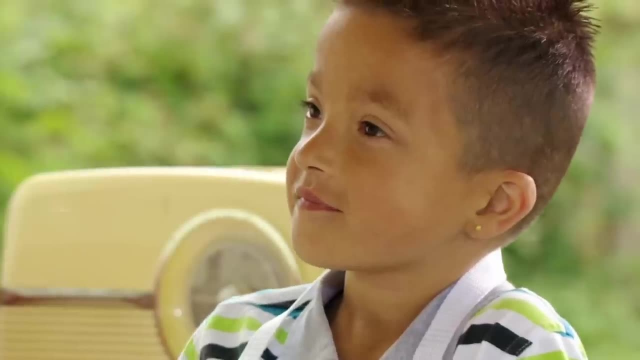 Oh Anya, what do you think Sminky? It's got a really strong smell. Let's add this into our cream. There we go, And the next thing we're going to add is some stock powder, which is this ingredient we've got here. 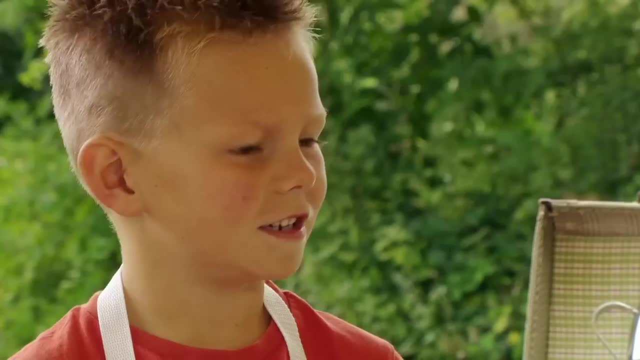 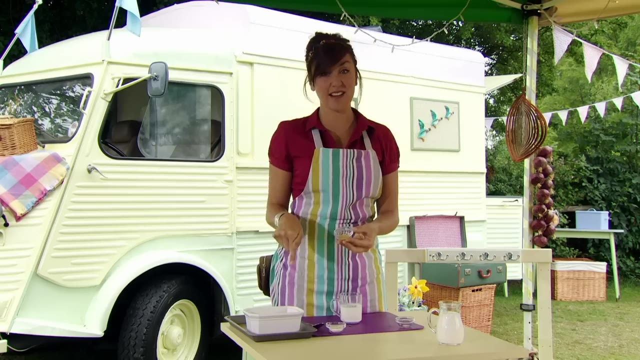 Oh, it's very strong. Smells like onion. Yes, it's because the stock powder has onions in it. That is going to add loads of flavour to this recipe, So let's sprinkle that into our little creamy potion. Mine's all done. 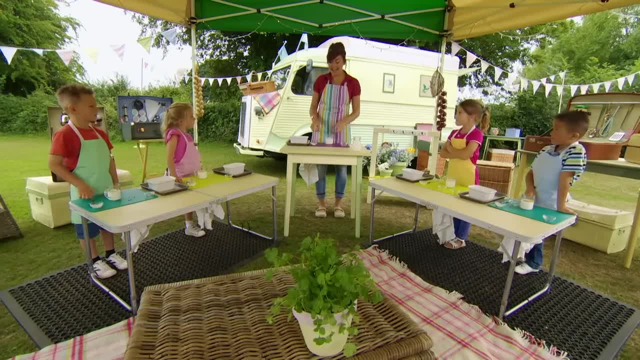 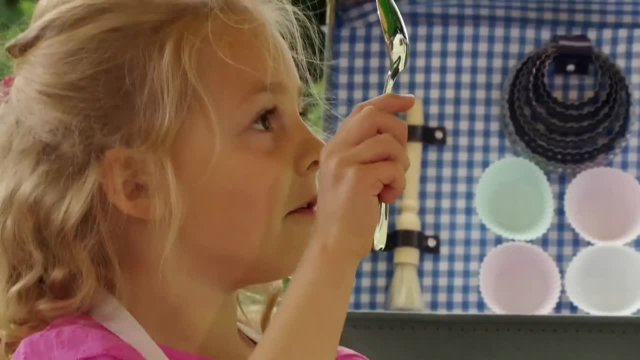 It's all gone into there, And the final ingredient we need to add is Flour, Flour. So let's sprinkle that in too. Oh, look at that Lovely Shall. we mix it now. Absolutely, We've got to mix it with our spoon. 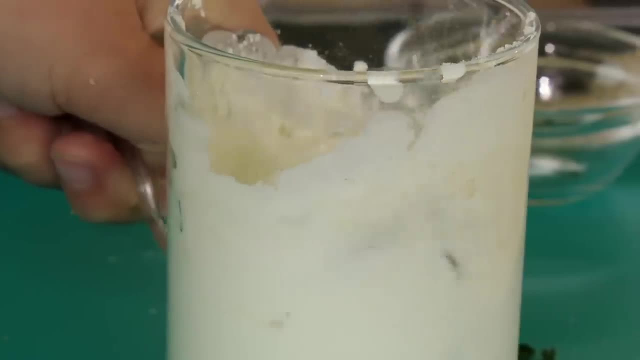 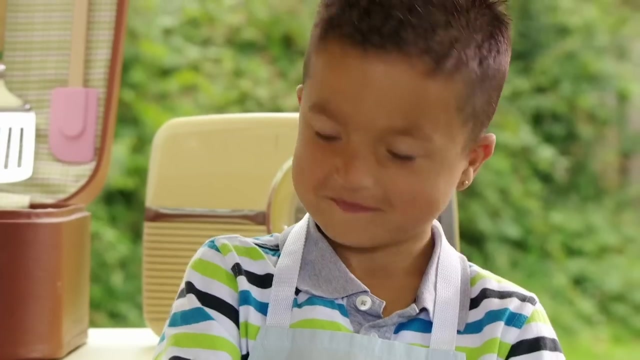 So we're going to give it a good stir. It looks like banana milkshake. Banana milkshake- Yeah, I don't think it's going to taste like a banana milkshake, though Let's pour it into our dish all together, as a team. 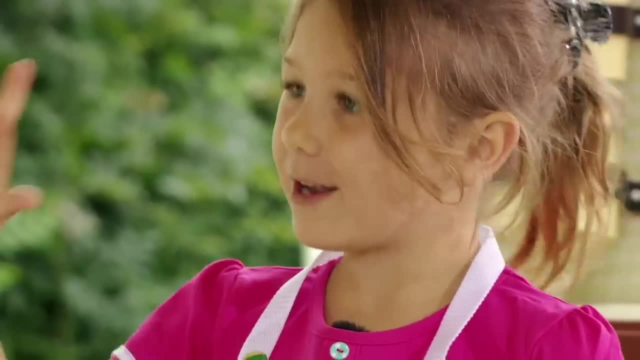 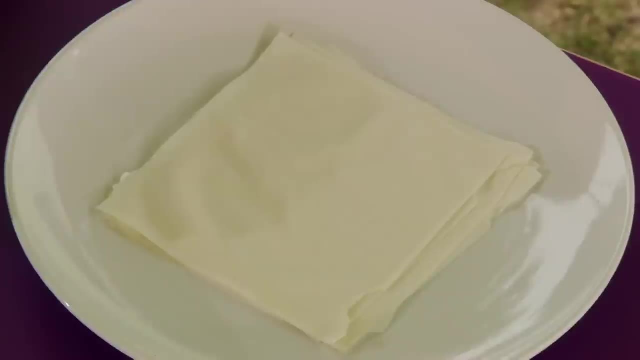 One, Two, Three Splash. One, Two, Three Splash. Good job, everybody. And the last thing we need is some phyllo pastry. We are going to bring one piece of phyllo pastry at a time onto our mat. 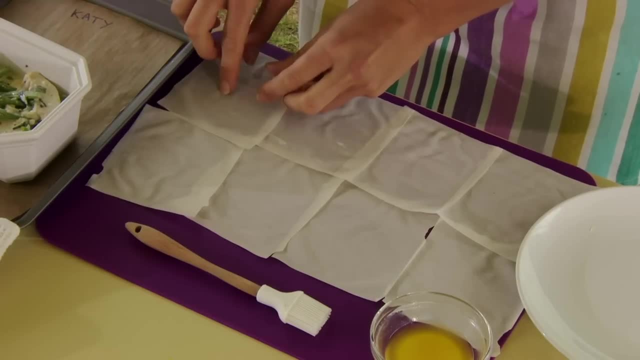 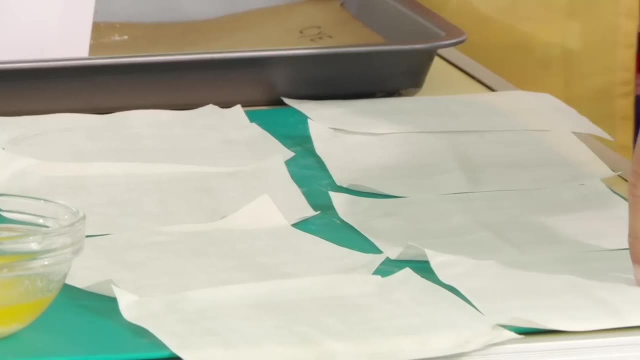 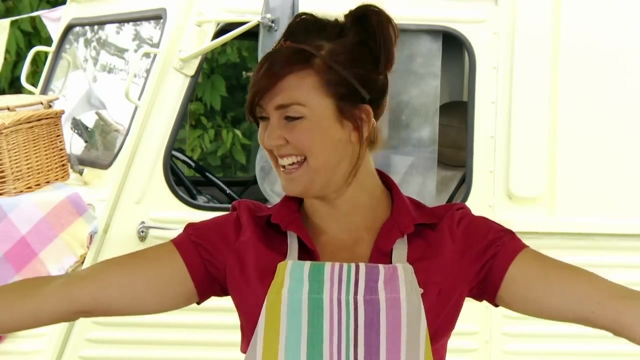 We've got eight pieces, so we need to do four at the top and four at the bottom all in a line: One, Two, Three, Four, Five, Six, Seven, Eight. Great, Who likes painting Me Me? 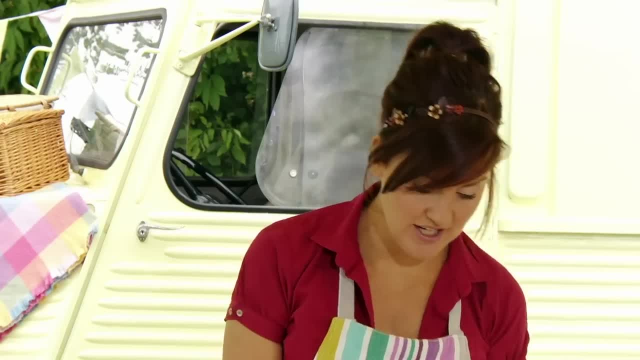 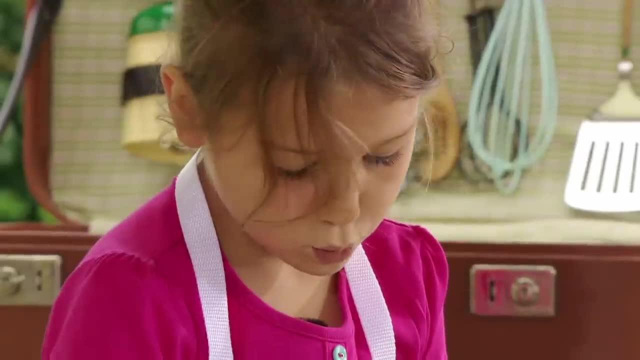 I love it And we're going to paint using this melted butter. So take your brush and dip it in the butter and go swirly, whirly, swirly, whirly, Swish, swosh, swish, swosh. 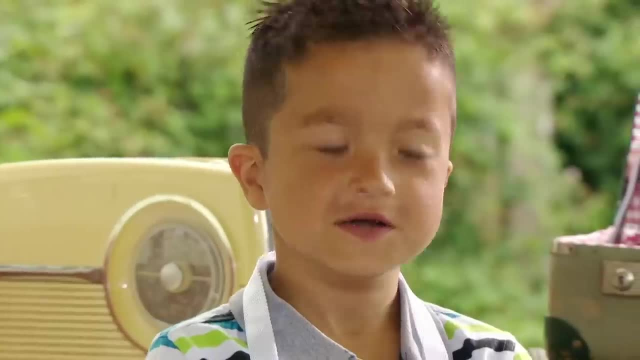 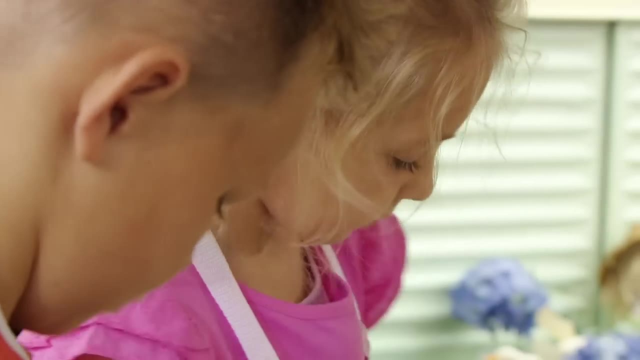 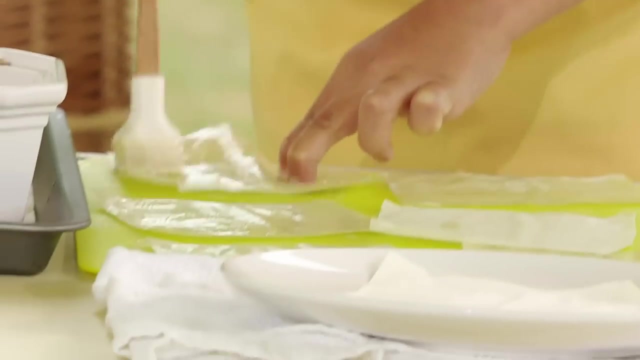 Kai. why do we paint it with butter? Because then it goes all soft. It's going to go shiny, a bit like butter actually. There you go, Ooh, we're getting buttery fingers. That's it, And once they've all been painted, you can put your brush and your butter to the side. 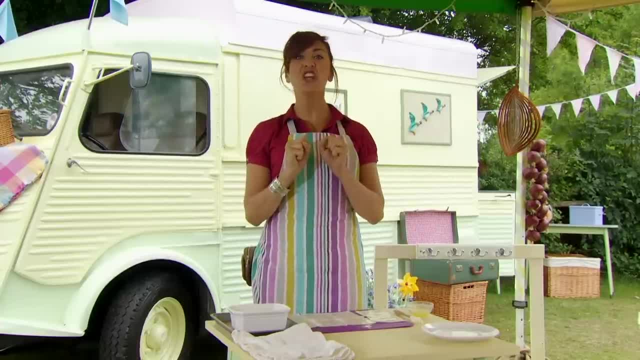 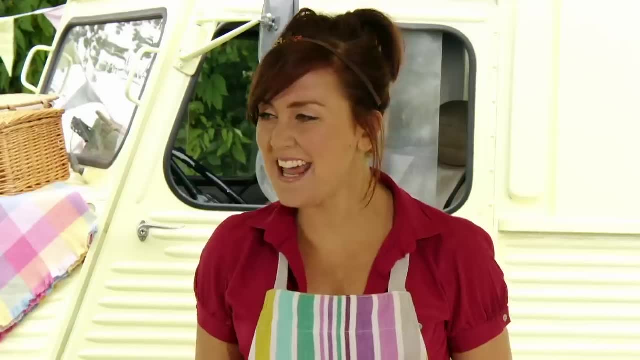 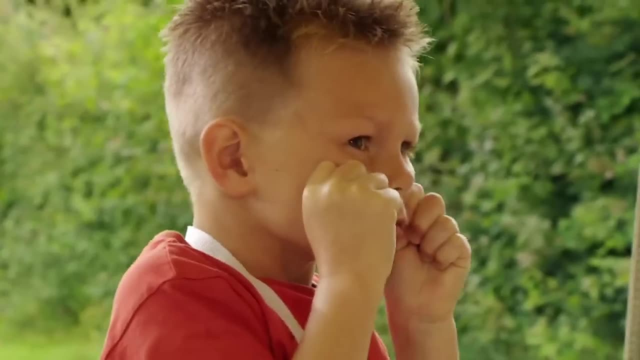 and we are going to do some scrunching. We're going to scrunch each of these phyllo pastry squares into scrunchy little balls. Can everyone do this? Yep, Well, that is what we're going to do with our pastry squares. 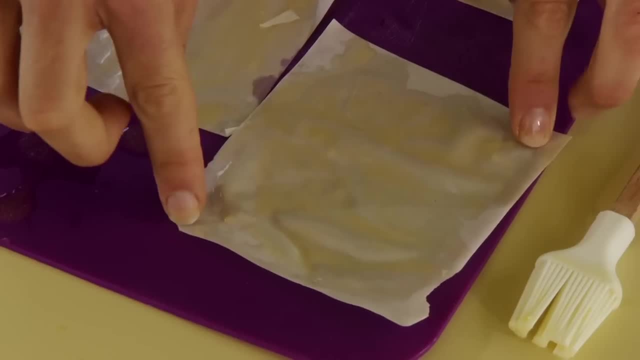 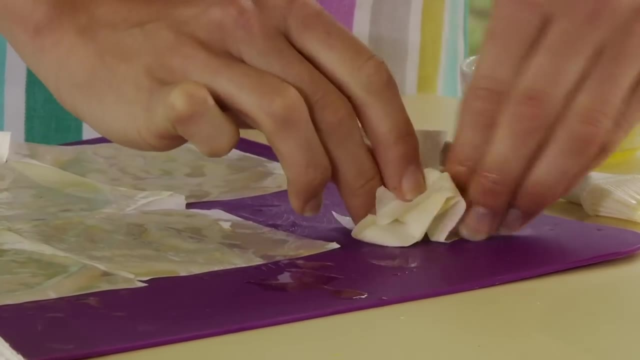 Watch, We put our two fingers at the side like this, Scrunch it together, like that. Then we get our fingers and put them on the other side and scrunch them together, And so they all suck up into the middle like this. That's it. 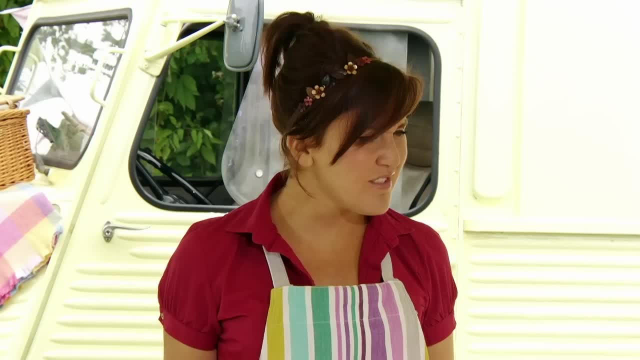 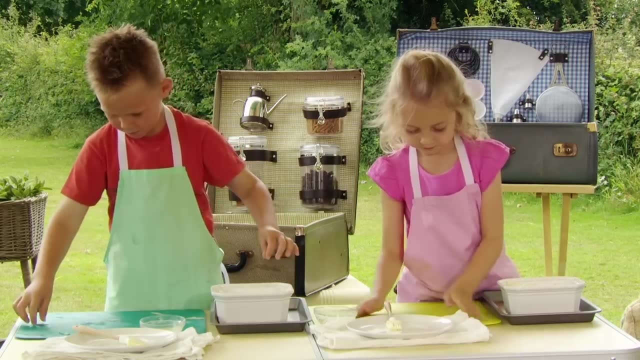 You're doing it. You're doing it. everyone Look Looks really really good. Well done. I finished mine. I have Put any extra bits of pastry on top And that's it. You've done it. You've put all the ingredients together for your scrunchy crunchy chicken, all by yourself. 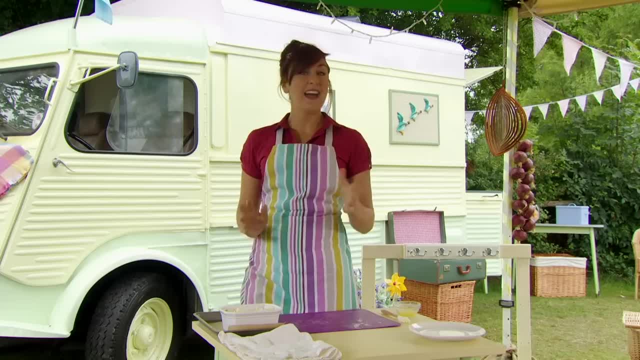 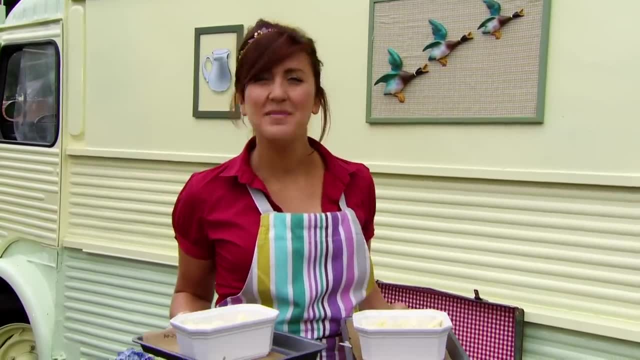 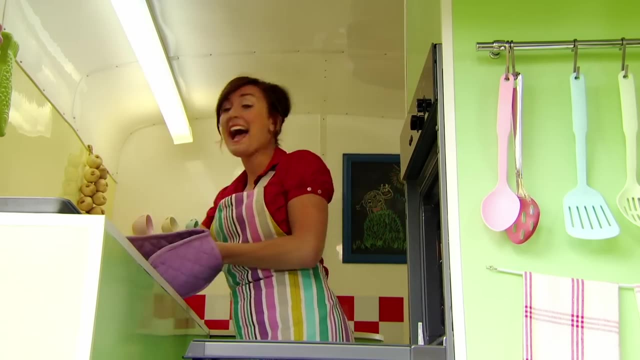 Well done, Yeah, And now I'm going to put them in the oven for you, But remember, ovens are hot, so don't go near. Ask a grown-up to help you here Now. we've cooked with you and had lots of fun. 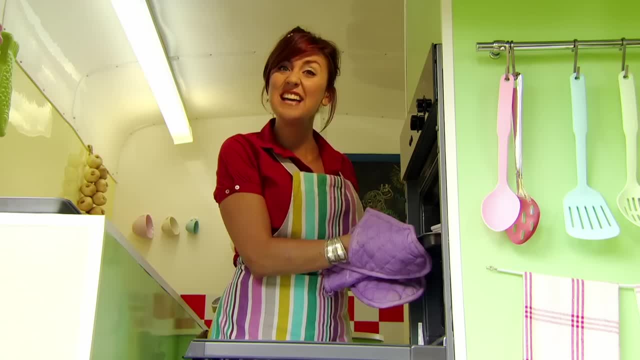 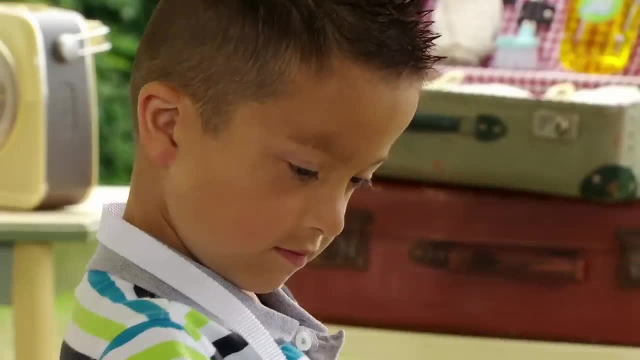 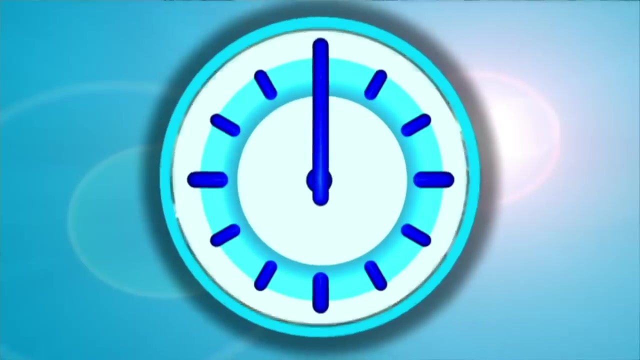 Let's tidy up and think of all the things that we have done. There was Clearing, Snipping, Snapping, Brushing, Clearing any mess, and putting things away is always fun to do at the end of the day, I am so excited everyone. 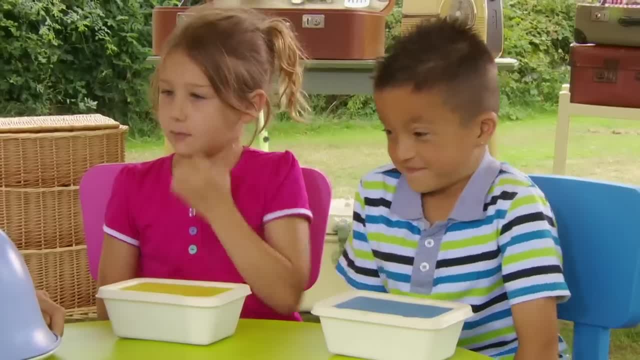 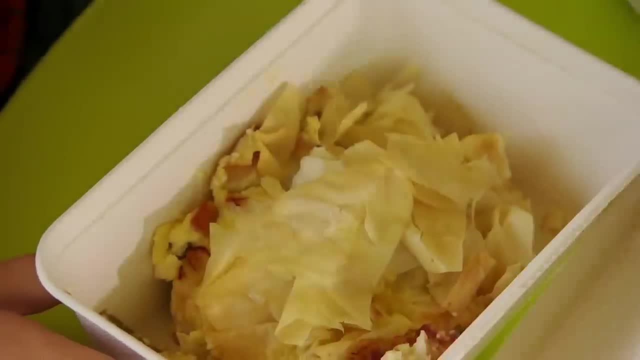 Our scrunchy, crunchy chicken dishes are all cooked. Shall we have a look at them? Yes, OK, let's see how they've changed. Why don't we have a look at yours first, Charlie? It's going all crunchy. 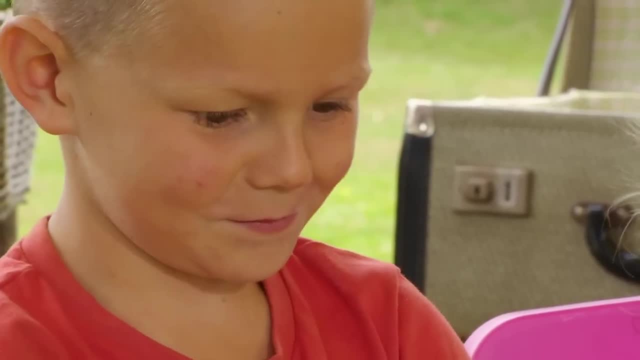 We said that, didn't we? It was going to go all crunchy. It looks really great. I bet it tastes good too. What's happened to yours, Mia? Let's have a look, Didn't it? What colour's it gone? 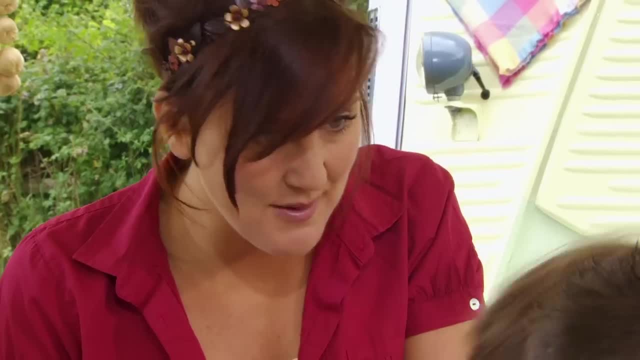 Brown and yellowish. Does it smell good? It smells like pizza. Let's smell. Oh, it does smell a bit like pizza. Why don't we put the lids back on our scrunchy crunchy chicken dishes and we'll save them? 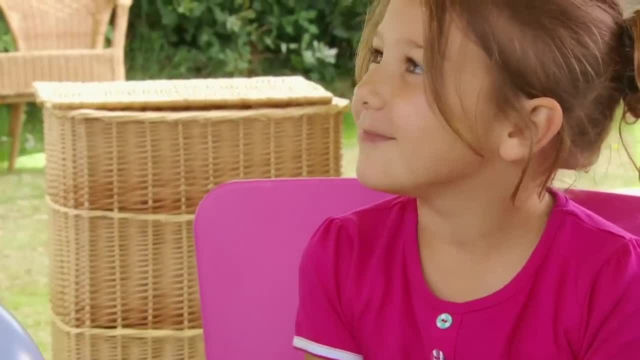 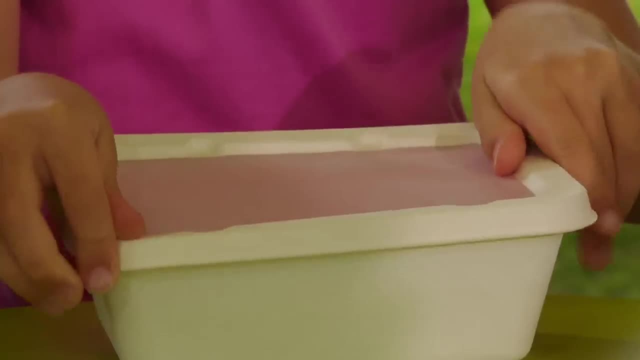 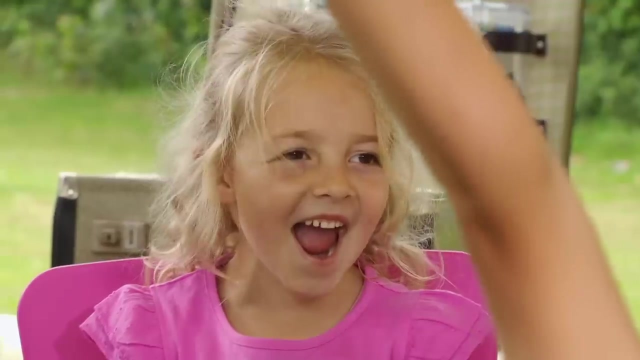 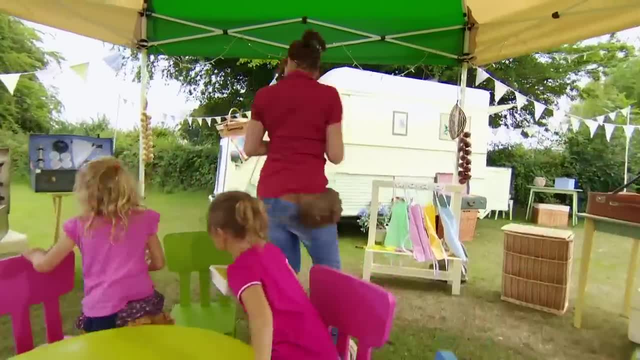 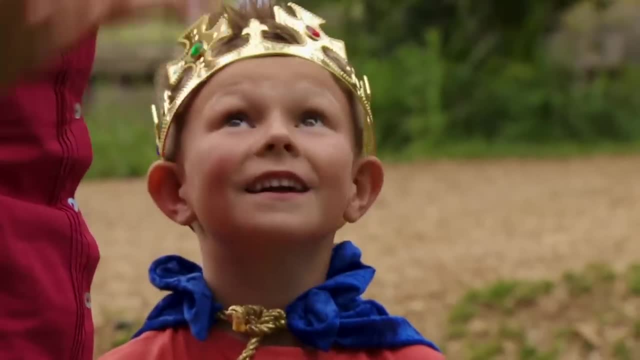 Come on, you can come with us, Follow me everyone. Well, here we are at the castle and we are all ready for our banquet. We've got our lovely food to share. Come on, everyone, let's go. Would you like some of my food, Mum? 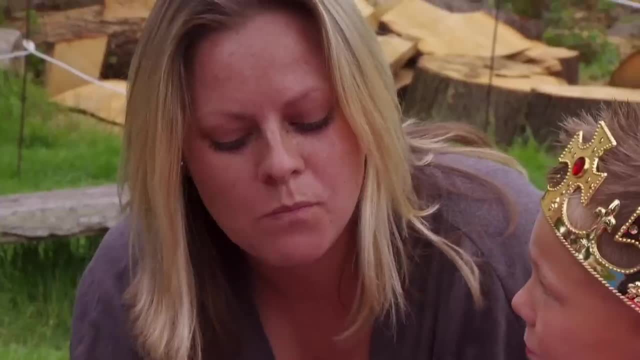 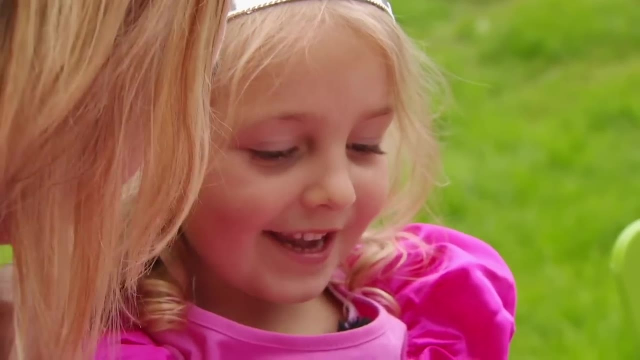 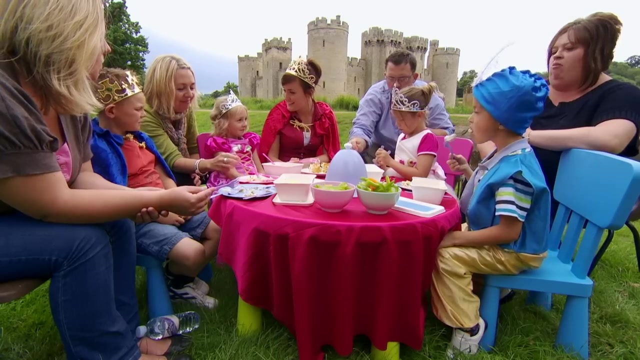 I would love some. Mmm. That's lovely and crispy. It looks delicious. How did the pastry change? It's gone. shiny and crunchy. It tastes good, It's good. This pie is really lovely. So, Anya, what was your favourite part of the cooking today? 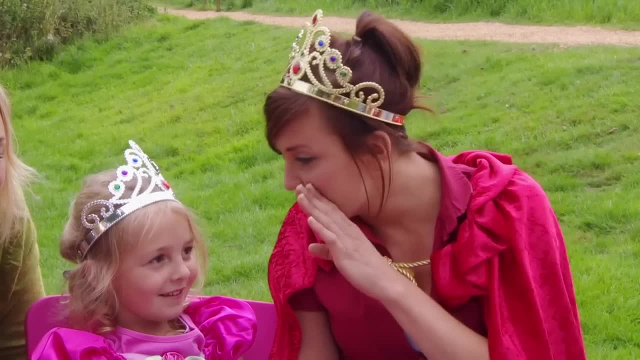 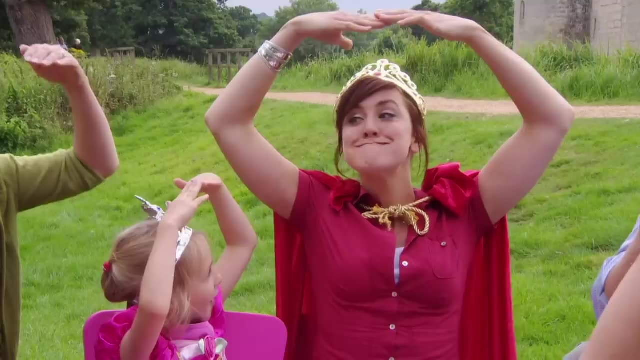 The mushroom face. The mushroom face. Shall we show the mums and dads how to do the mushroom face. What Do you remember? This is the mushroom face. You put your arms on your head and then you go like this: Look at your mum, Anya. 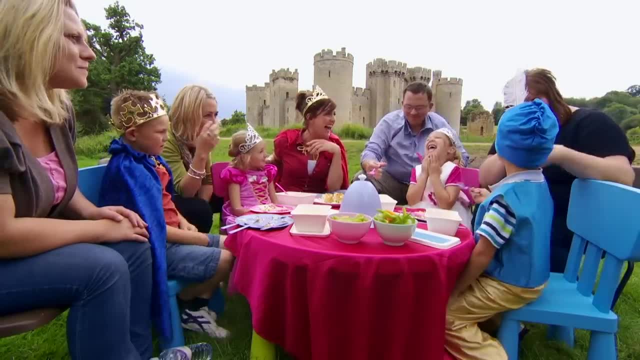 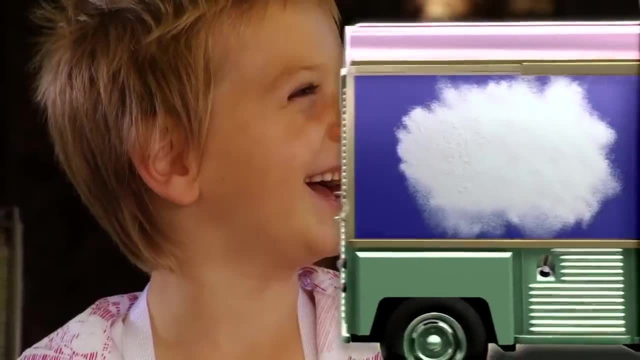 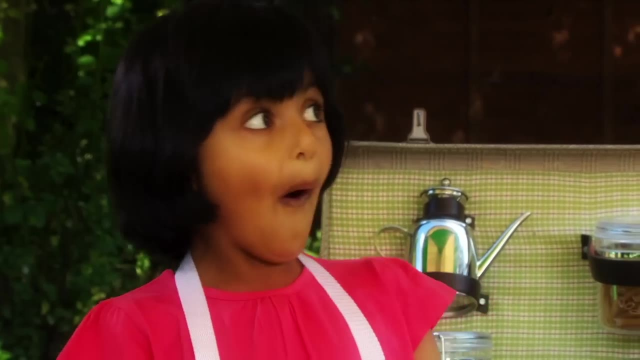 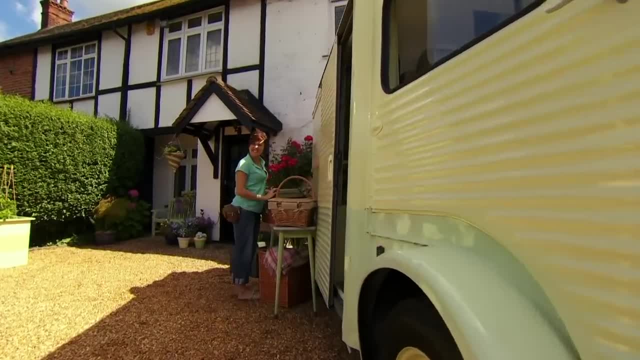 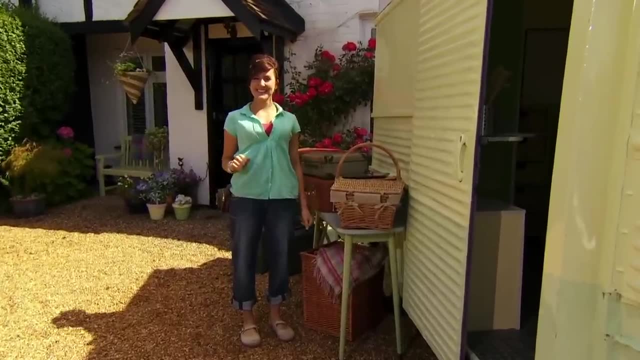 I can cook. I can cook With you. Hello, Oh, good to see you. I'm just getting everything ready to go on a journey and I hope that you're going to come with me and make some new friends. Ah ha. 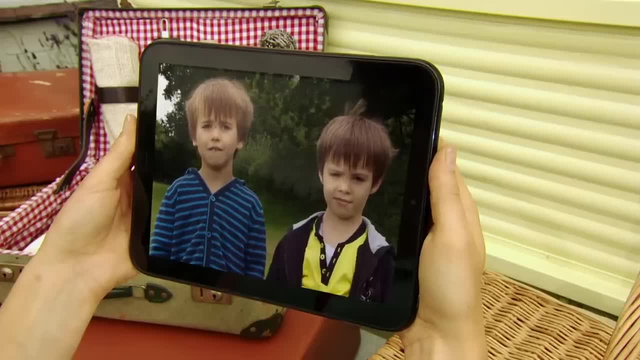 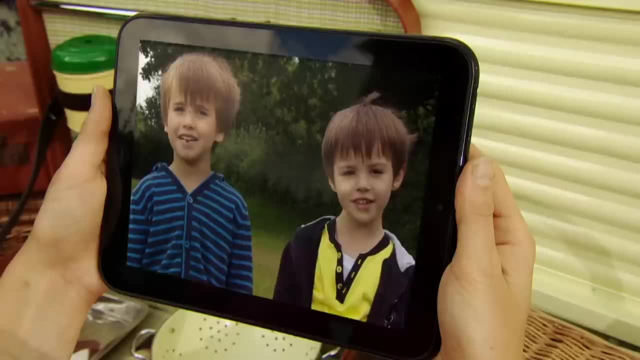 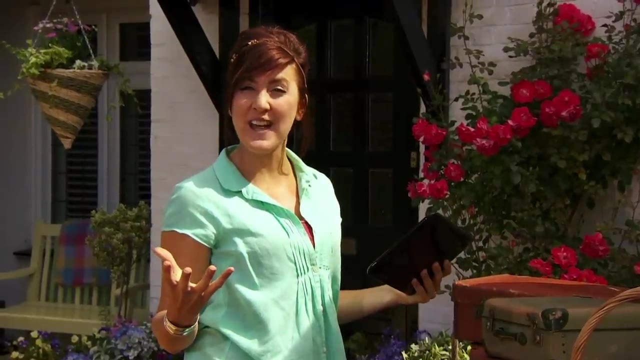 Hello, Katie. we love to make something to eat on the steam train and we love cakes. How exciting is that. Katie, can you cook with us please? I certainly can, and I would love to go for a ride on a steam train and you can cook with me too. 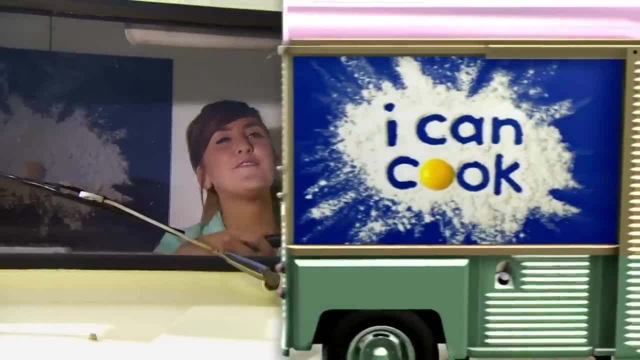 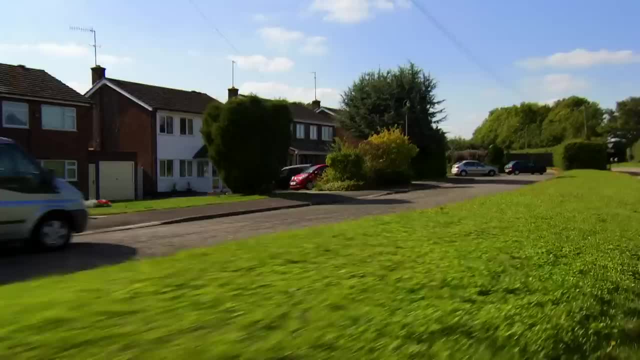 So let's pack up and go Off on a journey- and I'm coming to you. It's going to be busy and there's lots to do. Get ready to help John in and have fun. Let's cook a feast for everyone. 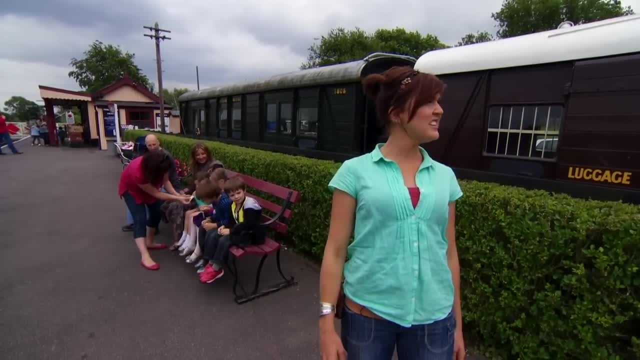 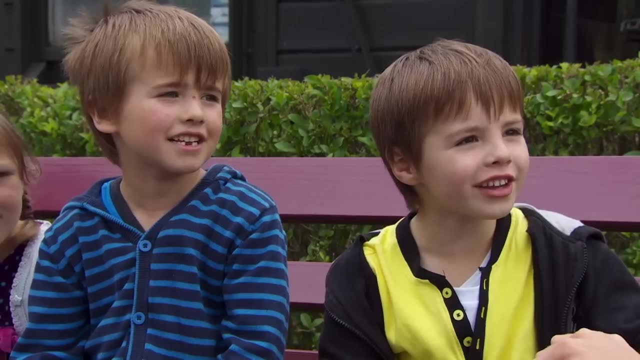 Wow, what an amazing old railway station. But I wonder where Ollie and George are. There they are look. Hi, George and Ollie. Hello, Katie, Are these all your friends and family? Yeah, Hello everyone. Hello. 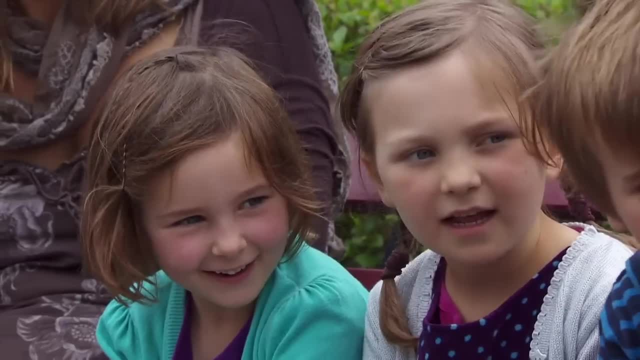 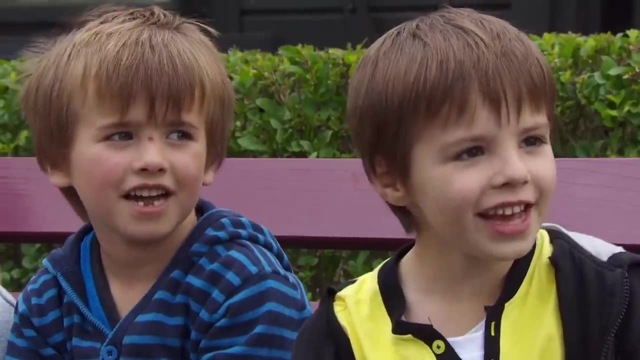 So what's your name, Natasha, And what's your name, Lisa? Oh, it's brilliant to meet you all. Now, boys, I'm so excited. Are we actually going to go on a steam train? Yes, and we're going to have a picnic there. 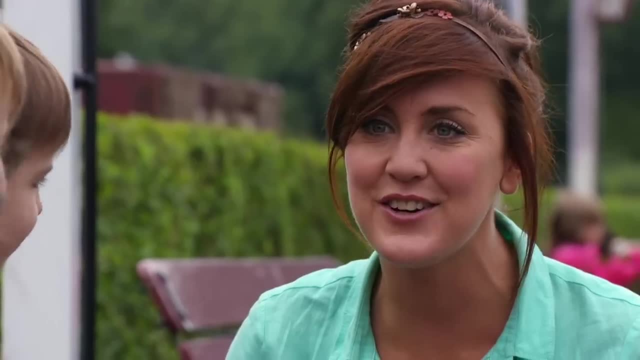 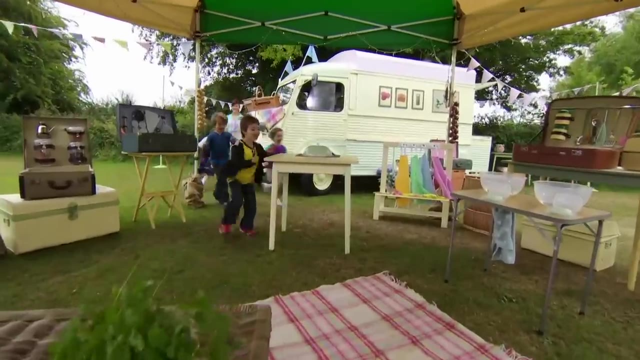 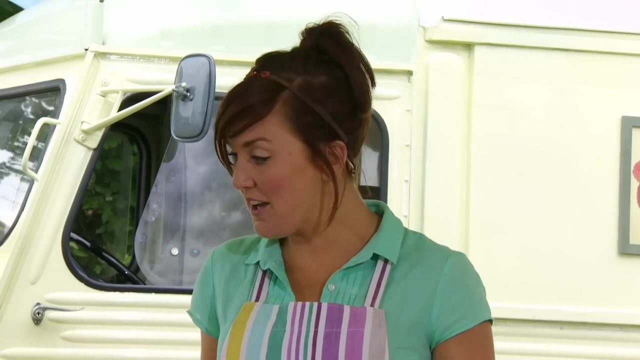 Oh, that's brilliant. I have got such a fantastic recipe for us to cook together. Come on, follow me and I'll show you Welcome to my outdoor kitchen. Who's ready to do some cooking Me? Do you want to see what we're going to cook today? 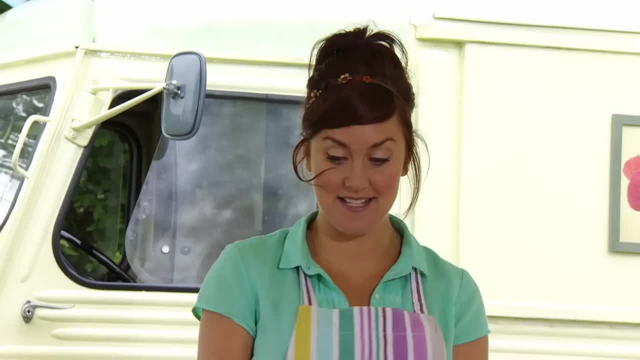 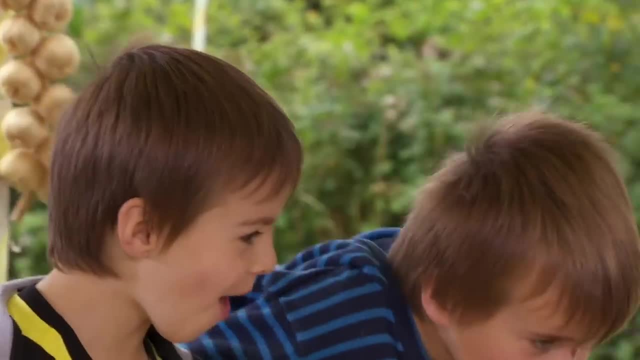 Yeah, Ok, ok, ok, I'll show you. It's under here. Today's recipe is spiced fun buns. Yes, Oh, they smell good, Mmm. But before we cook them, we've got to do something really important. 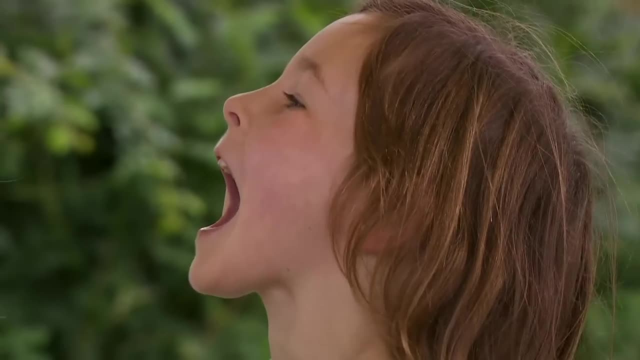 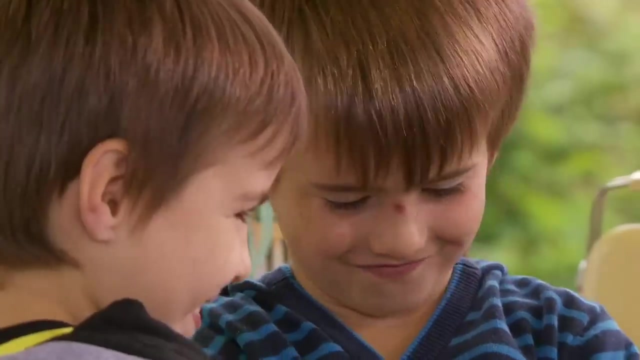 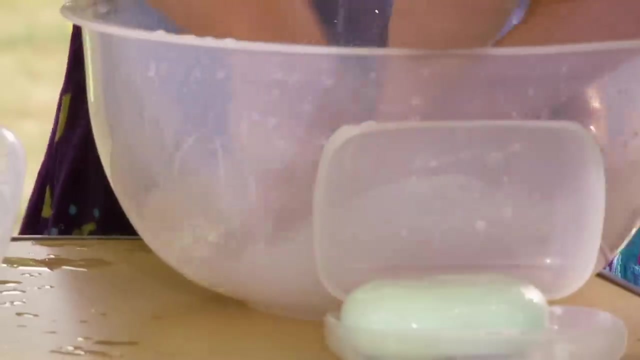 Do you know what it is? Wash our hands. That's right, we've got to wash our hands. Come on, team Music, Roll up your sleeves, Give your hands a wash With flippy dippy soap. Splish, splash, blosh. 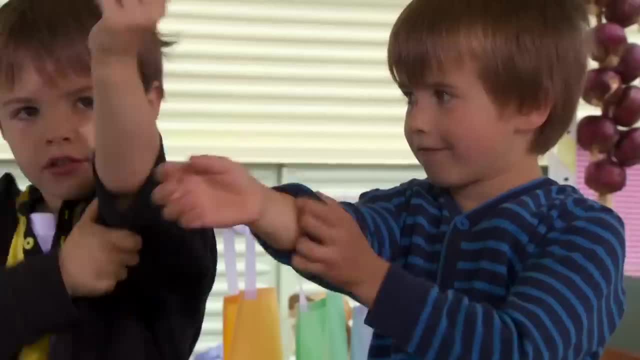 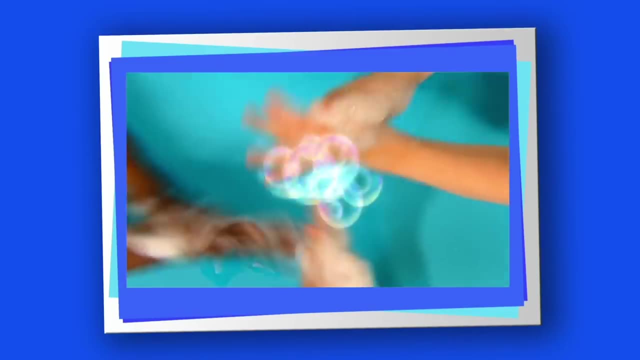 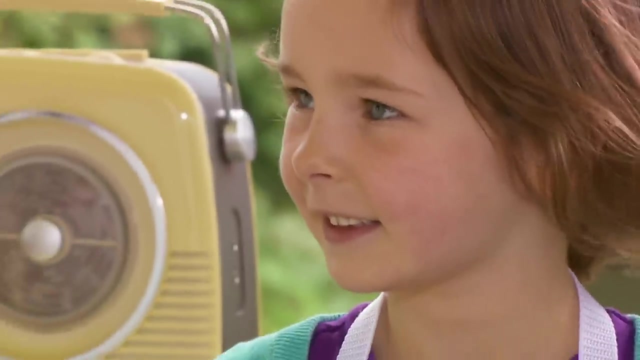 Have you done? your hands Washed and dried, Sleeves rolled up, Apron tied. What can you do? I can cook, Right. let's get started Now. to make our spiced fun buns, we are going to need three spoonfuls of currants, two spoonfuls. 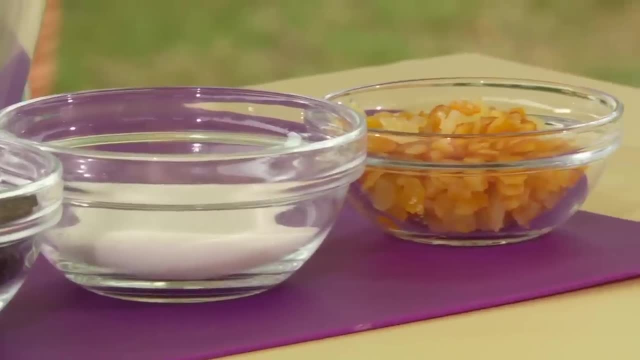 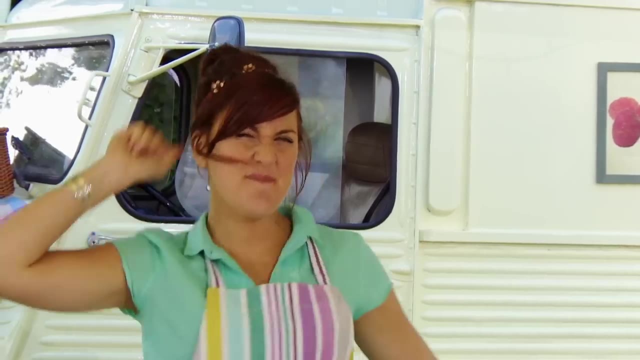 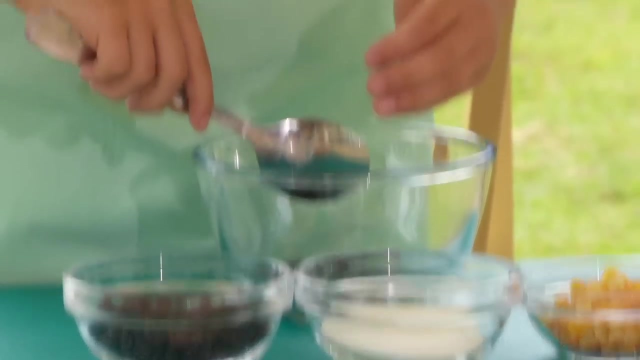 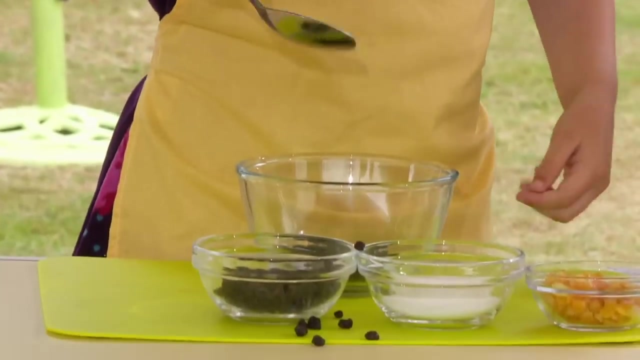 of cast sugar and one spoonful of fruit peel. So that is three, two, one blast off. Ok, let's get measuring. then. One, two, three, Yep, Two, three, One, two. Ok, let's get one spoonful. 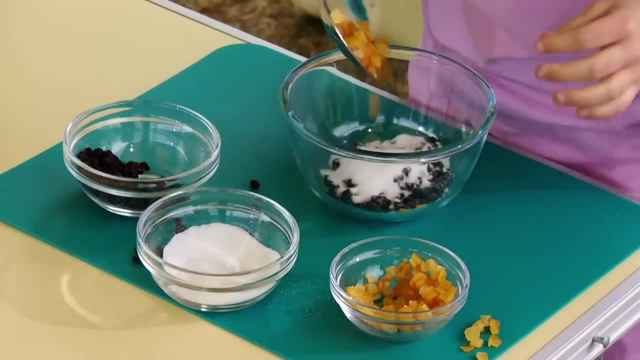 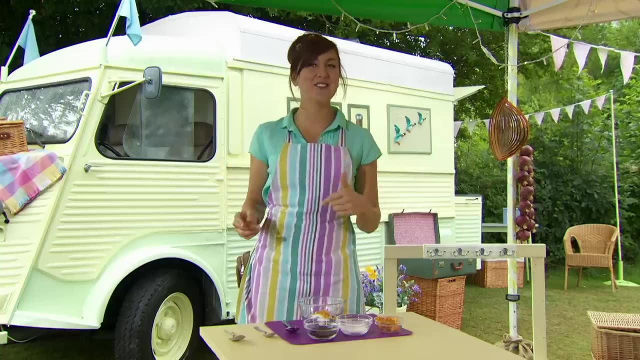 Two spoonfuls of fruit peel. There we go. One Finished Right now we've got everything in our bowl. we're going to give it all a really good mix, And you can join in with the mixing at home too. 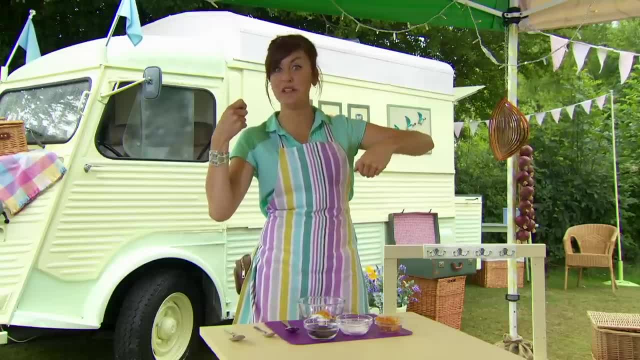 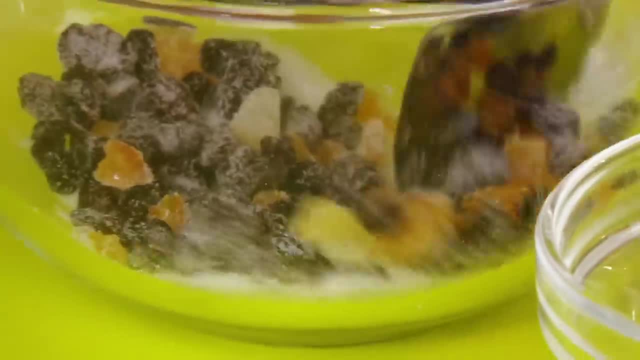 Just get your bowl and then get your spoon, Mr Spoon, and give everything a really good mix like this: Mix, mix, mix. There we go. Ok, let's call this our fruity bowl, And for the fruity bowl, we're going to do the fruity bowl. 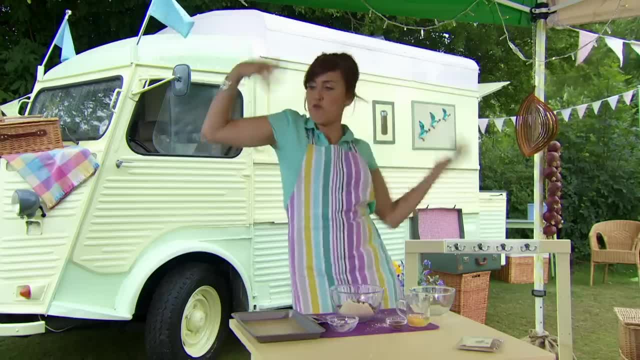 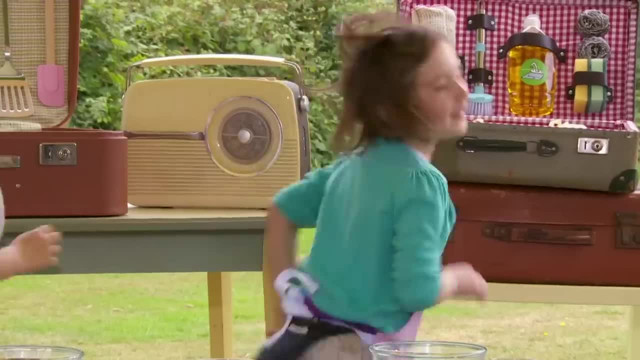 the fruity dance. Who can do the fruity dance like this: Frutty, frutty, frutty, frutty, frutty. Can you do the fruity dance with us? Frutty, frutty, frutty, frutty, frutty, frutty. 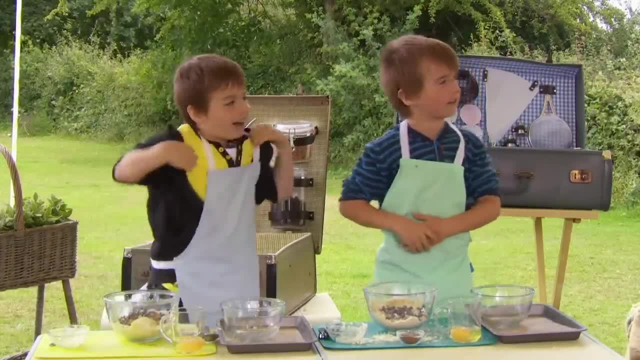 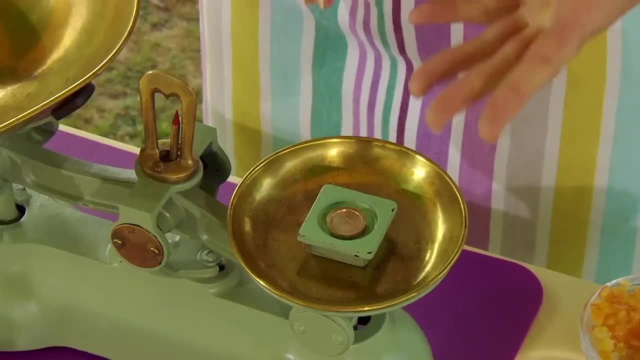 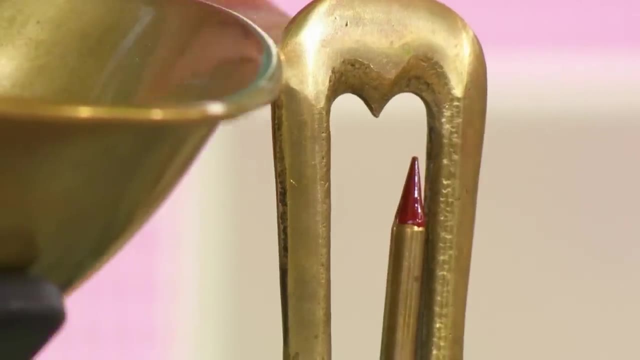 Everyone say frutty. Next we're going to do some more measuring, but this time we get to play with the scales and it's really fun. This weight here weighs as much as the flour that we need, which we're going to put on the other side. So when this little red pointy 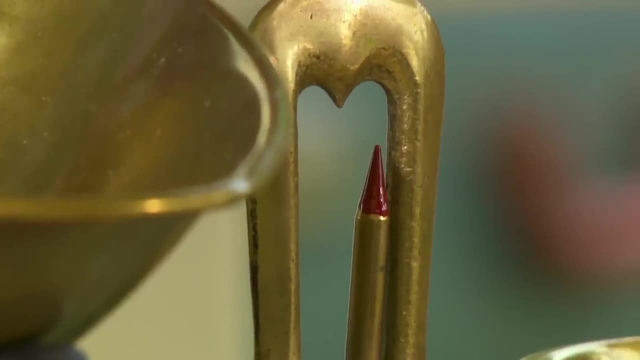 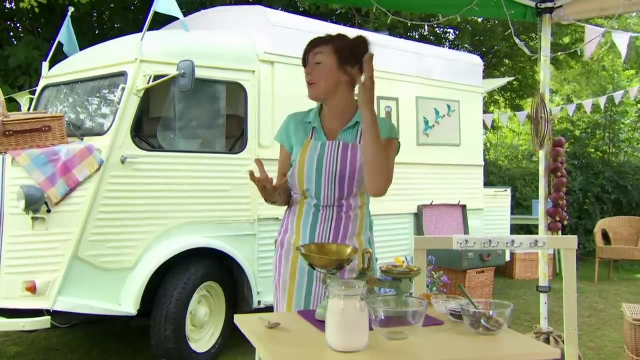 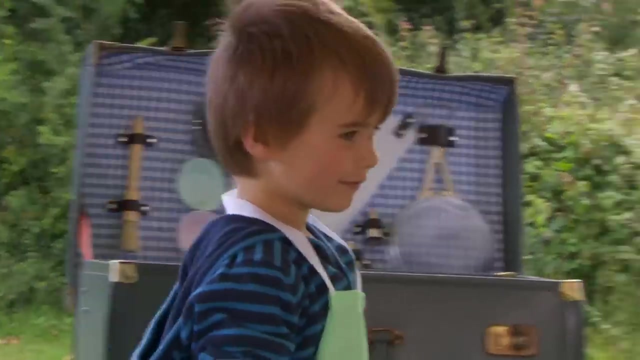 thing points to the middle, that's when the two sides are balanced. What I need you to do in the weighing game is shout out. if we need more, Can you shout more, More. Let's hear you say less, Less, Brilliant. We're ready to play the weighing game, George, you. 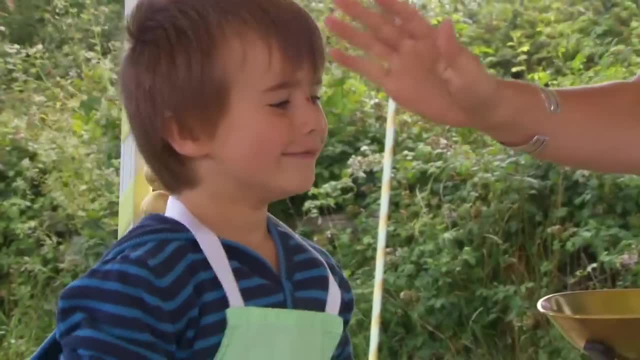 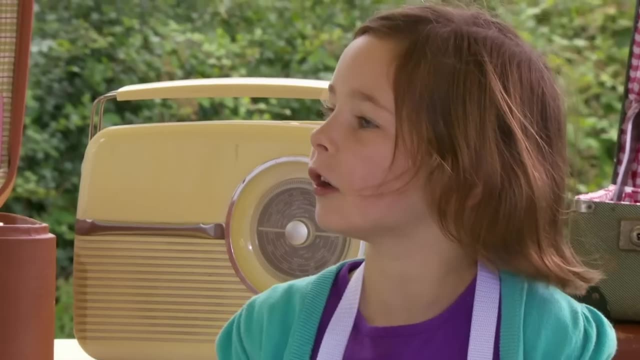 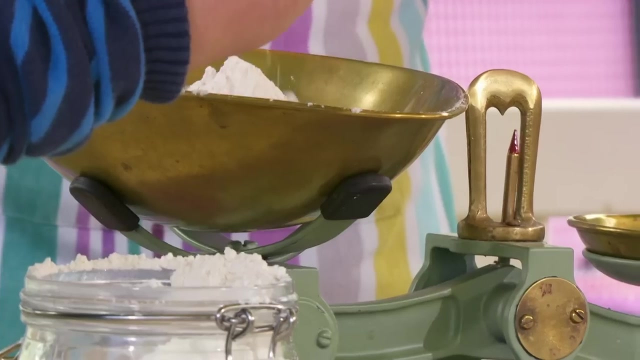 can do the measuring and everyone. remember we're going to shout if we need more or less, and don't forget to join in with us at home. Okay, there we go. More Do we need more or less? More, Oh Less, Take some out, Oh Yes. 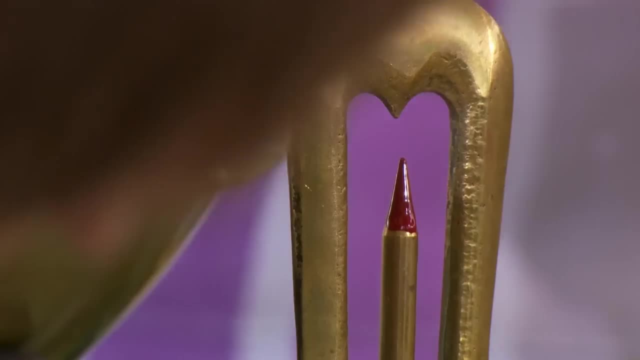 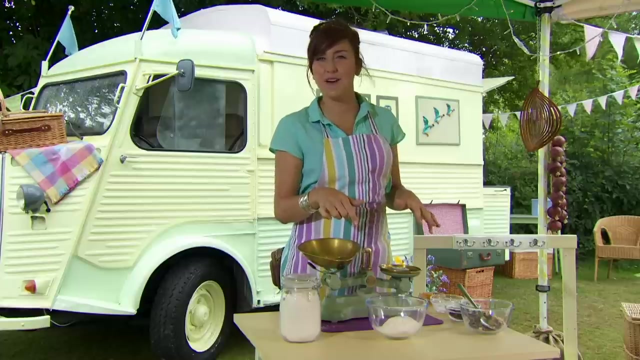 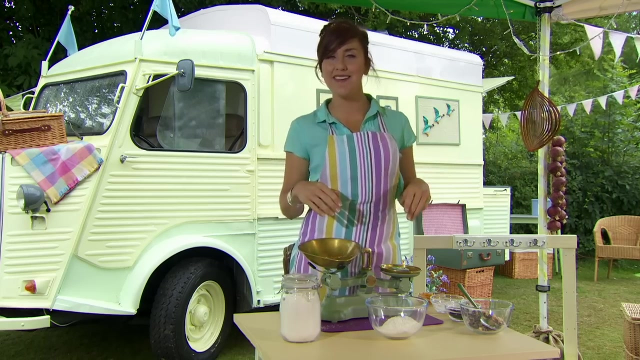 It's in the middle. you did it, George, Good job. Thanks for your help, everyone. Now, what ingredient do you think we're going to need next in our Spiced Fun Buns? What is next? Well, let us see. Let's see if you can guess what it could be. So we've got some raspberries, a loaf. 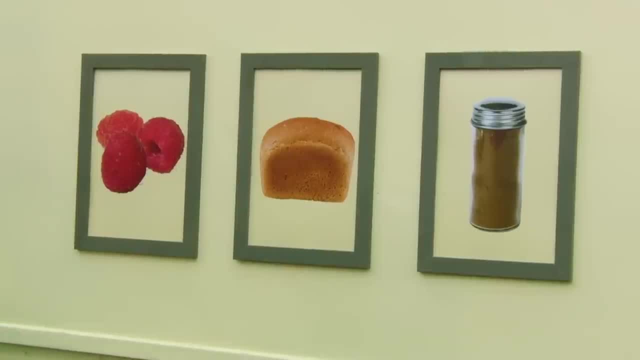 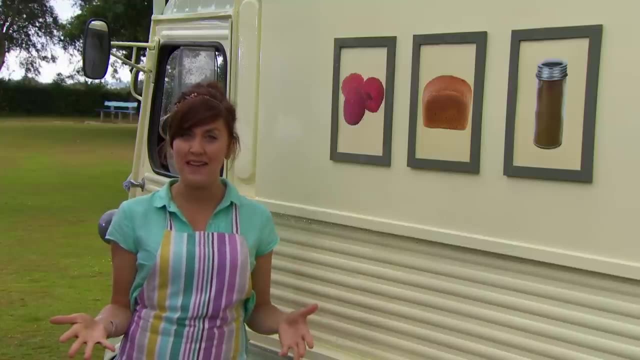 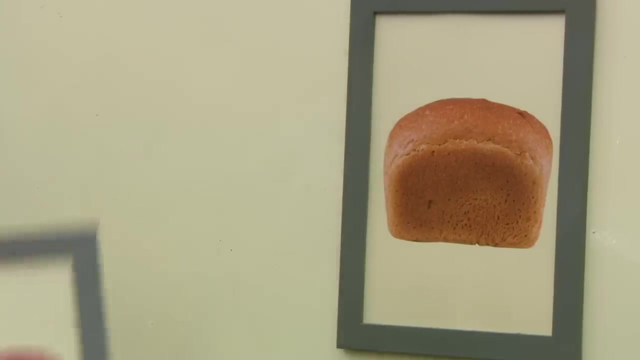 of brown bread and some mixed spice. What would you choose for our Spiced Fun Buns? I know I'll give you some clues and you can try and guess what you think it might be. The special ingredient is brown. Well, raspberries are red, so we can take that one away, Okay. 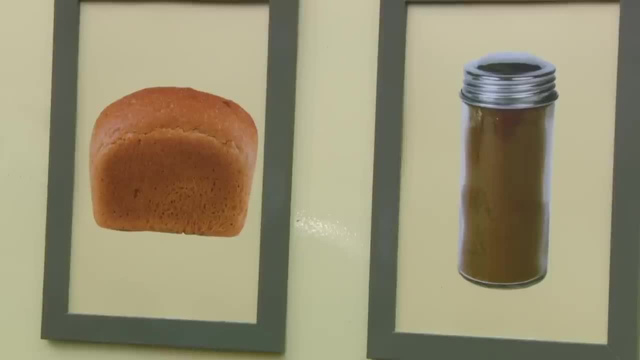 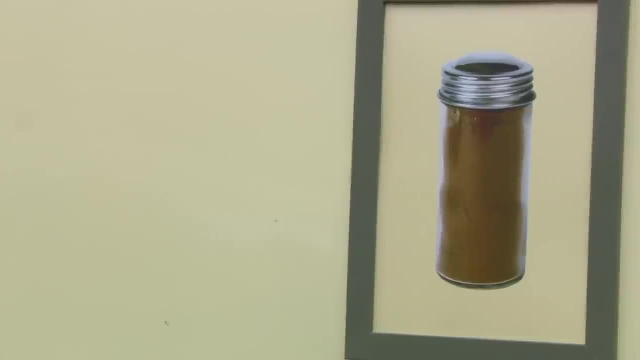 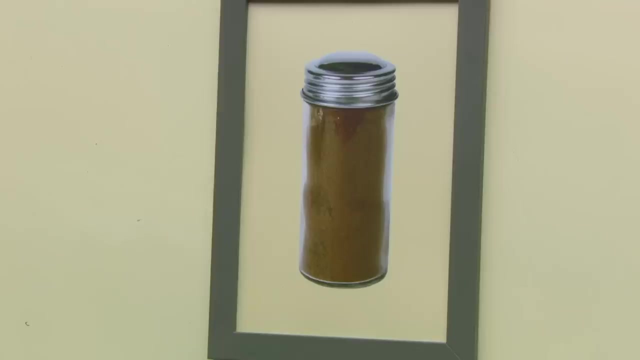 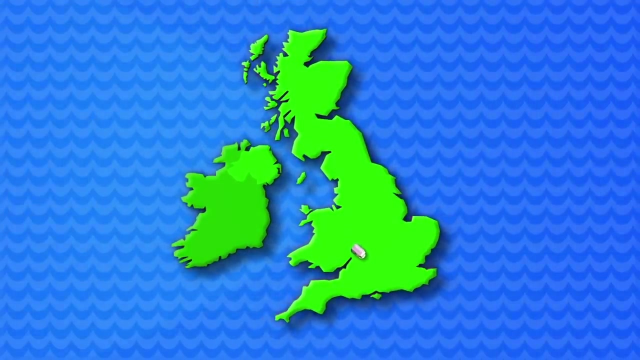 here's another clue, And it's a powder. Well, brown bread isn't a powder, is it? So we can take that one away too. There you go, Which leaves us with mixed spice. We're going to need some mixed spice in our Spiced Fun Buns, and I went to find some. 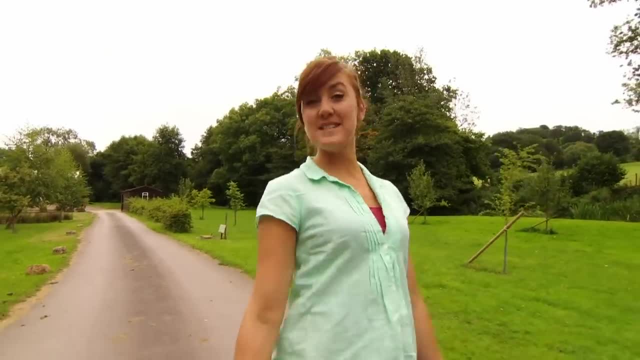 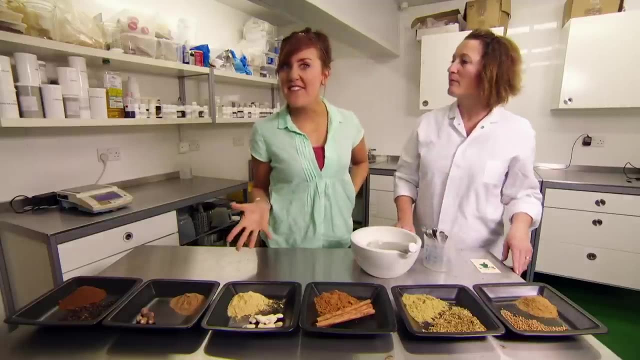 I've come to Alderley in Gloucestershire to find out what goes into mixed spice. Come on, let's go and have a look. I'm here with my friend, I'm here with Becky, who's a flavourist, and Becky's going to tell me what different. 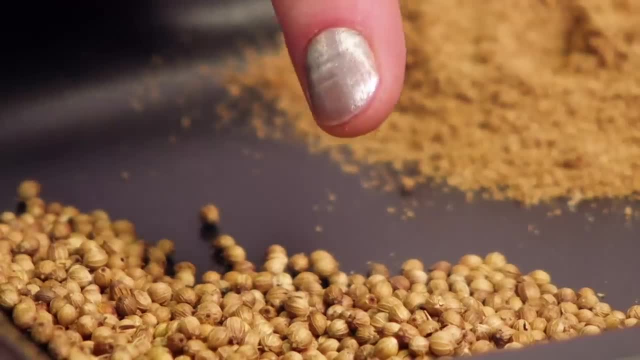 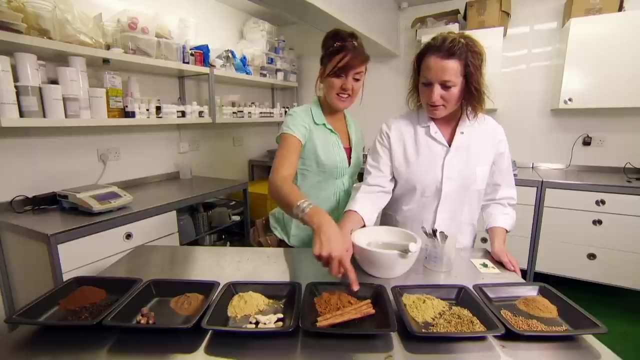 spices are in mixed spice. This is coriander and this is from India. Okay, We also have fennel, which comes from India, This is cinnamon and this comes from China. They're like little wooden sticks. The ginger comes from Africa. 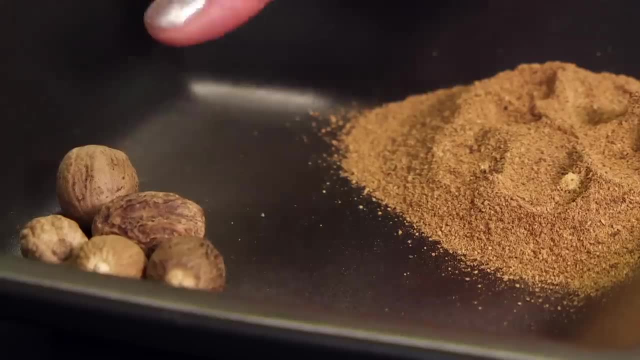 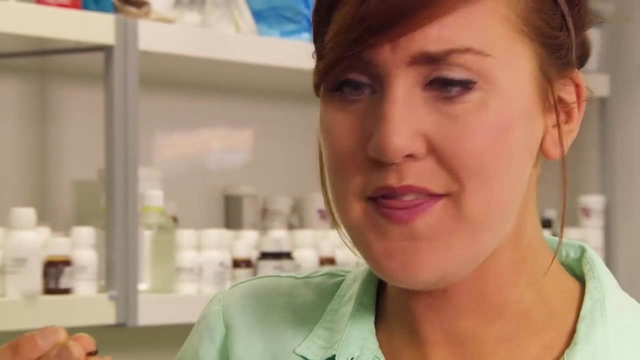 Oh my gosh, they look so funny. Look, it's like white seaweed, This is nutmeg and it comes from the Caribbean, and we have cloves that come from Indonesia. Wow, they smell really good, Really strong. Actually, they smell a bit like Christmas. 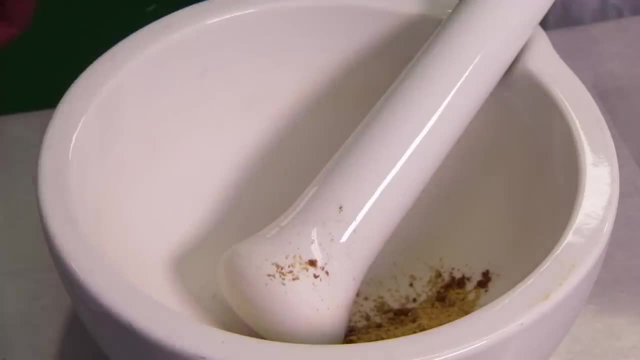 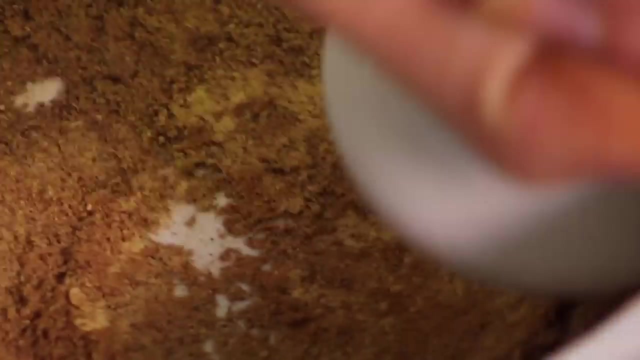 And now we just need to use this, which is called a pestle and mortar. All of these ingredients are ground up. Wow, look at all the colours mixing together And there we have it: a lovely mixed spice. Should we put it in the bag now, Becky? 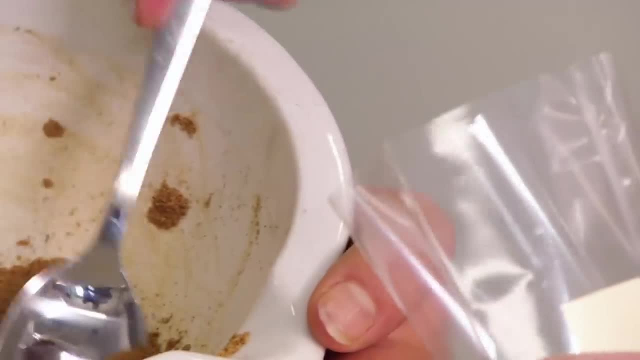 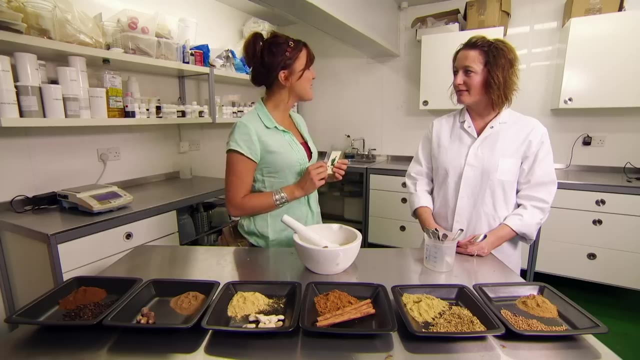 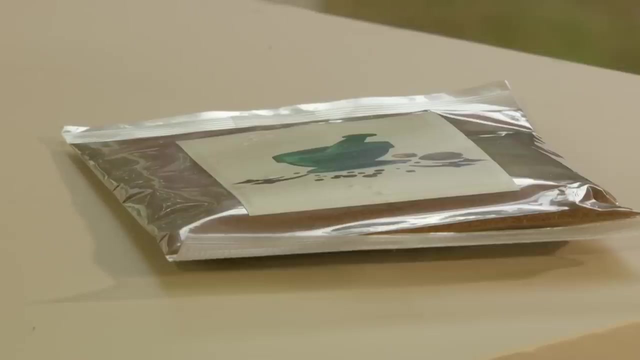 We can. Smells absolutely fantastic. Great, This mixed spice is going to taste delicious in our Spiced Fun Buns. Okay, Spiced Fun Buns. Thank you very much, Becky. Thank you, Bye, Bye, Katie. Those spices smelt amazing. So let's take a pinch of mixed spice and then sprinkle it. 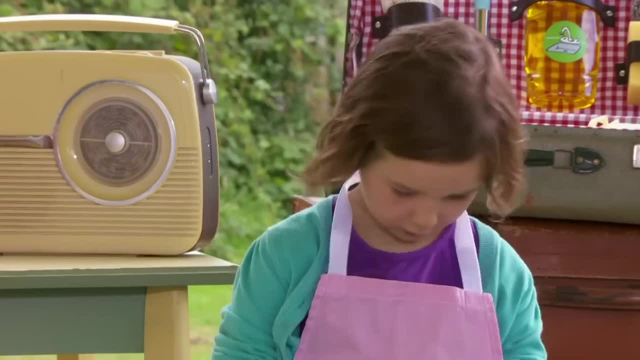 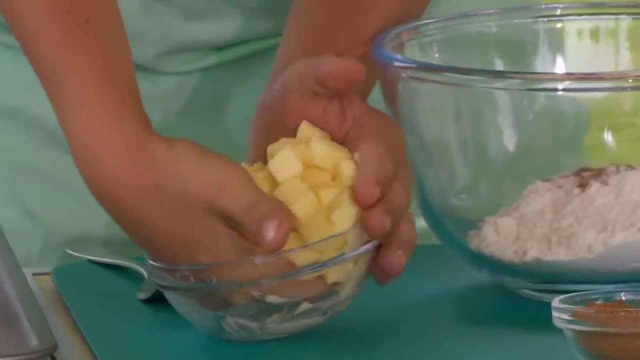 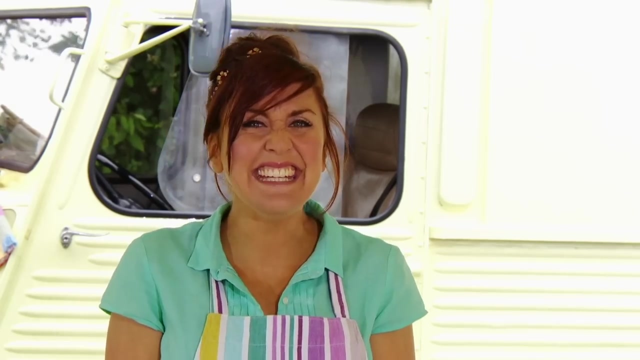 into this bowl with the flour in it. That's it. Bring your flour bowl into the middle of your mat, because next we're going to use some butter. Scoop the butter out of the bowl. Oh, it's all sticky. Now this is how you do tickling. First of all, you need your tickle. 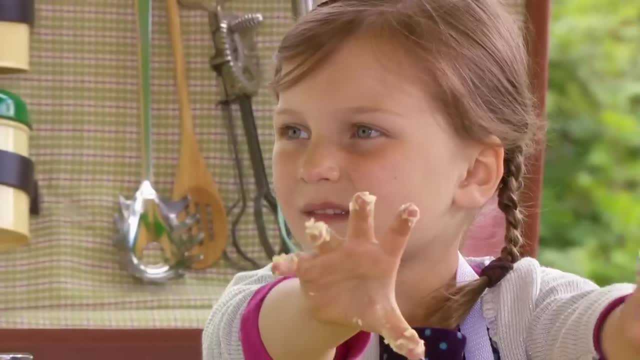 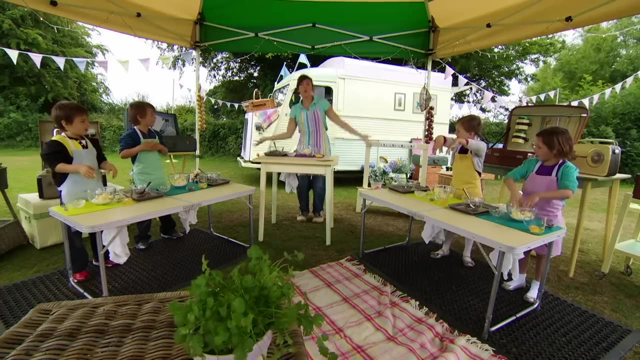 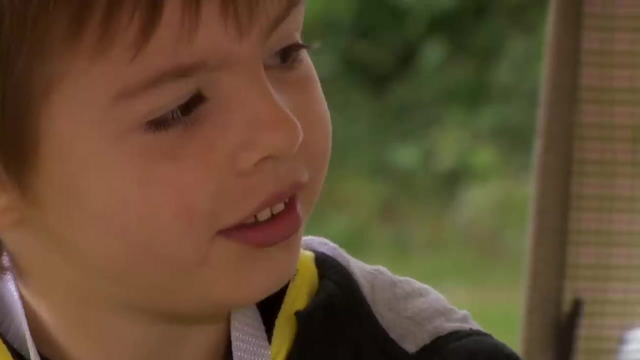 fingers. So put your fingers like this and go tickle, tickle, tickle, That's it, And we put our tickle fingers into the bowl. So we dive in like this, Whoa, And get right down to the bottom and give everything a good squeeze, Squeeze, really, really hard with. 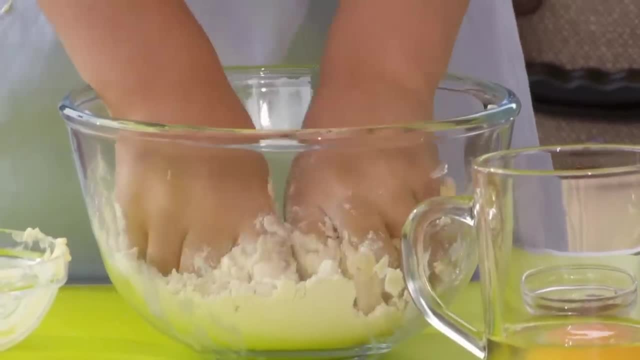 your fingers, Okay, And then rub the butter and the flour in the mixed spice together with your finger tips. It's all slimy, Everyone go. tickle, tickle, tickle, Tickle, tickle, tickle, tickle. 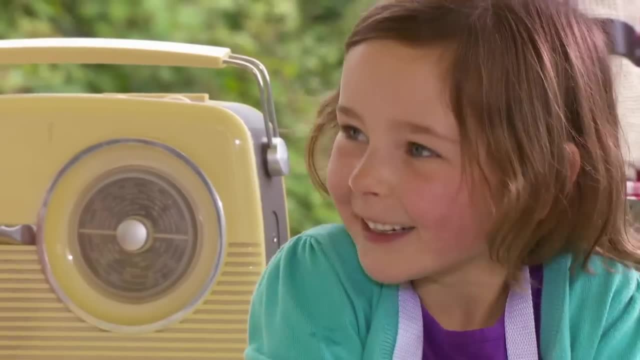 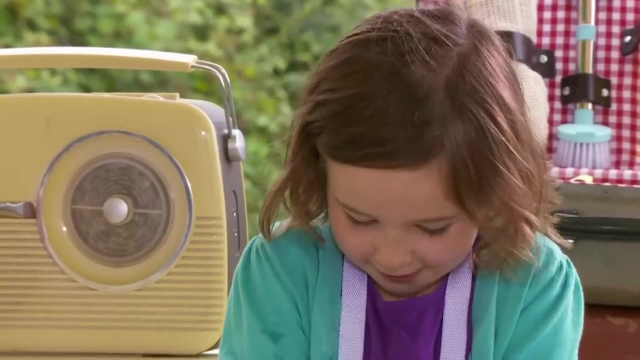 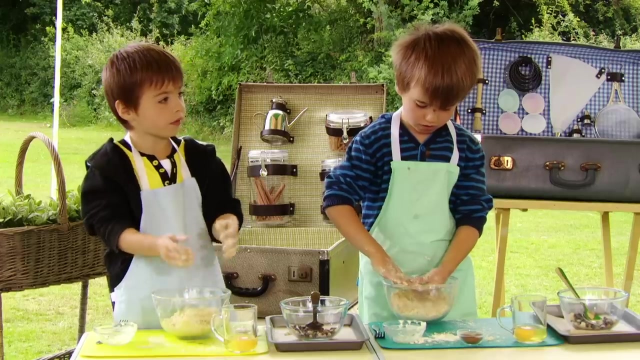 Oh my goodness, Look at my hands. Look at my hands. We look like monsters. Who has got monster hands? Yeah, Hold your hands out in front of you like this. This is really fun. I love this part: Ready Go. 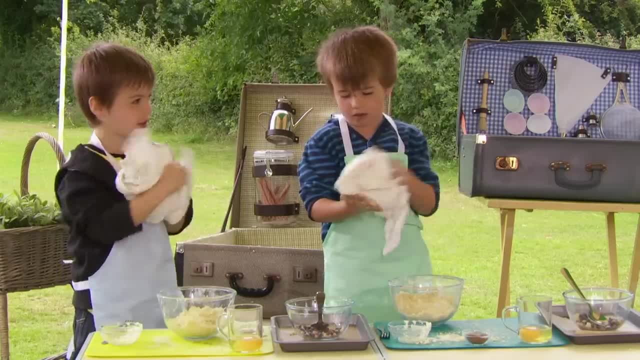 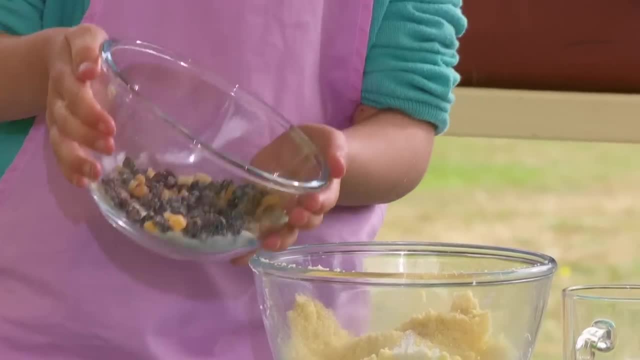 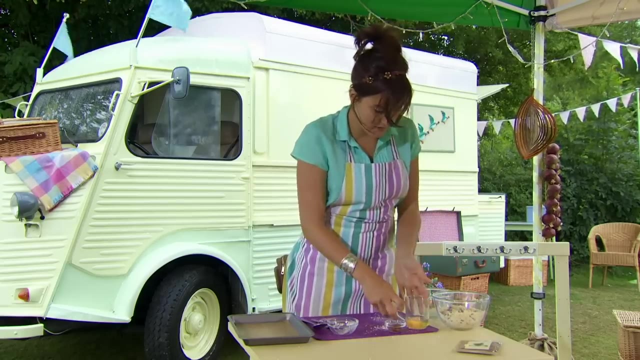 And then give your hands a wipe quickly. Next, we're going to add our fruity mixture into our crumbly mixture. One, two, three, Whoosh, Whoosh. Let's put this bowl to the side for a minute, because now we need to bring over this cup. 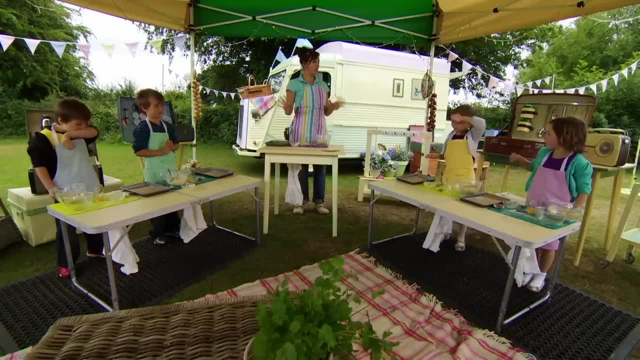 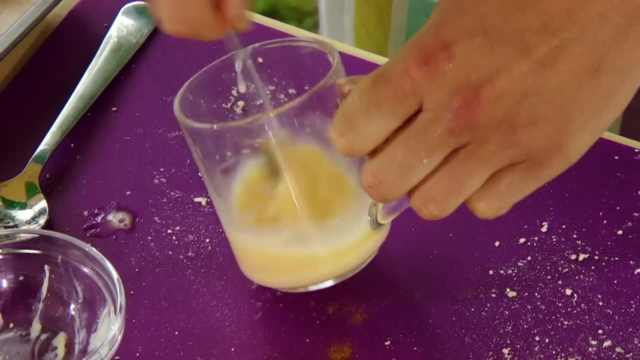 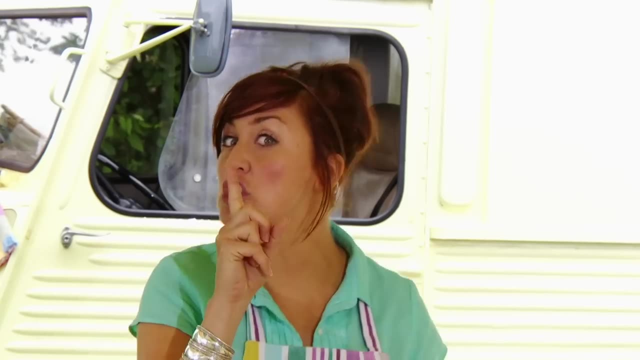 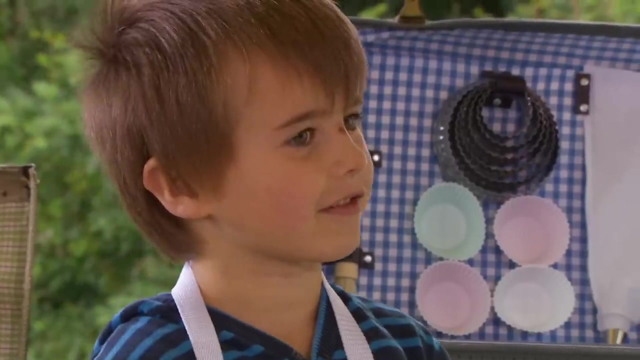 which has an egg that I've already cracked for you And we are going to whisk it up. Let's get whisking. This is fun, Great. Now the next part of the recipe is a secret. Everyone go shhhh. Now the secret is that we use some, but not all, of the eggy mixture. Can you say that? 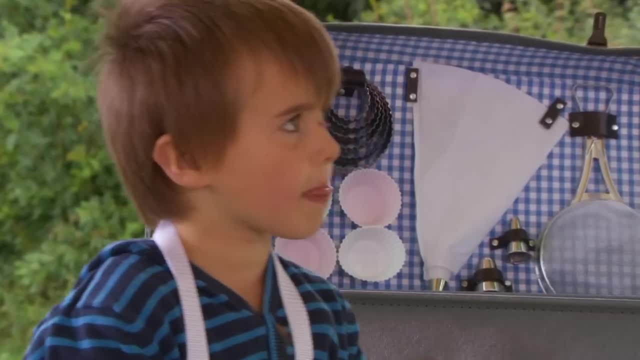 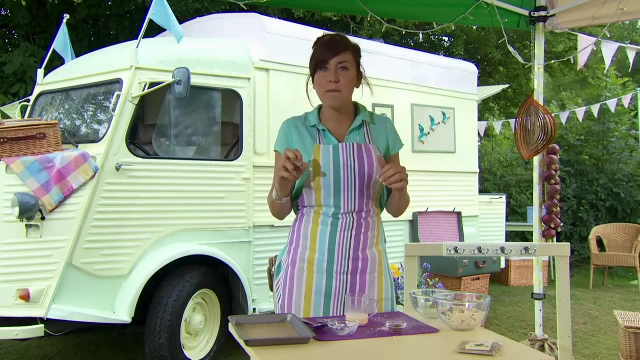 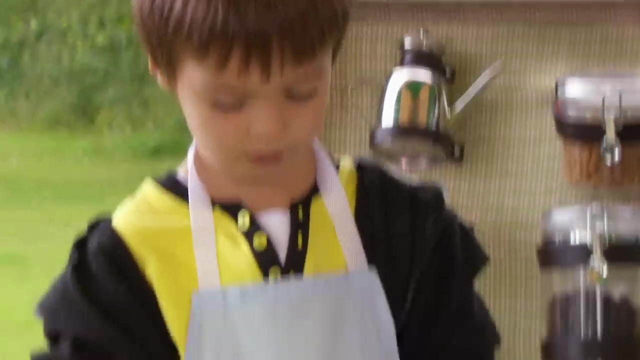 Some, but not all. That's it OK. Do you know why? Why? Because that is what's going to make our spiced fun buns really crumbly, Really crumbly and bumpy, Really delicious. So bring back your mixture Ready. 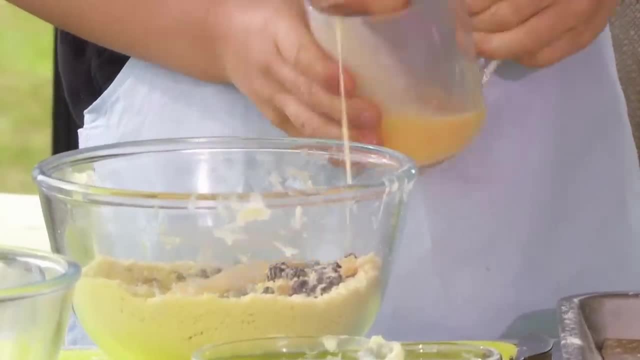 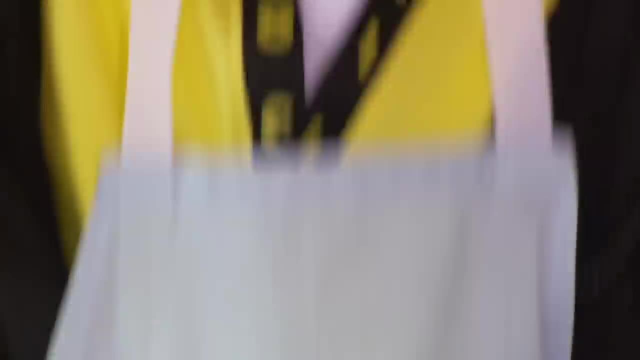 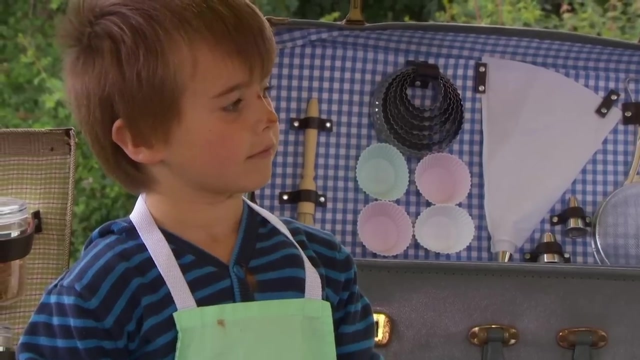 Pour And stop, And then use your fork to mix it all up. So let's get mixing team. The next thing we have to do is get really messy. Are you ready to get messy? Yay, I thought so. OK, Take your fork out of your bowl and just put it on the side. 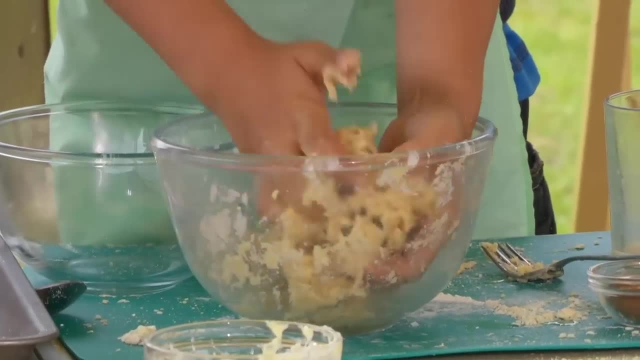 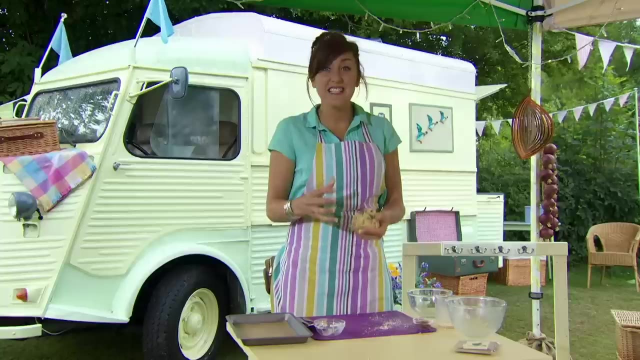 And then get your fingers right into the bowl and into the mixture and make it into a big ball. Now we are going to make this one ball into eight spiced fun buns, and I'll show you how. First of all, we split this one into two pieces. 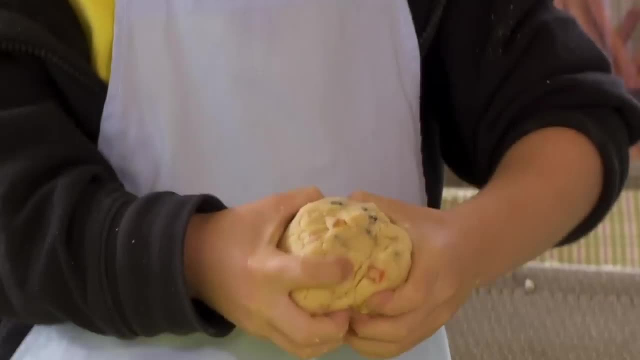 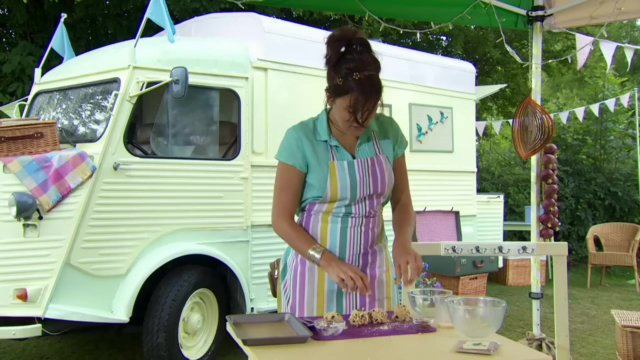 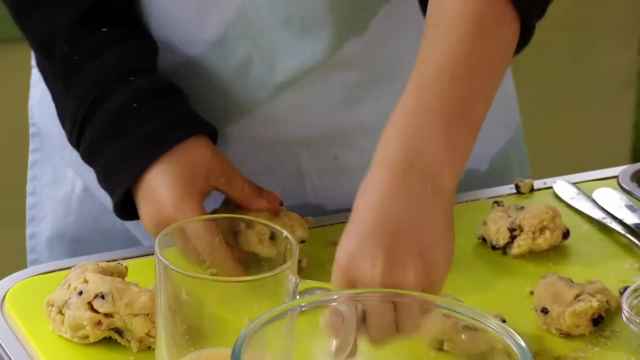 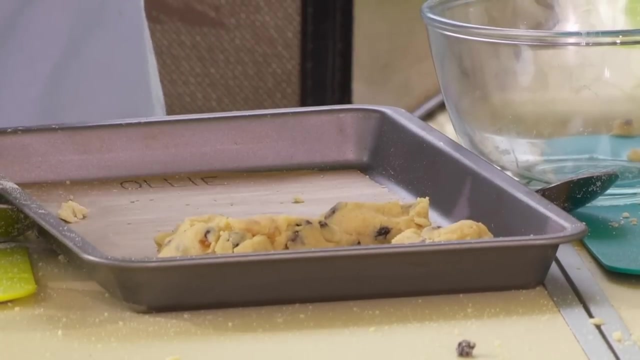 There we go, Put that on the mat, And then we split both of these two into two, And then we split each one of these into another two pieces. My fingers are so sticky. So now we've got eight, And once you've made eight you can put them onto your baking tray in two lines. 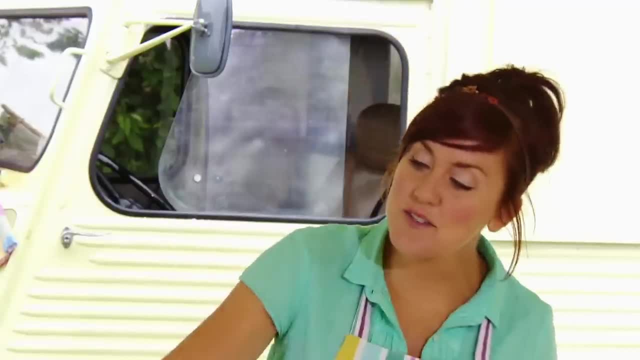 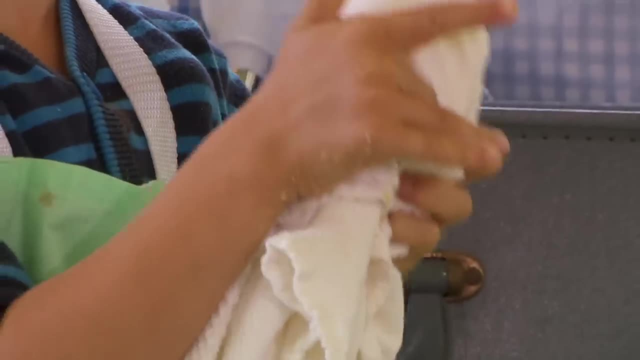 I don't know. Yes, I do. There we go, Ollie, yours are brilliant. They look like fluffy clouds with little black spots, And that is it. You did it. You put all the ingredients together for your spiced fun buns. 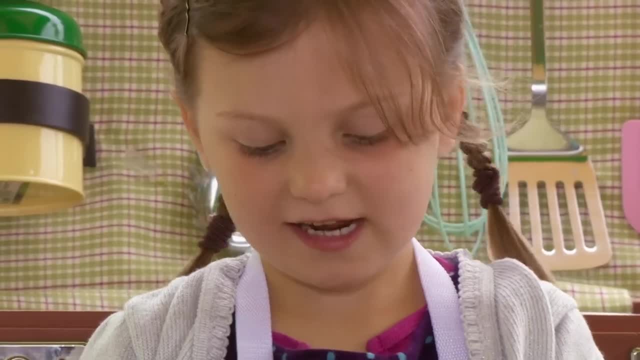 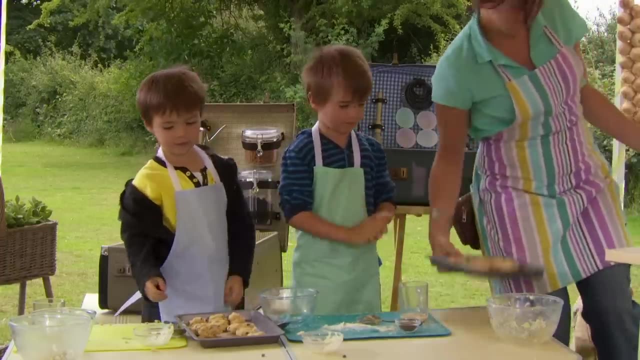 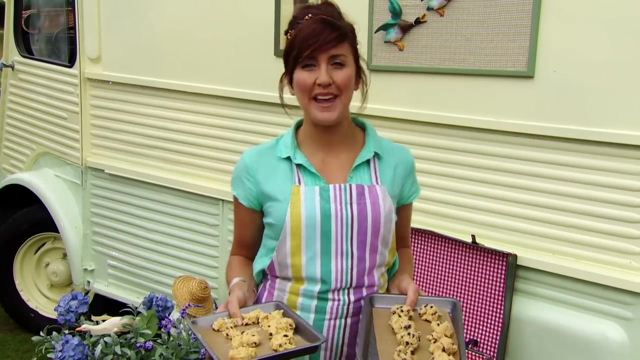 All by yourself. Well done. Everyone say yeah, Yeah, And now I'm going to put them in the oven for you. There we go, But remember, ovens are hot, so don't go near. Ask a grown up to help you here. 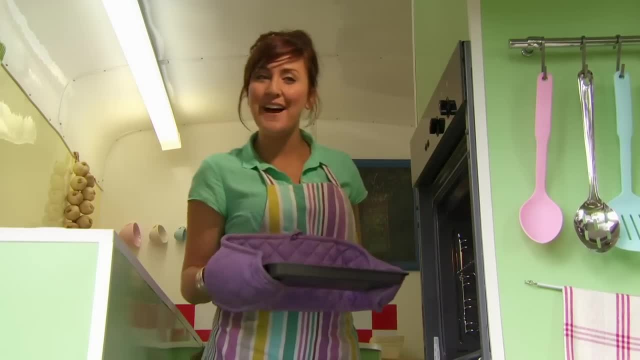 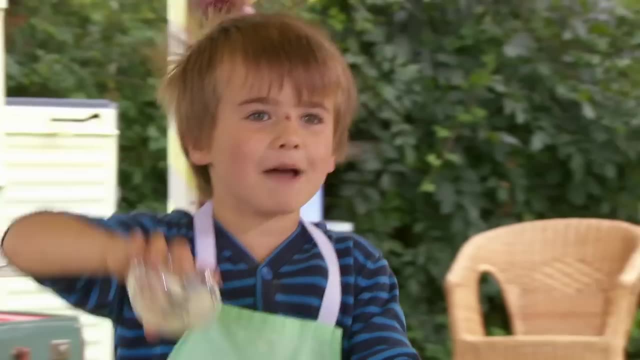 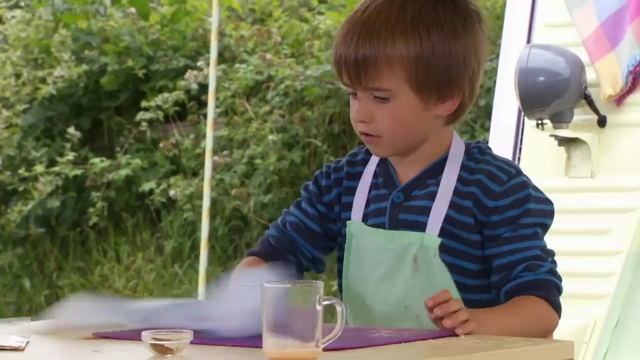 Now. we've cooked with you and had lots of fun. Let's tidy up and think of all the things that we have done. There was Cooking, Sizzling Memories, Whisking. Clearing any mess and putting things away is always fun to do at the end of the day, 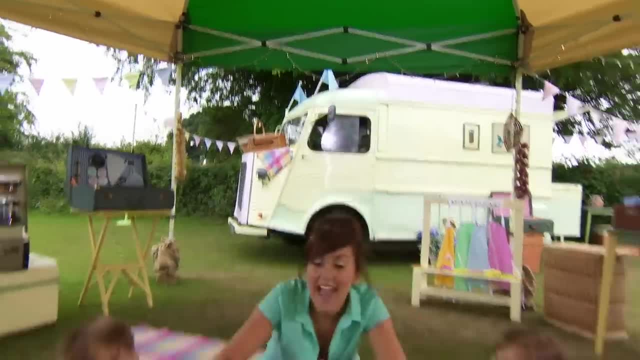 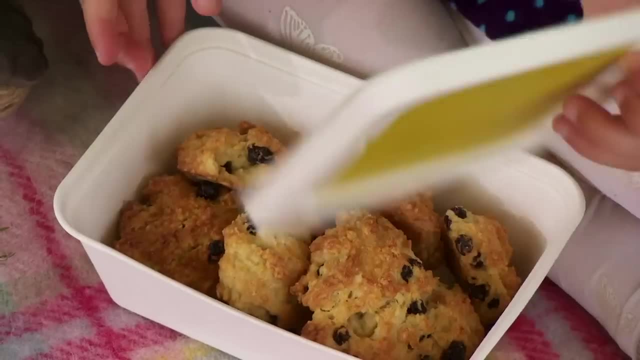 And here are your spiced fun buns, and they're all cooked and they smell so delicious. There's yours, George, Natasha, let's have a look at your ones. They're good, aren't they? Yes, Can I have a smell? Oh my goodness. 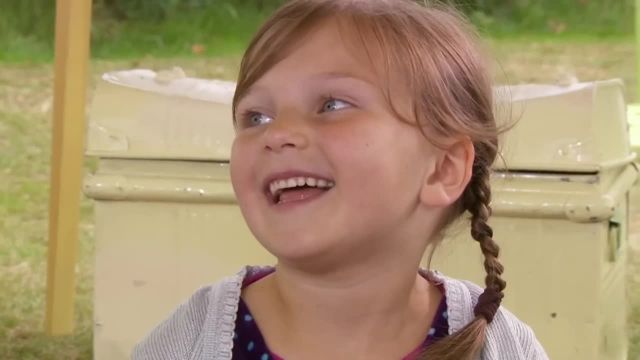 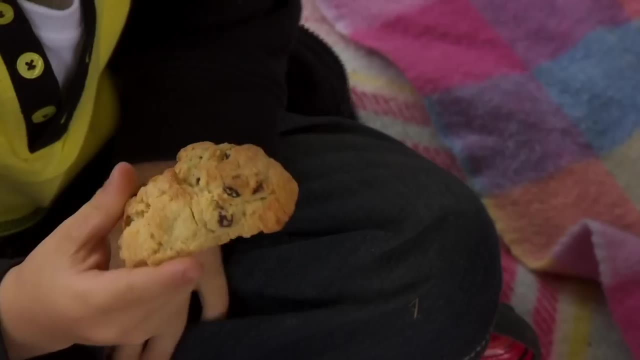 They smell delicious. I can't wait to get them later on. Okay, let's have a look at yours, Ollie. Hey, what do you think of yours? Good, Why don't you pick one up and see what shape it's turned into? 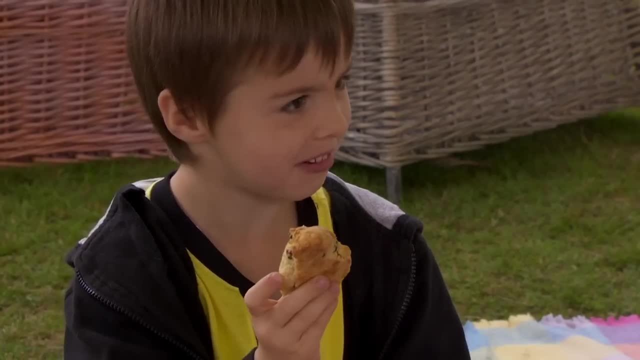 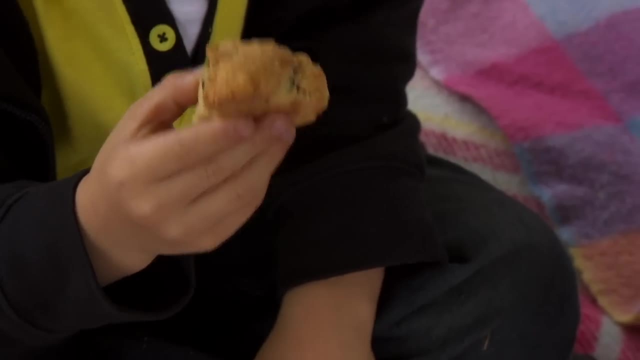 This one, I think, turned into a pig head, Because look, there's a nose and then the head. I think it looks like a rocky mountain. Right, let's put the lids on and save the rest for later on. We've travelled to you, we've cooked and had fun. 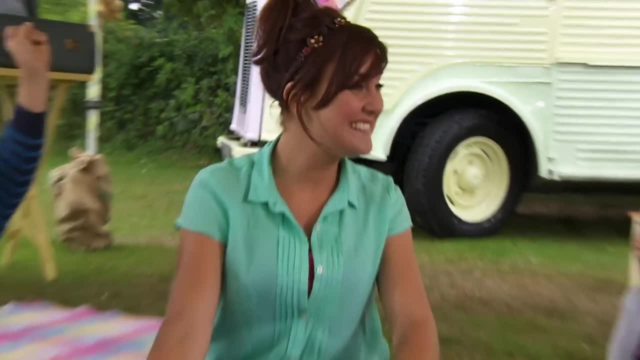 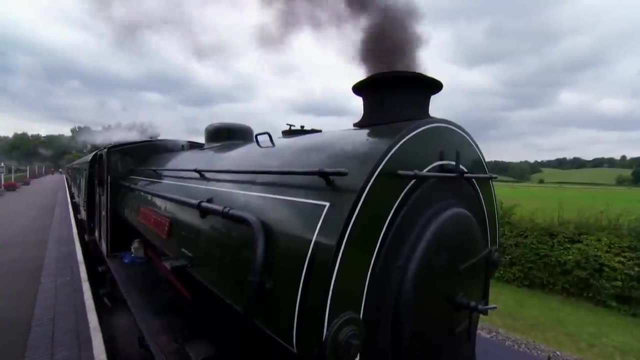 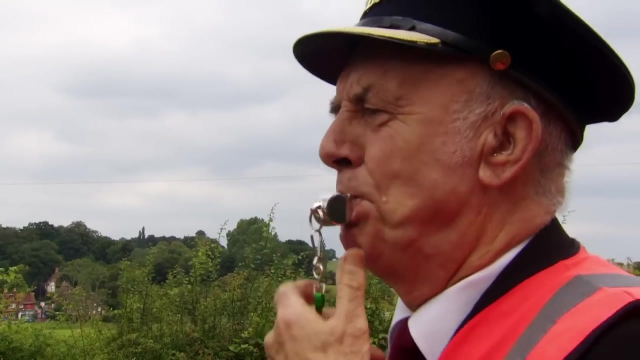 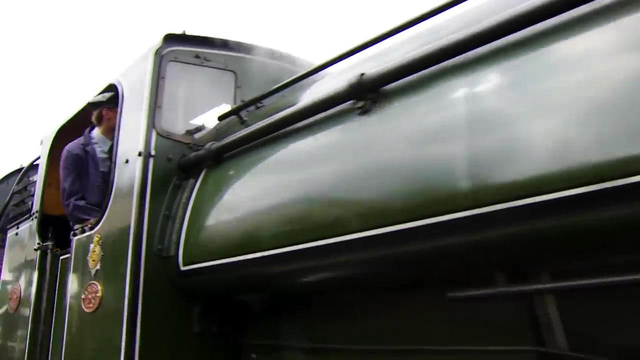 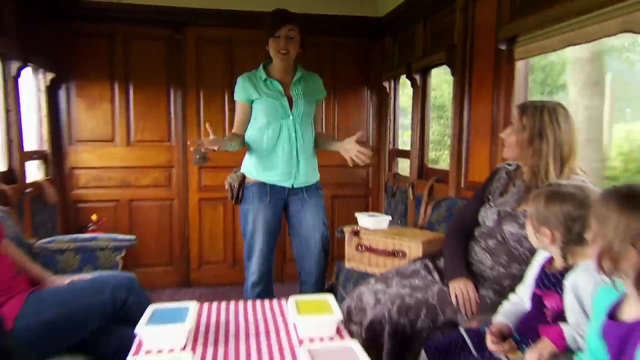 Now let's have a party. We're going to have a party with everyone. Yeah, Come on, follow me everyone, and you can come too. Well, here we are on the steam train, and it is so exciting. I've never been on a steam. 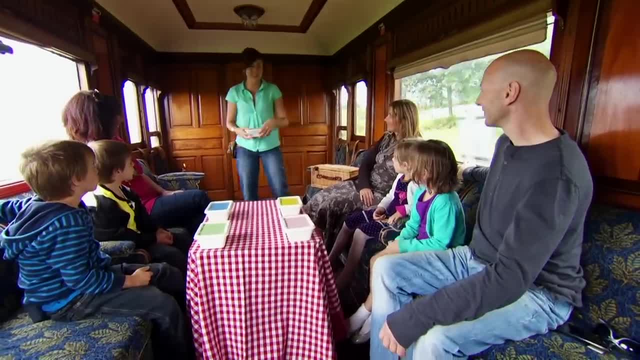 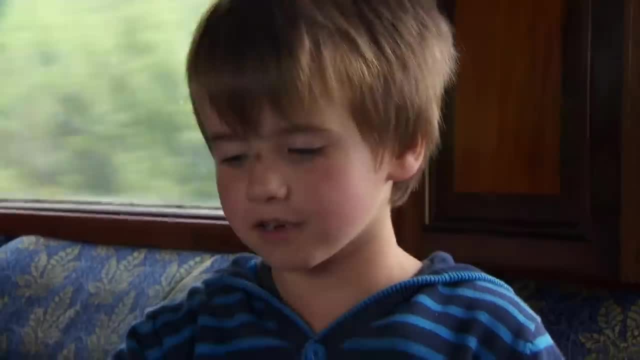 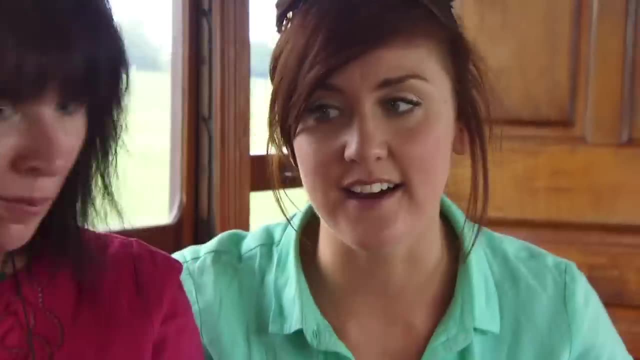 train before and we've got all our food to share with everybody. Mum, would you like to try some of our food? Of course, yes, please, George, Look at this. it's delicious, Mmm. I like it Delicious. Shall you make your mum do the fruity dance? 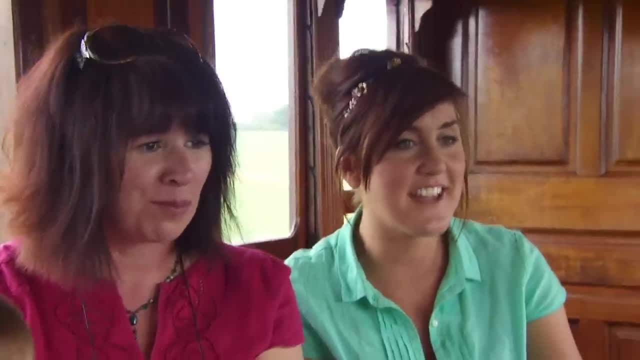 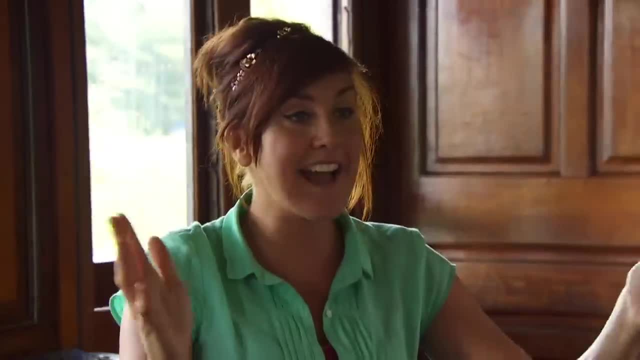 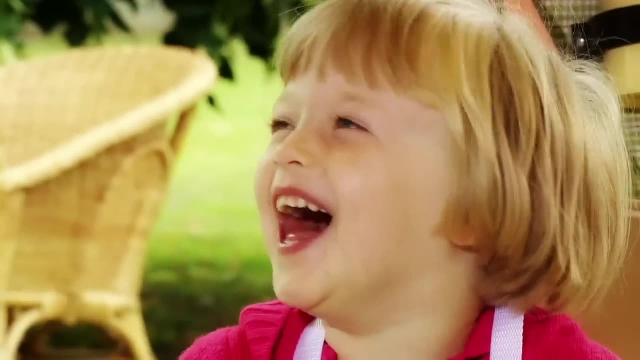 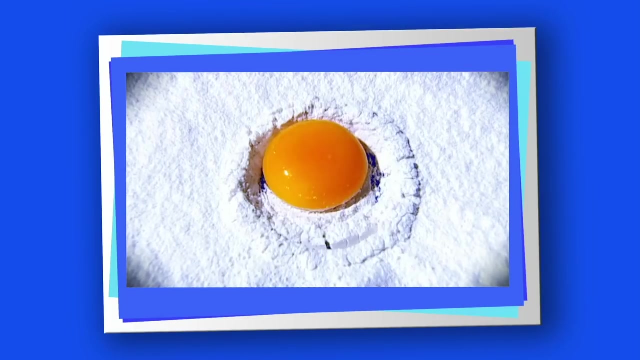 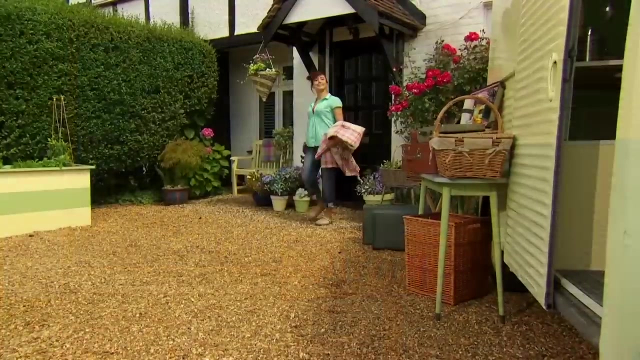 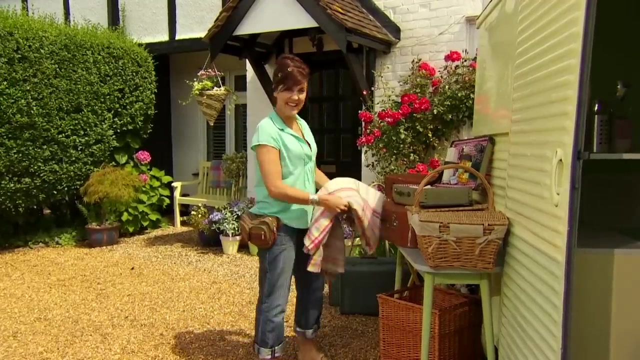 So, everyone, what can you do? I can cook With you, Oh great. I've been waiting for you. I've got everything ready to go on a journey and I hope you're going to enjoy it. Come with me and meet some new friends. 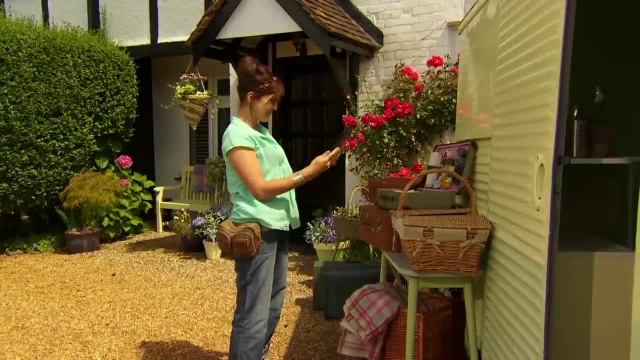 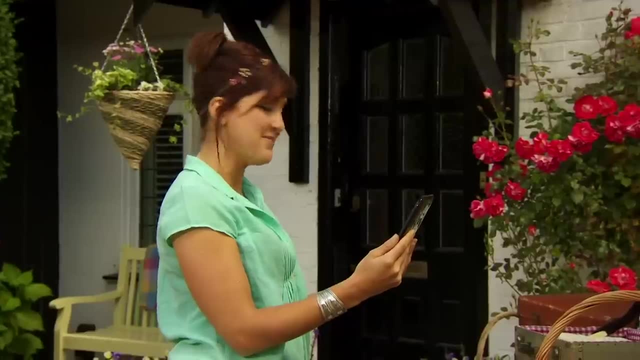 Aha, Hello, Katie, I love doing that stuff and I really like courgettes. Katie, can you cook with me please? I can and you can cook with me too. I've got the perfect recipe to cook with courgettes. 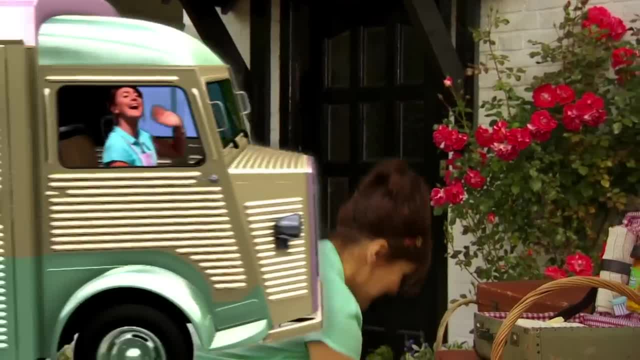 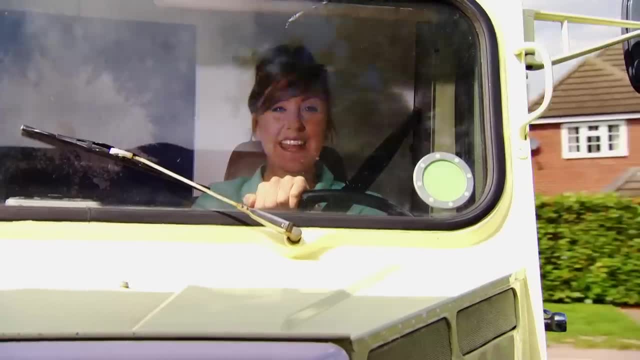 So let's pack everything up and get going Off on a journey- and I'm coming to you. We're going to be busy and there's lots to do. Get ready to help, join in and have fun. Let's cook a feast for everyone. 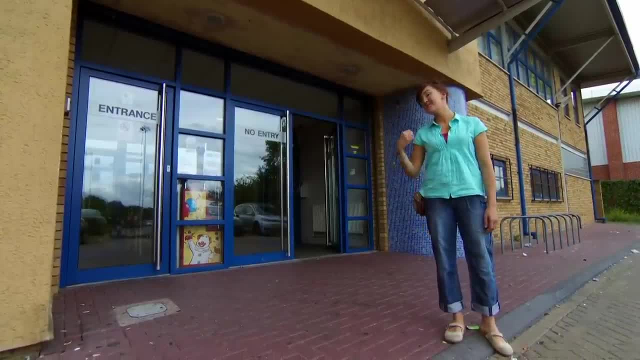 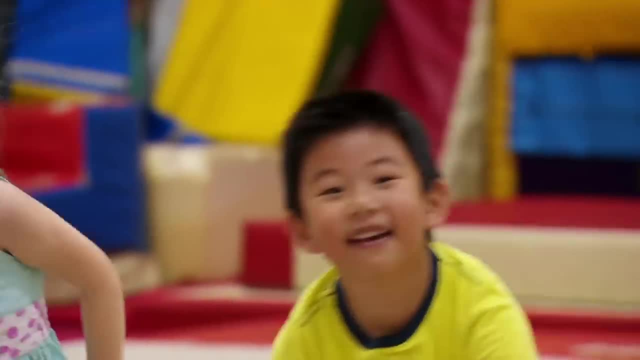 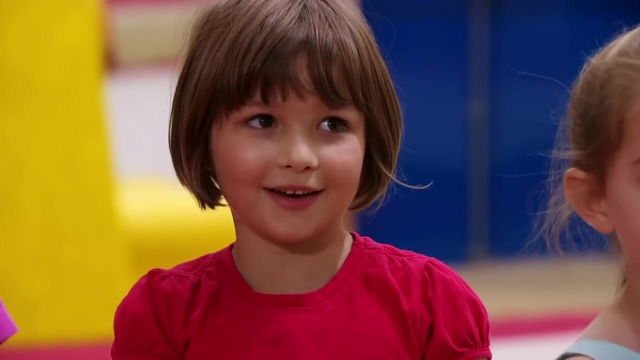 Well, here I am at the gymnastics hall where I've been invited by Wilson, So let's go and find him. Hi Wilson, Hi Katie Wilson, are these all of your friends? Yes, What's your name? Jessica Caitlin. 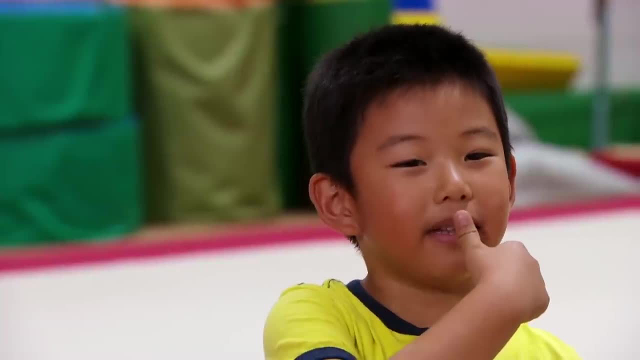 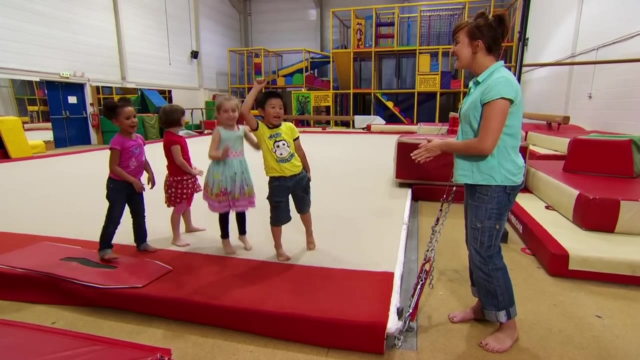 Hegan. So Wilson, what are we going to do today? Make something with courgettes, Courgettes. I have such a good recipe with courgettes in it. Do you all want to cook it with me? Yeah, Well, come on then let's go and do some cooking. 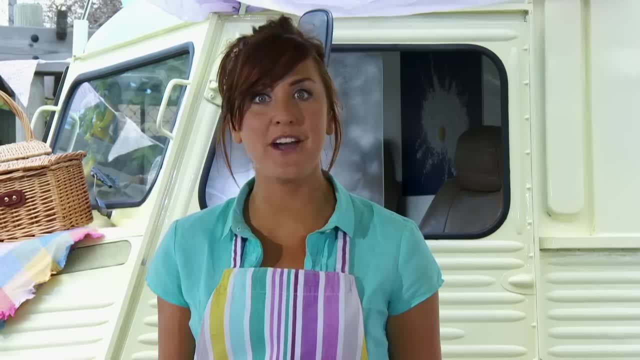 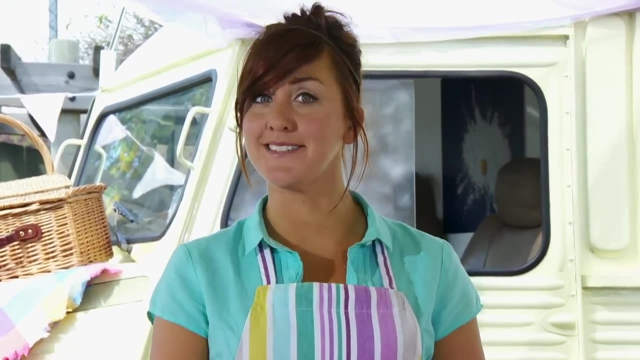 Welcome to my outdoor kitchen team. Who wants to know what we're going to cook today? Me, Okay, I'll tell you. Today's recipe is the delicious green parcel pie. Oooh, Look at that Now before we start cooking. 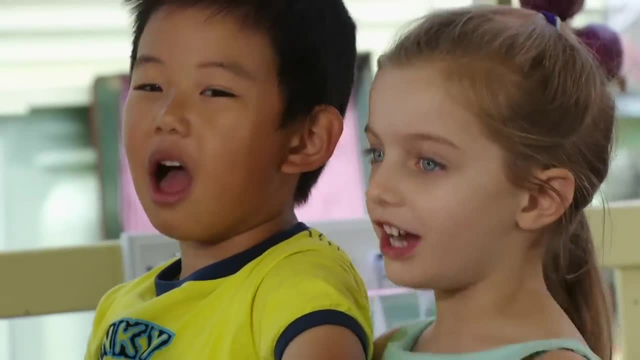 we've got to do something first. What do you think it is? Wash our hands. You've got it, team, We're going to wash our hands. Let's go Roll up your sleeves. Give your hands a wash With slippy dippy soap. 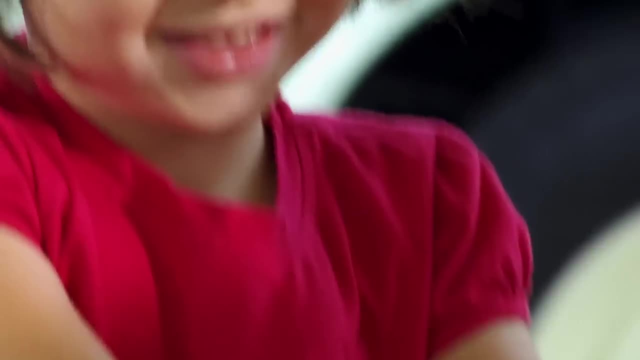 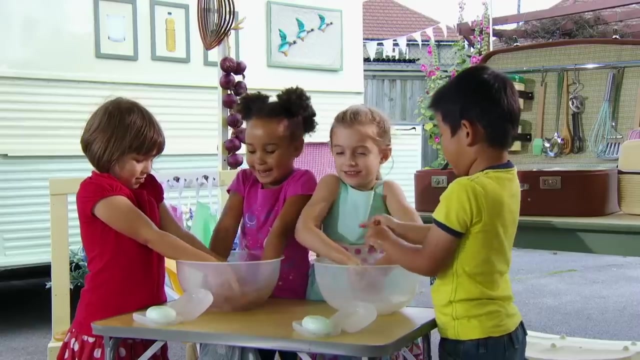 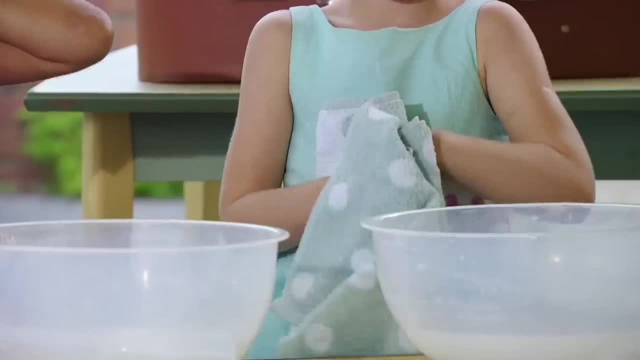 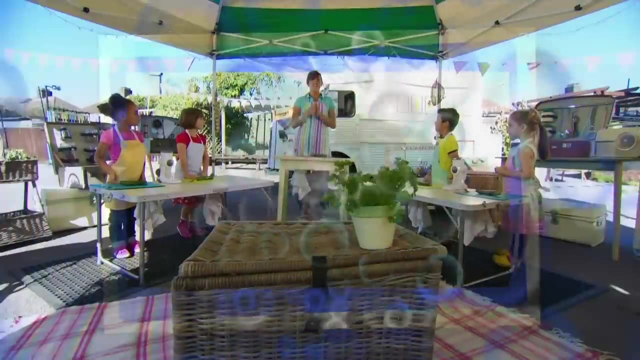 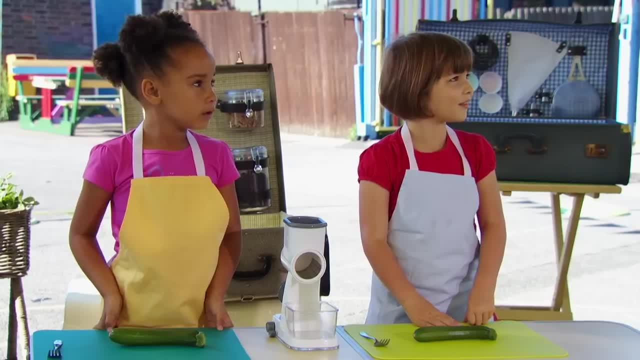 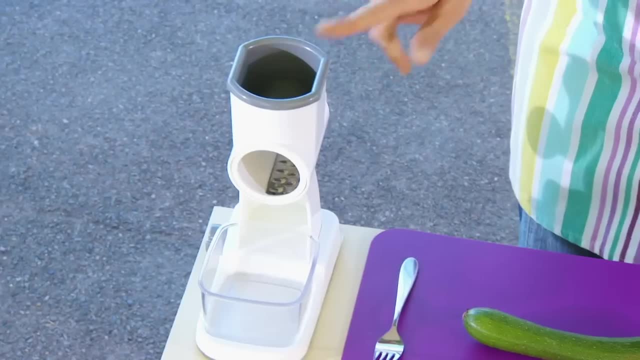 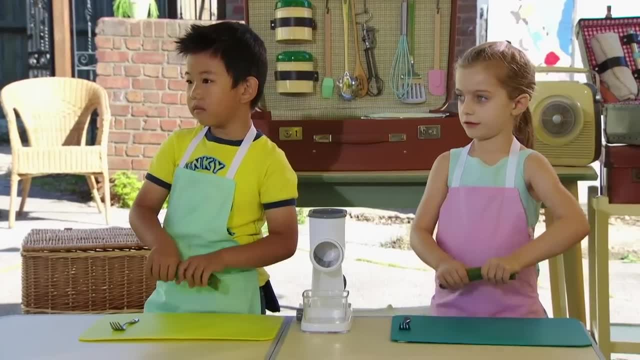 to make our green parcel pie is some grating And we're going to grate this. It's a courgette and we're going to grate it using a grater, That's it. But the first thing we have to do is snap the courgette in half. 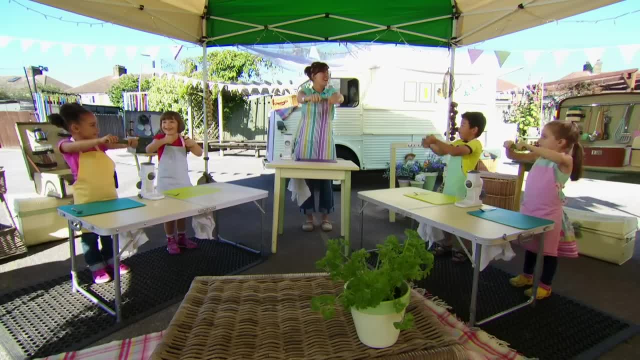 like this: We hold it out in front of us and then after three, we're all going to snap it like a big snapping crocodile. Oh, look at that. Look, it looks like a crocodile's mouth. Snap, snap, snap. 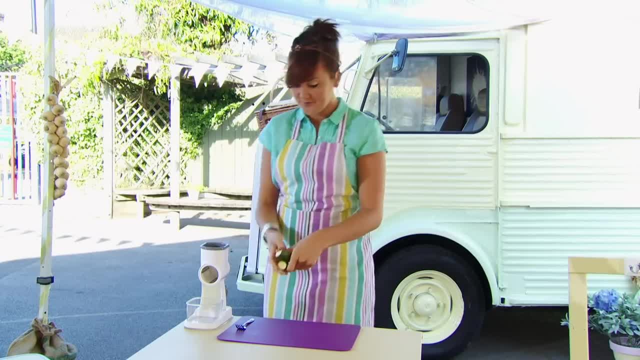 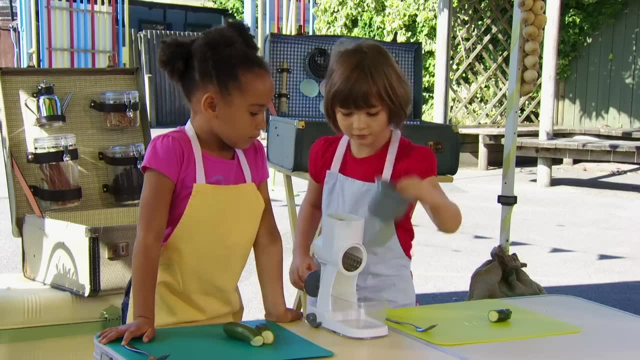 Now we need to put these pieces of courgette into the grater, So we put it in the top part like that, And then we put the lid on top of the grater And then push down on the top and turn the handle. 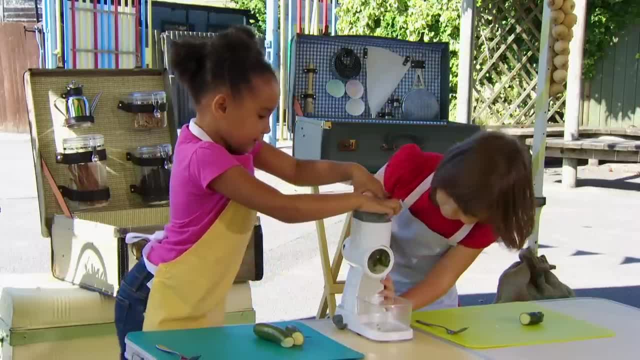 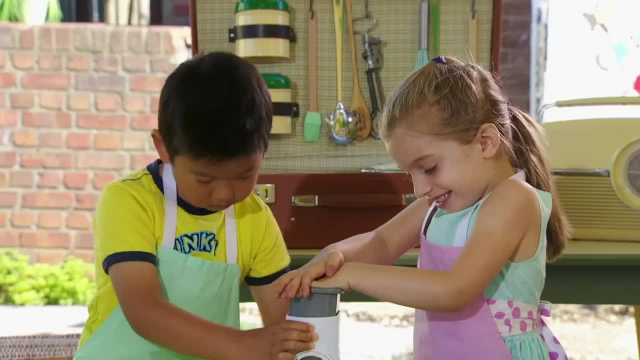 So push down really hard Tegan on top, Make sure that Wilson can move it. That's it, Good question, He's a top grater. And next use your fork and scrape out some of the bits in the middle. 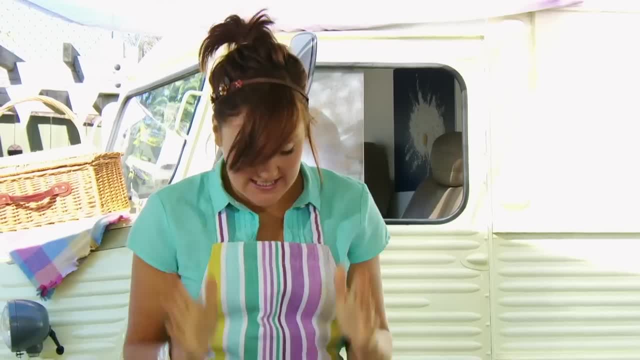 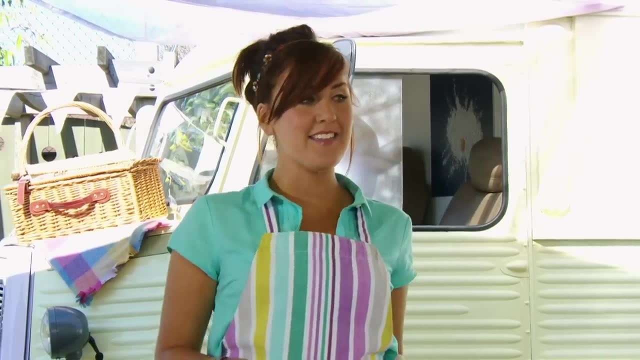 That was great, grating everyone. Next, we're going to need this. This is an egg which I've already cracked for you in a bowl, And does anybody know where an egg like this might come from? Chicken, That's right. 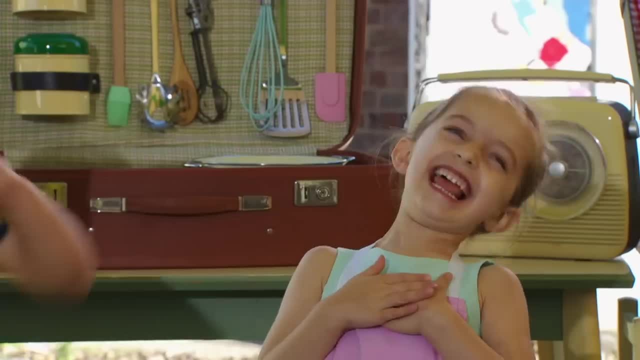 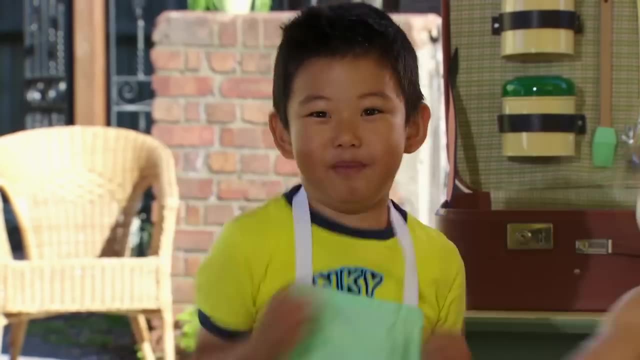 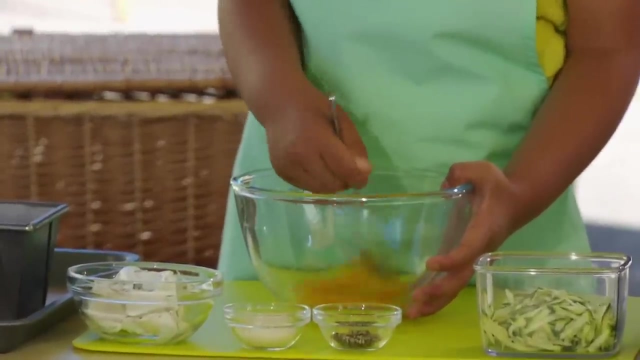 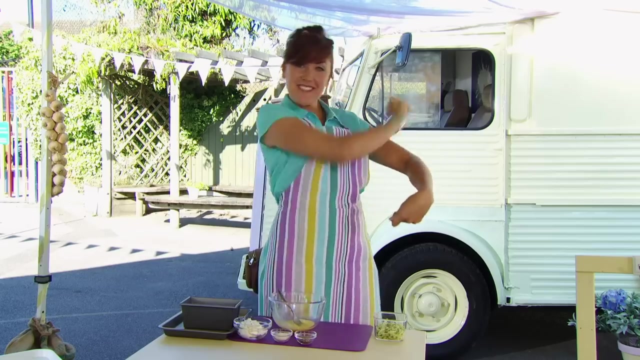 It's a chicken Who can pretend to be a chicken. Right, let's get whisking, then, team. Why don't you do some whisking at home as well? You can get your bowl and then get your fork, and then whisk, whisk, whisk. 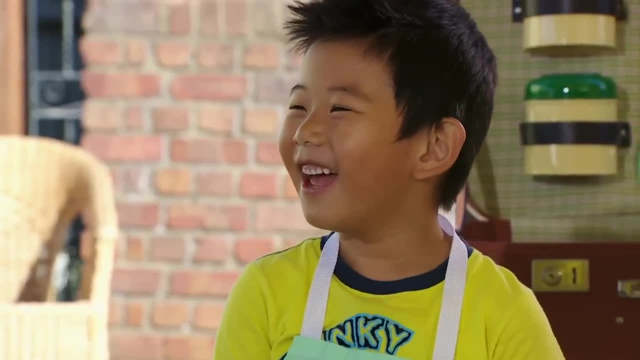 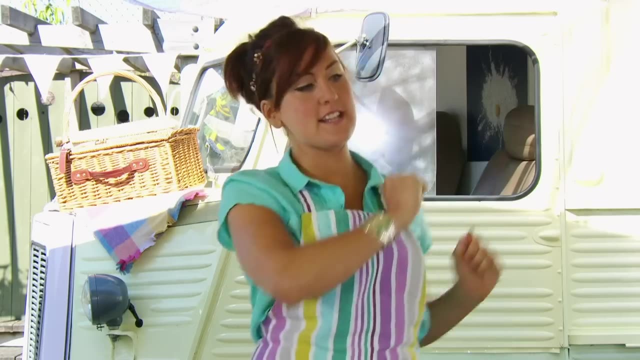 Wilson, what's happened to your egg? It's turned yellow. OK, the next ingredient is this: This is a delicious soft cheese and it's got a secret ingredient in it. Does anybody know? Do you know, what these little green bits are inside it? 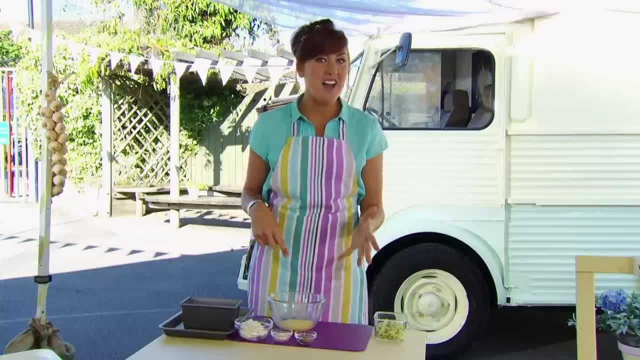 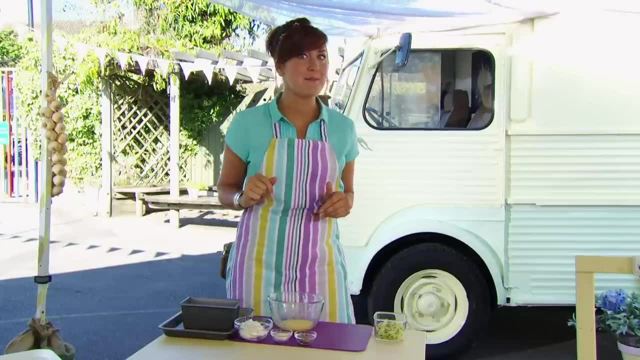 No, They're chives which come from the same family as onions. They've got a really strong taste. So this cheese is cheese and onion flavour which is going to be delicious in our green parcel pie. So let's take our soft cheese and our fork and scoop it into our egg. 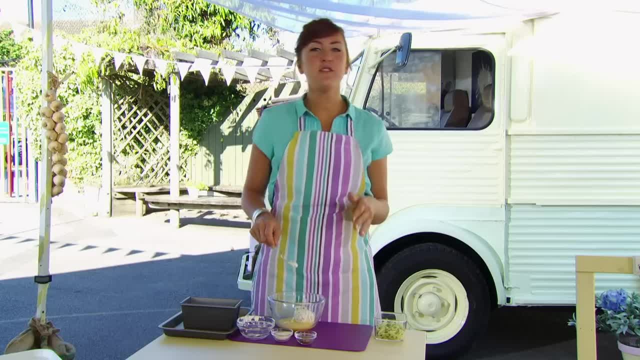 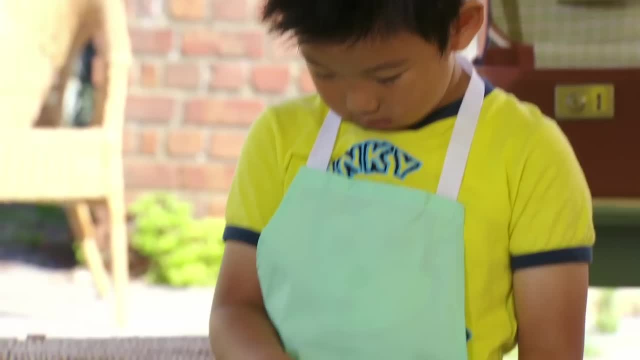 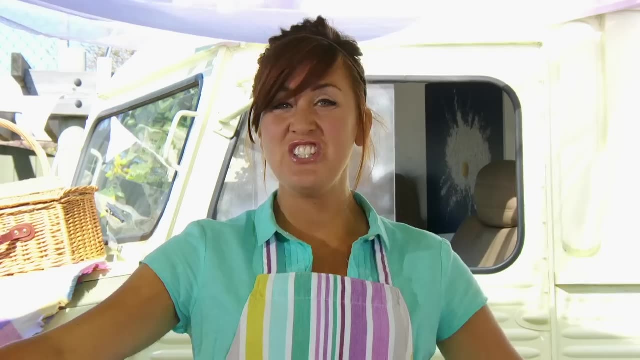 Ready Scoop, And then we're going to use our fork to mix it all up. Let's go team. And then, when you've mixed everything up, we're going to add another cheese. Who can go? The next cheese we're going to add is an Italian hard cheese. 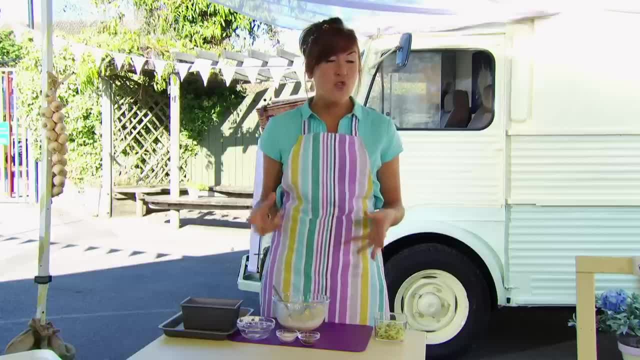 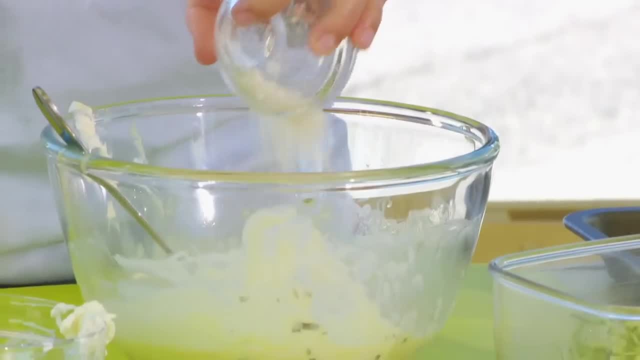 which you might have had with pasta at home, And it's got a really strong taste and it's got a really strong smell too. So let's sprinkle it in: Sprinkle, sprinkle, sprinkle. Next we're going to take a pinch of pepper. 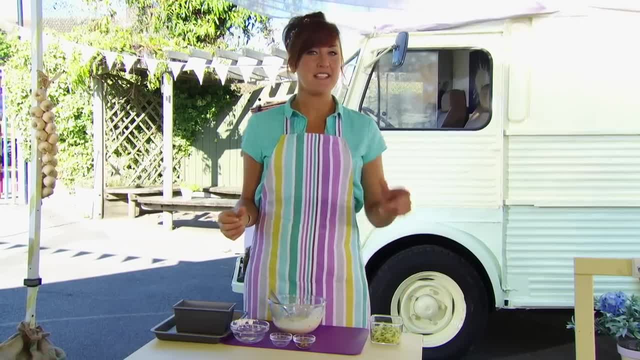 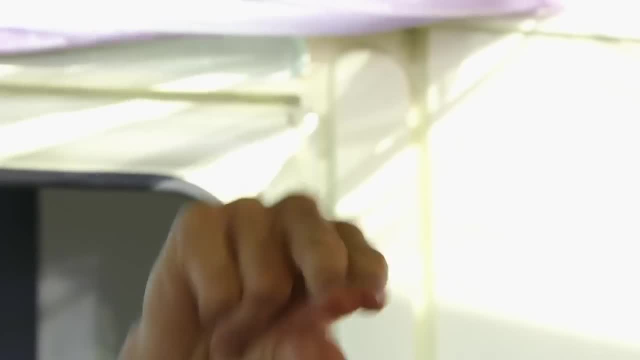 and we're going to need the help of our pinchy parrot to do that. And to make a pinchy parrot, you put your thumb down and your fingers on top and do a big squawk. My parrot's so hungry. 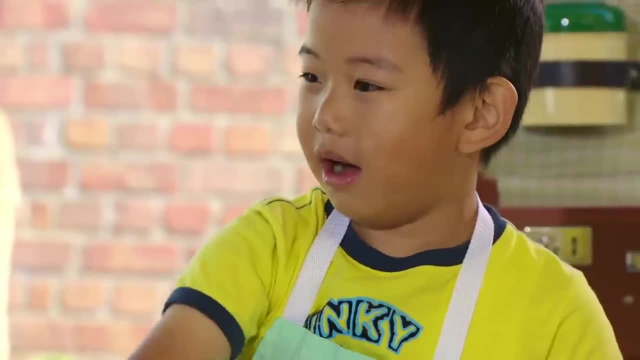 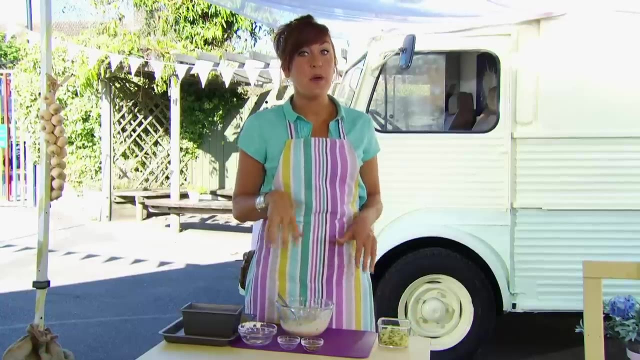 Yeah, and the parrots are hungry, so they need to take a pinch of black pepper And then sprinkle it into your bowl. And next we're going to add the grated courgette into the lovely eggy cheesy mixture And then give everything. 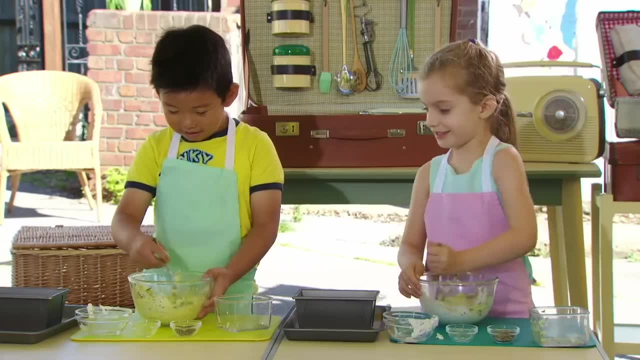 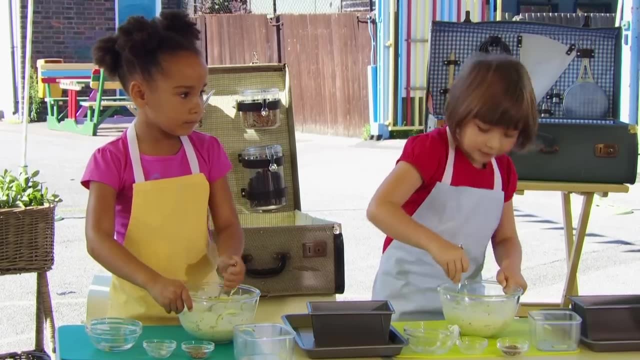 Make sure you get all the courgette mixed in with the eggy and cheesy mixture- Eggy cheese- And put your fork down, everybody. Now we need to grease our loaf tins, And I wonder what we're going to need to do that. 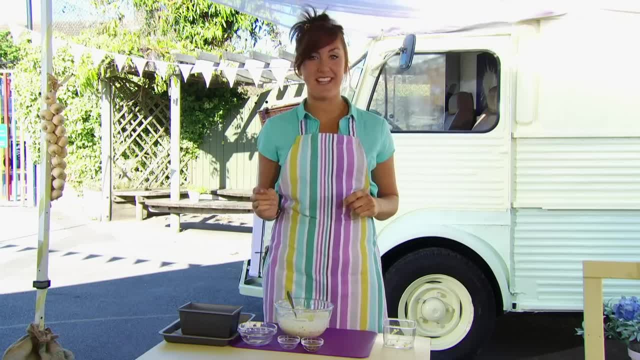 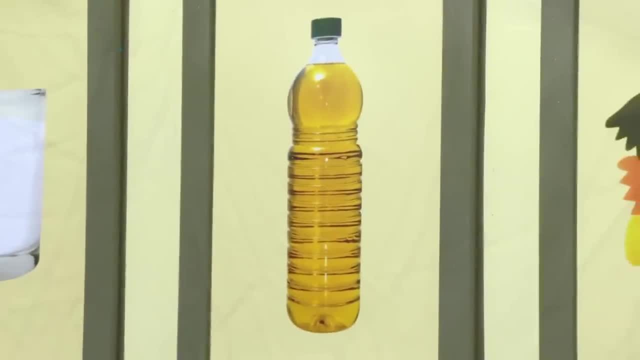 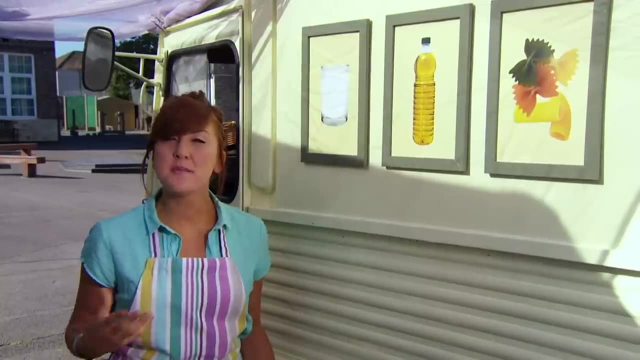 What is next? Well, let us see if you can guess what it could be. So we've got some milk, some rapeseed oil and some pasta. What would you choose for our green parcel pie? I know I'll give you some clues. 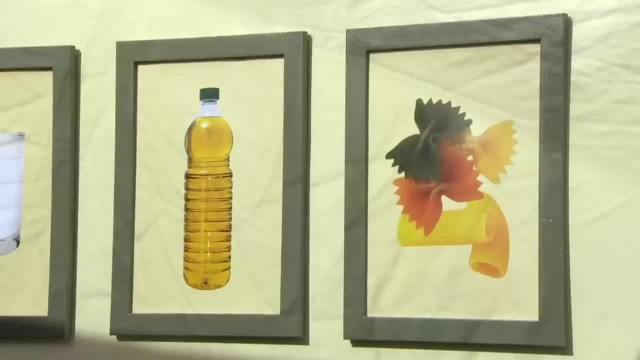 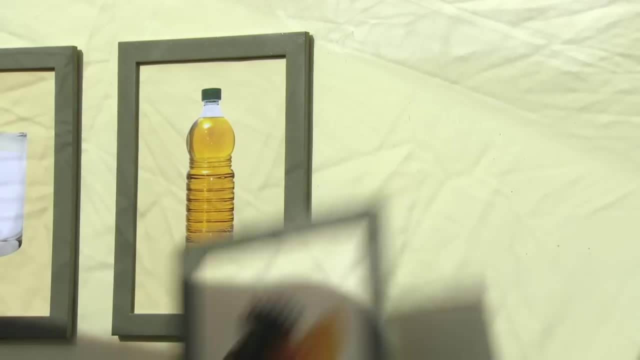 and then you can try and guess what it might be. The special ingredient is a liquid. Well, pasta is a solid, isn't it? So we can take that away. There we go. OK, here's another clue. The special ingredient is a liquid. 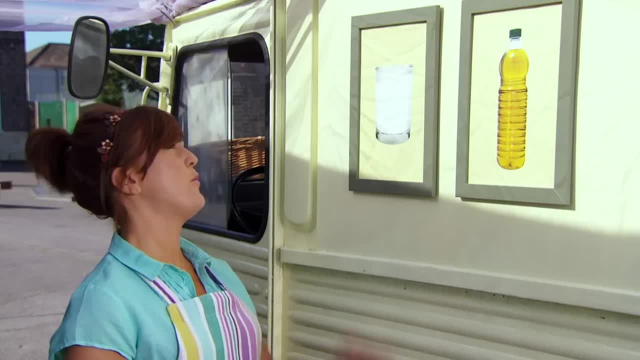 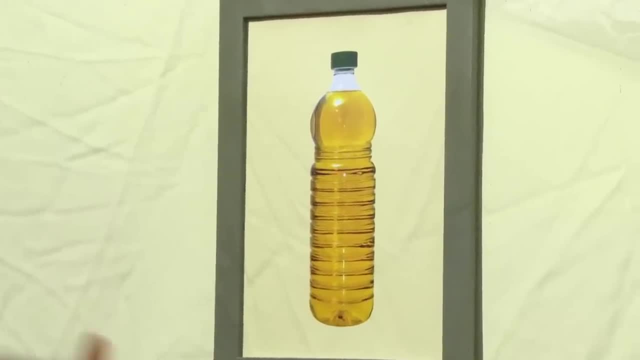 and it comes from plants. Well, milk comes from cows, doesn't it? So we can definitely take that one away as well, Which leaves us with rapeseed oil. We're going to need some of this in our green parcel pie. 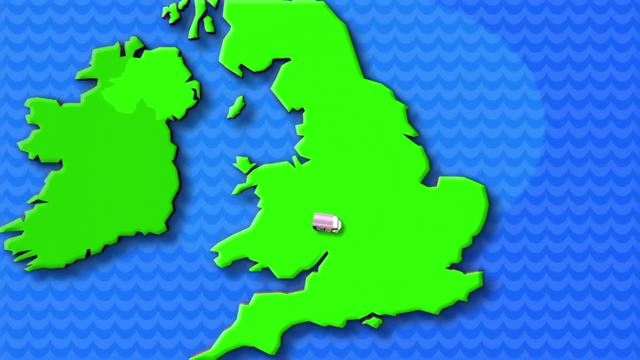 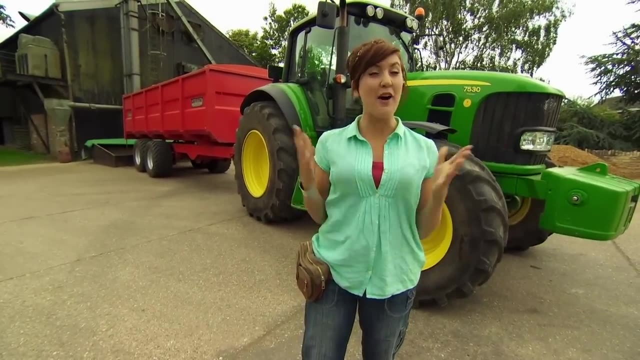 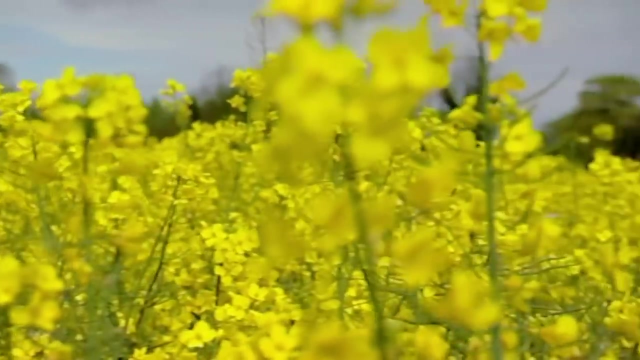 And I drove to find some. I've come to a farm in Hargrave in Northamptonshire to find out how rapeseed oil is made: When the plants bloom, the flowers are bright yellow And when the sun cooks them. 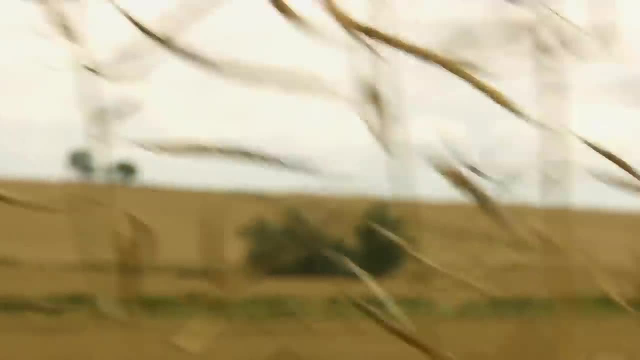 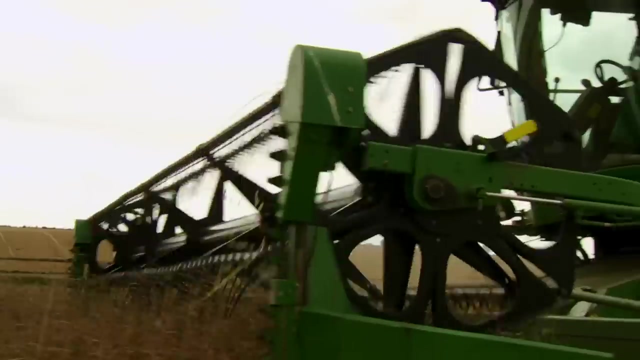 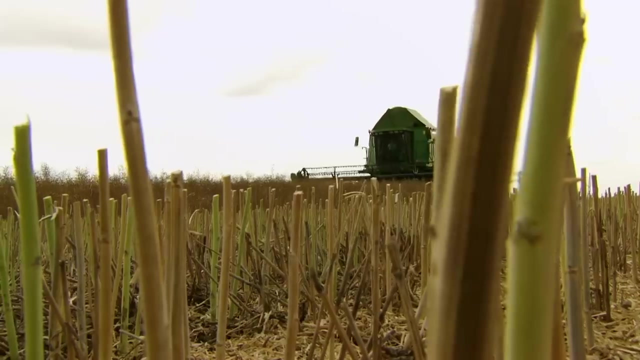 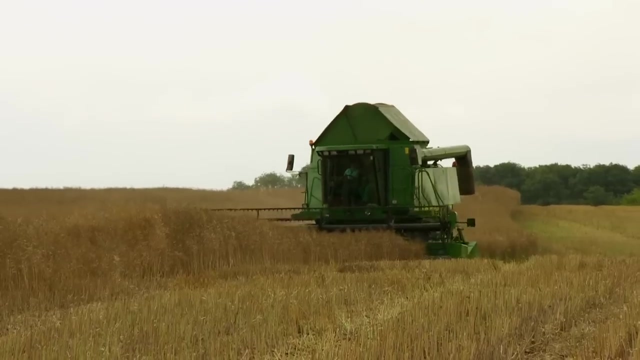 they turn into this lovely golden colour. The rapeseed plants that look like this are cut down by a big machine called a combine harvester, And there it is now. Look Right, I think I'm going to have a go. There we go, look. 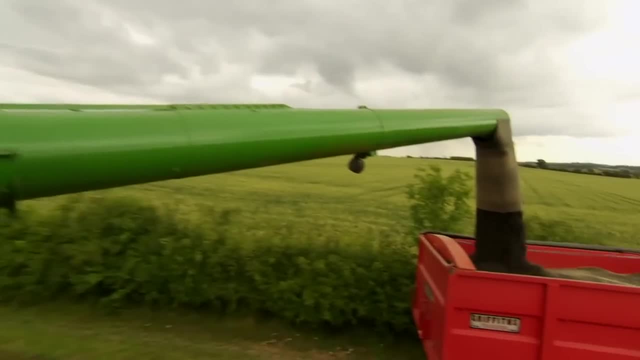 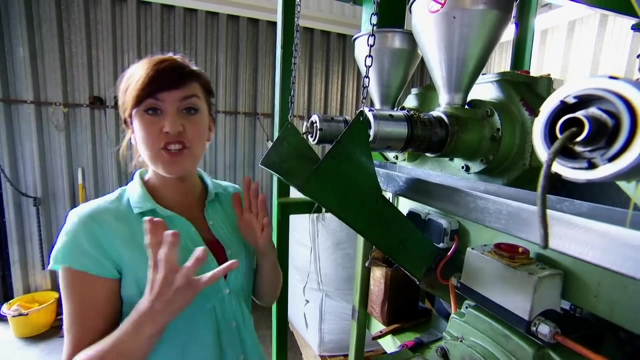 This machine collects all these little black seeds, and that's where the rapeseed oil comes from. The rapeseeds are brought back to the factory and they're put in this big machine which gently squeezes them until the oil comes out. Look, 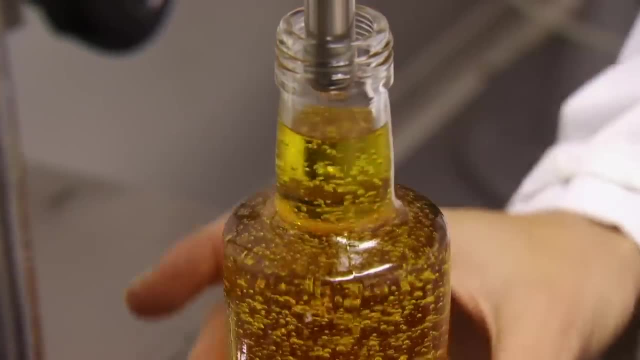 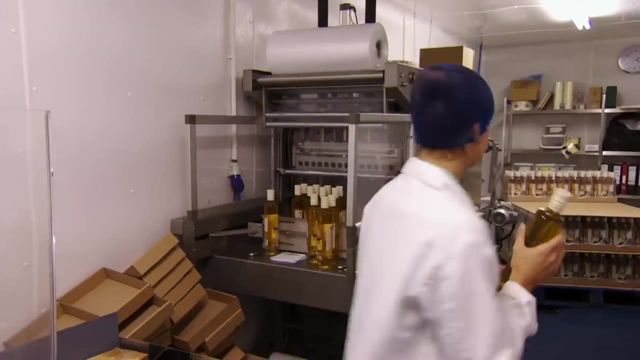 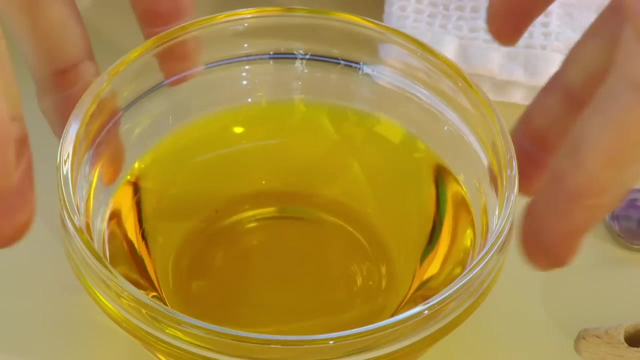 Once the oil has been filtered, it just needs to be poured into bottles- Fantastic. I can't wait to use this in our green parcel pie. Finding out how rapeseed oil is made is fascinating, And look, we've got it here. 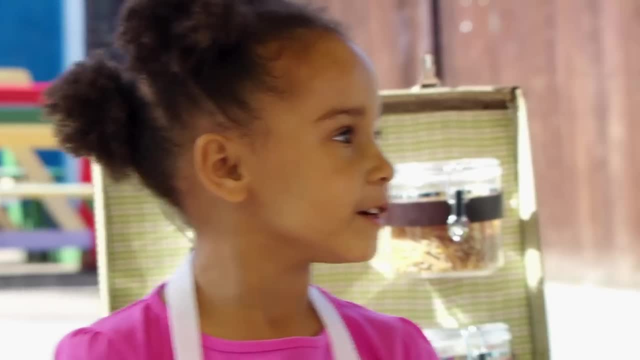 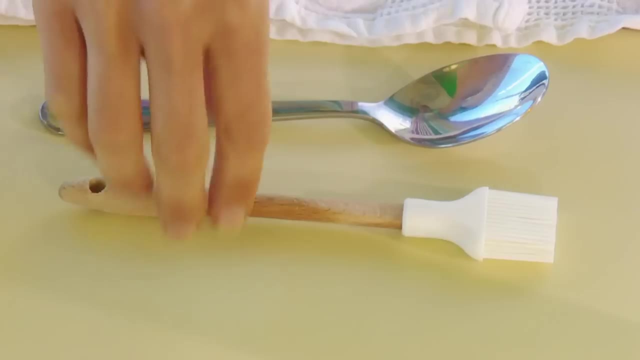 What does the colour remind you of? Shiny gold, Shiny gold, Yes, shiny gold. Now we're going to use this rapeseed oil to grease our loaf tin, And for that we're going to need our brush. So why don't we practise doing some brushing? 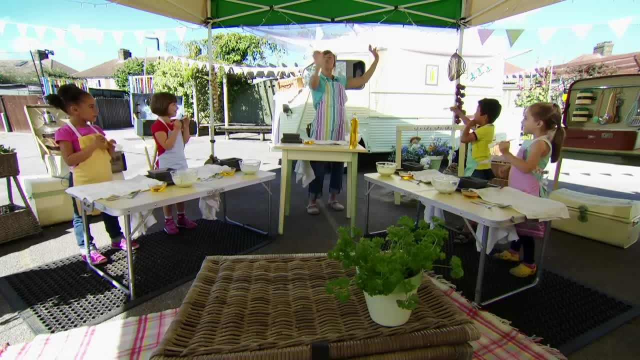 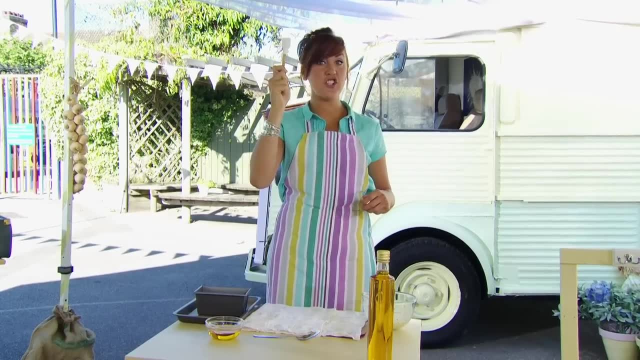 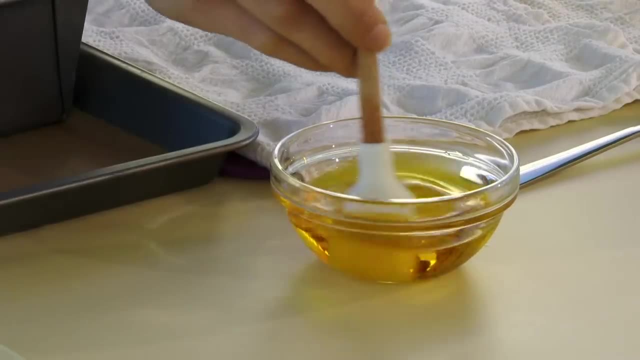 like we're painting a picture, like an artist. So everyone go brush, brush, brush. Can you do some brushing with us? Get your brush and go brush, brush, brush. Now dip the brush into the oil, Look at that And then brush it all over your loaf tin. 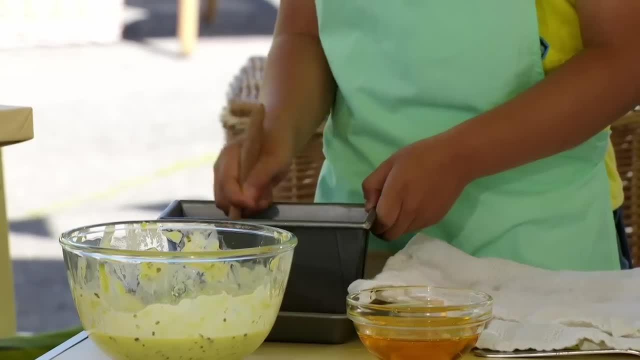 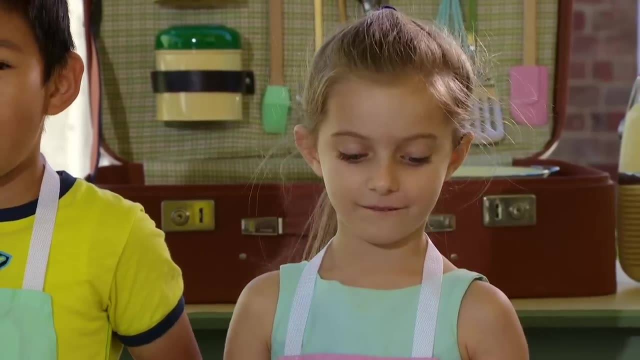 We have to grease our loaf tins so that our green parcel pie won't stick to the edges when it goes in the oven. And next we need to make the pie, And for that we're going to use pastry, And the type of pastry we're using is phyllo pastry. 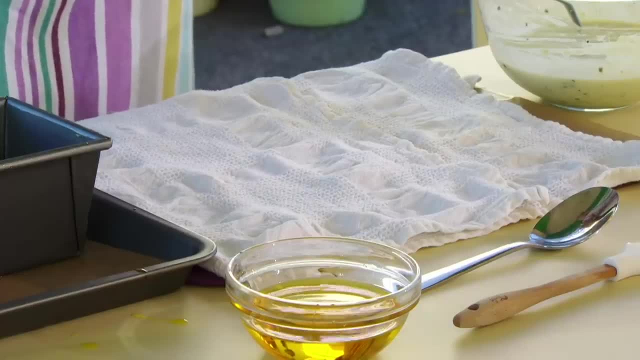 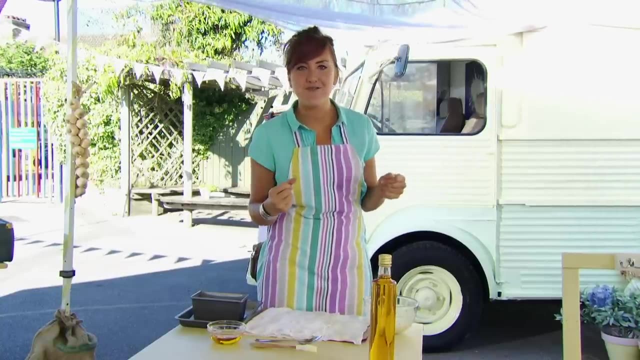 And I've covered the phyllo pastry in a damp towel so that it doesn't dry out. But when the phyllo pastry goes in the oven later on it's going to go so lovely and crispy. So let's take the damp towel away. 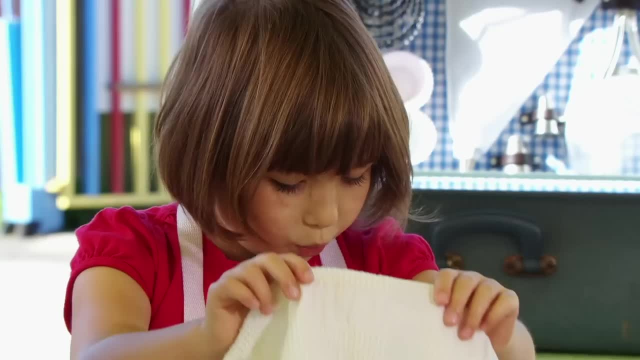 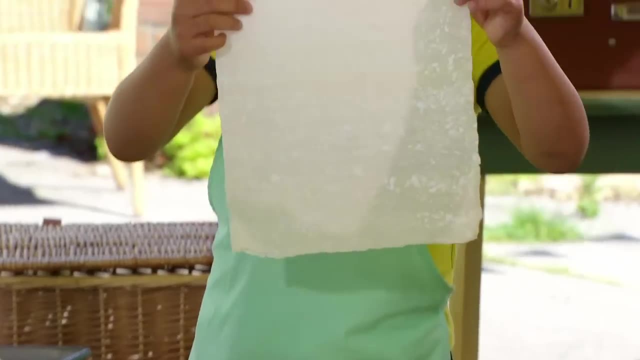 Can you see it underneath? Yeah, It's so white and fluffy And we're going to peel off one layer of phyllo pastry And we're going to hold it like this: Gently drop it into your loaf tin. That's it. 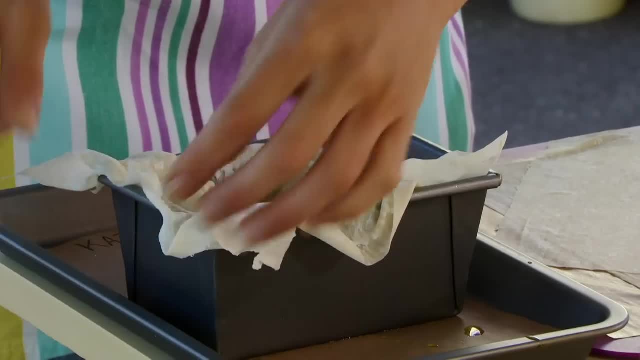 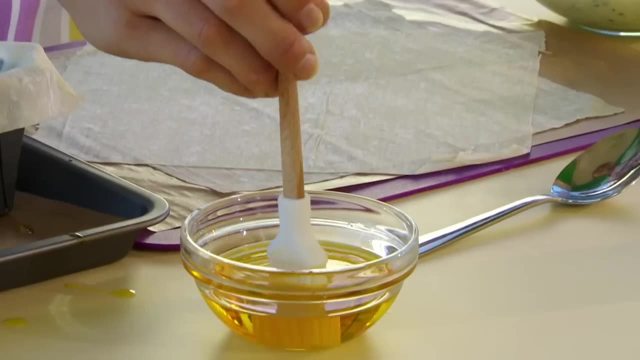 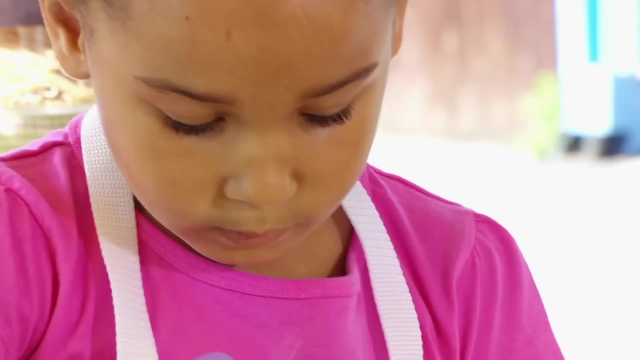 And make sure all the edges lie on the outside of the loaf tin like that. There we go And then use our brush, dip it into the rapeseed oil and dab it all over your pastry in the tin like golden raindrops. 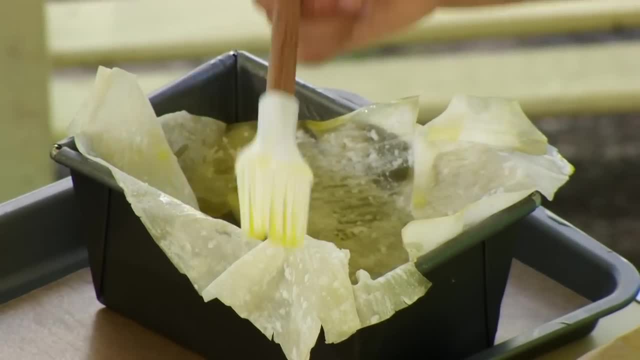 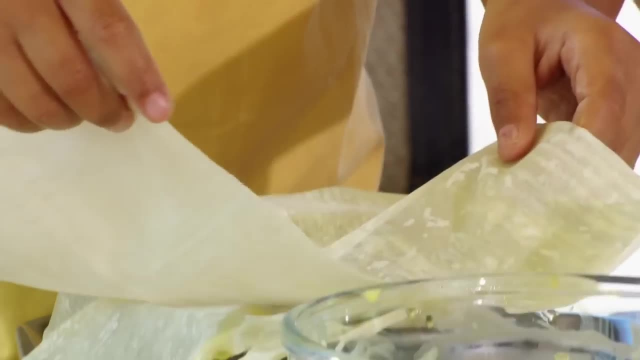 And remember to get it right round the edges, because they're the bits that are going to go extra crispy when it goes in the oven. And next we're going to add another layer of phyllo pastry, like you're making your little bed, Okay, and then we need to dip and dab again. 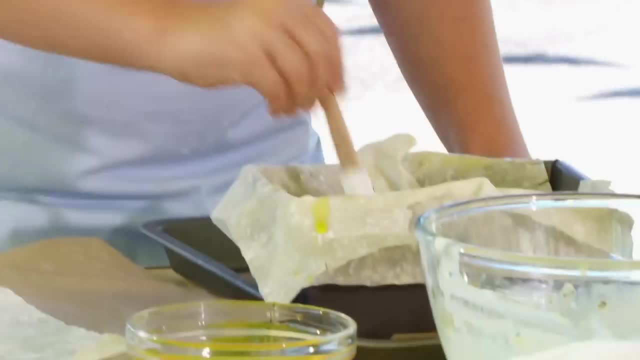 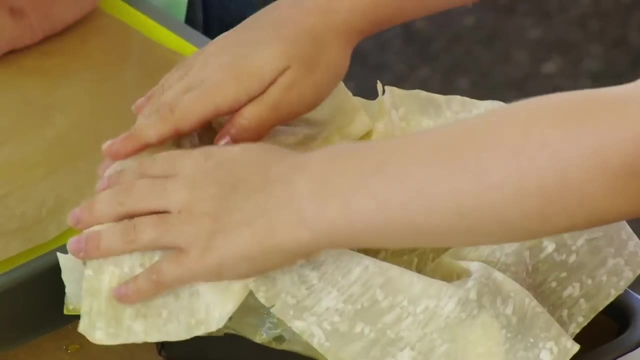 And then we need to put the very last bit in quickly, before it dries out, And we don't need to put any oil on this bit- And the next thing we need to do is scoop the eggy cheesy mixture into the pastry bed. 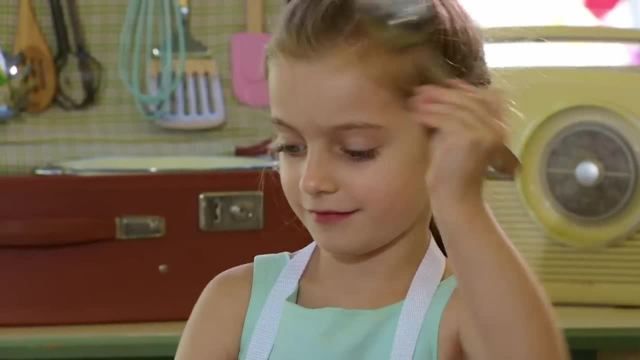 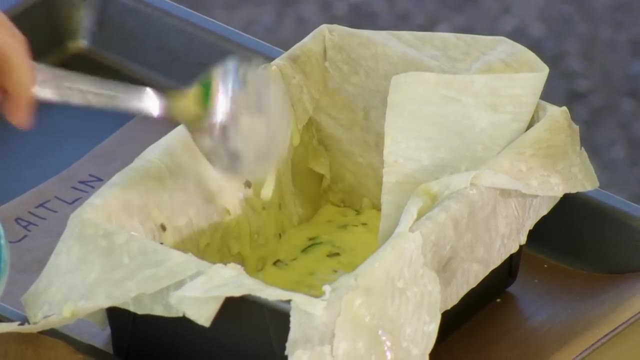 So get the spoon. Have we got a spoon? Yes, Okay, and take your bowl and scoop the mixture up and splosh it into its bed. Scoop and splosh, Splosh, sploshy And keep scooping. 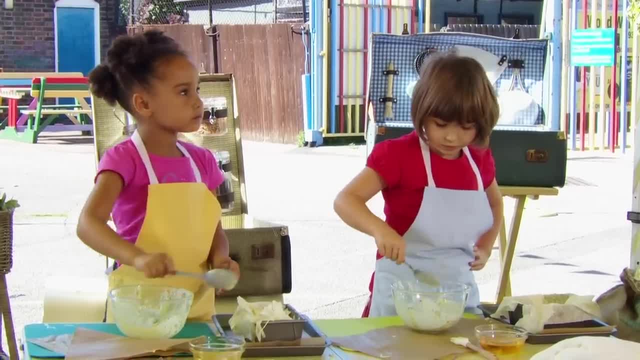 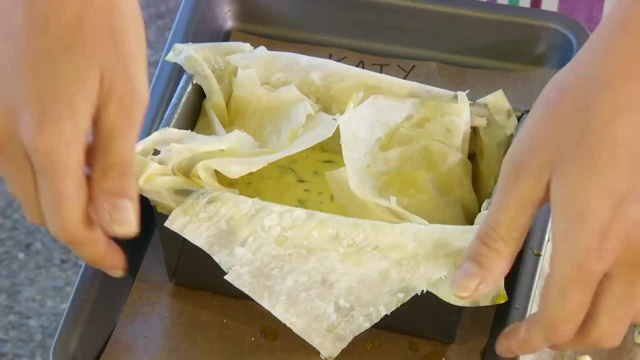 until all your mixture is in the phyllo pastry bed. And then, last but not least, we have to tuck the mixture in. So, very gently, take all the phyllo pastry from around the side and fold it over the top. Make it all spiky. 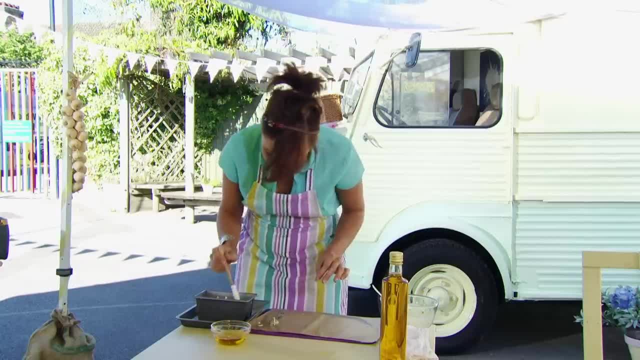 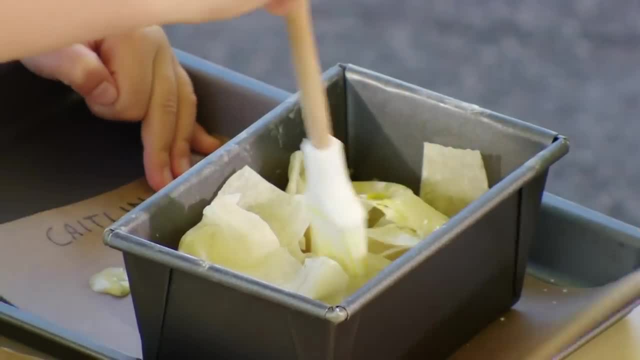 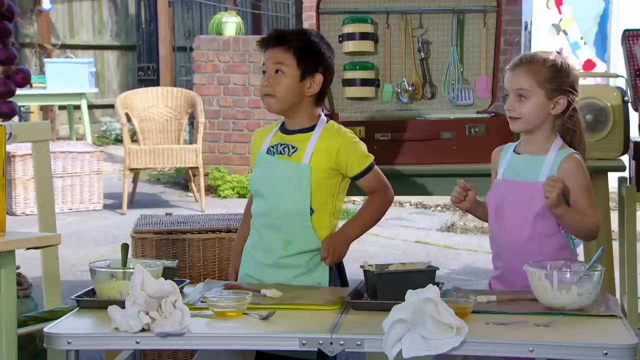 We just need to dab one last bit of oil on top to make it extra crispy and shiny, Just for some extra shine. Shine, shine, shine And that is it. You've done it, everybody. You've put all these ingredients together. 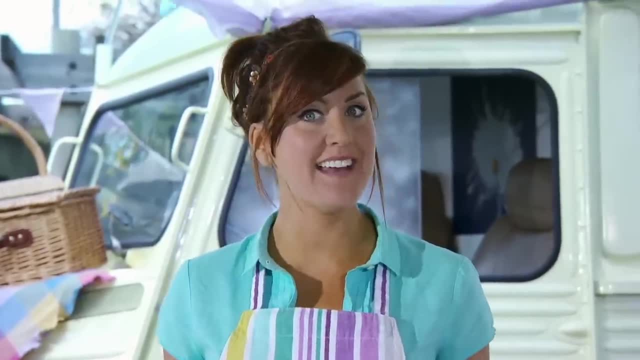 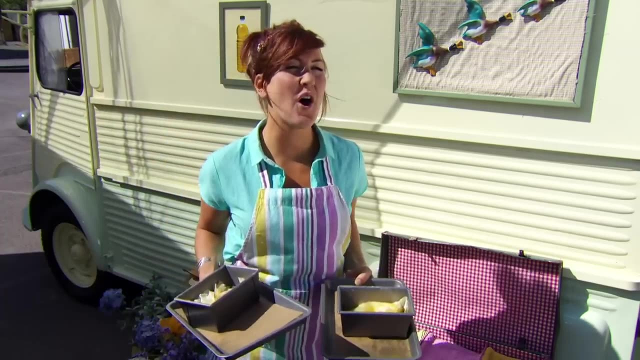 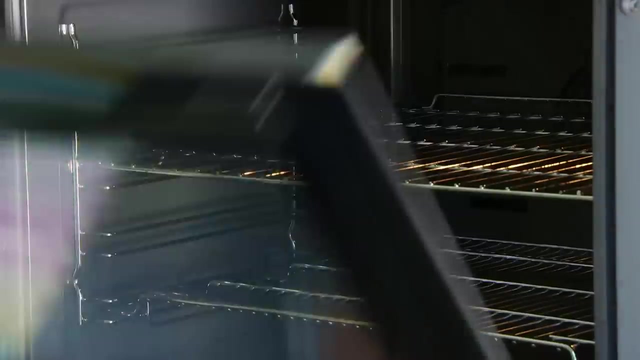 for your green parcel pie all by yourself. And now it's time to put them in the oven to cook. But remember ovens are hot, so don't go near. Ask a grown-up to help you here. Now we've cooked with you. 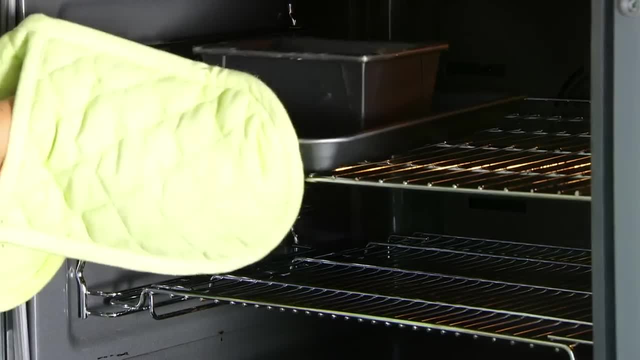 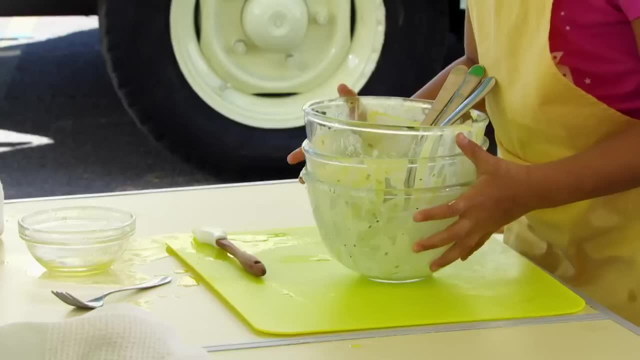 and had lots of fun. Let's tidy up and think of all the things that we have And when we have done. there was grating, whisking, mixing, brushing, clearing any mess and putting things away is always fun to do. 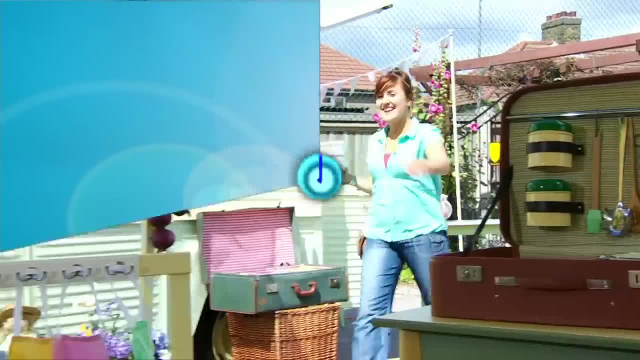 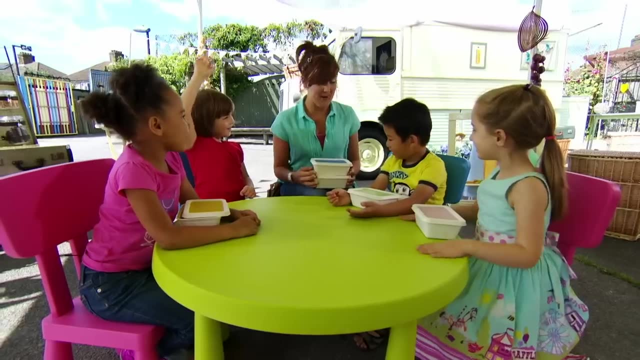 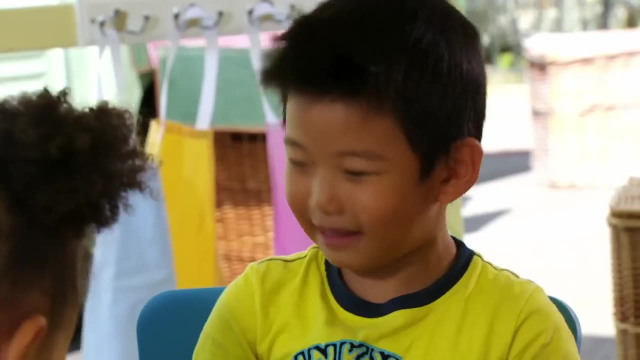 at the end of the day. And here they are, all cooked and ready to eat. Who's excited Me? Oh, I'm so excited. Okay, let's have a look at yours, Wilson. What's changed with yours? It's a different colour. 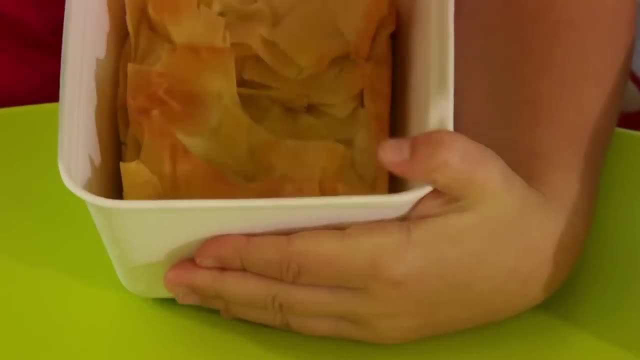 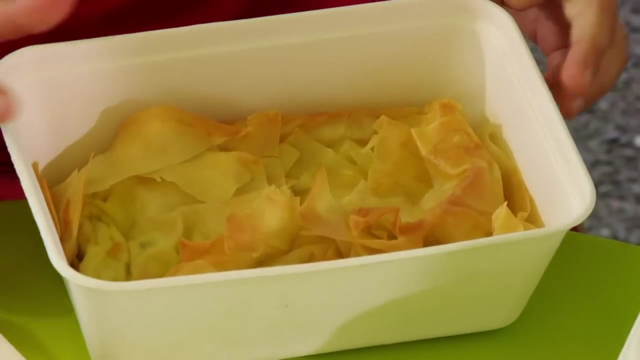 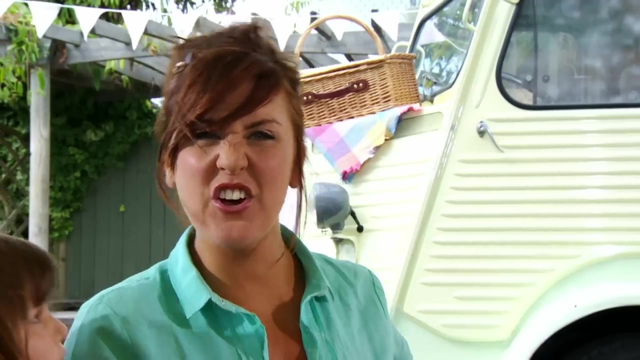 Okay, Caitlin, ready to look at yours? Let's see What does it look like? It looks hard and crispy. Okay, team, let's put the lids on top, and then we can save this for later on. We've travelled to you. 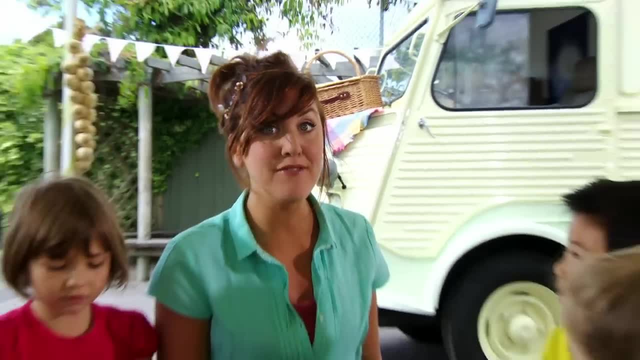 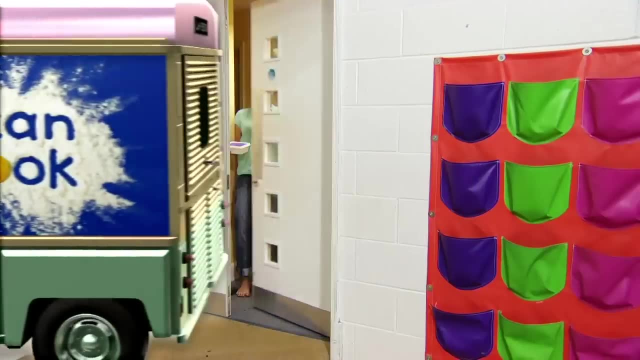 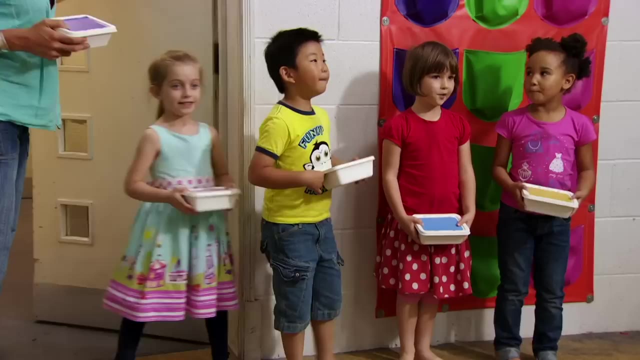 we've cooked and had fun. Now let's have a party with everyone. Yeah, And you can come with us? Come on. Well, here we are at the gymnastics hall and we've got our food to share with everybody Who's hungry.